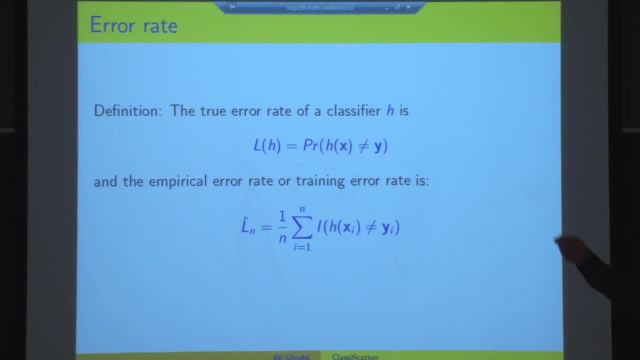 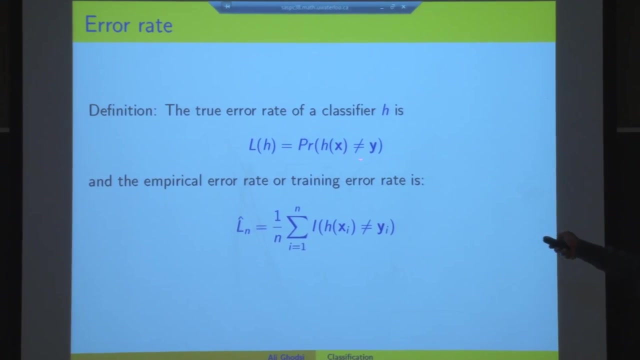 So the chance that my function predicts a table when it's a chair, This probability is called true error rate. Pay attention to this X here It's a random number, It's a random variable and this Y is a random variable. so we are talking about probability. 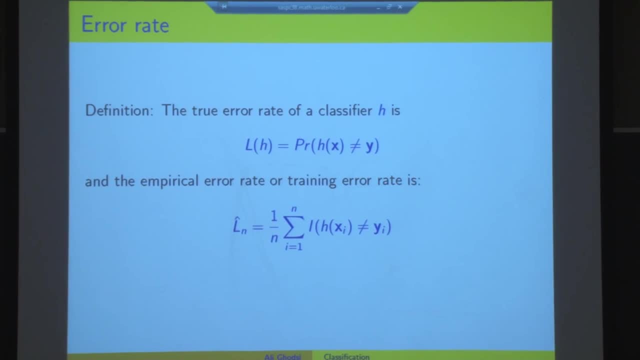 of this random variable not being correct, So we can't usually compute this probability because what we have is only a sample of our random variable. You have a random variable X, but you have N samples of this random variable. And you have a random variable Y, but you have N samples of this random variable. 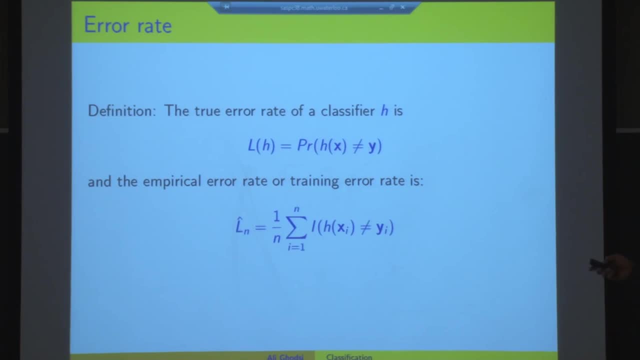 So we can't compute this probability, but we can estimate it. How can we estimate it? We can estimate it this way: This I here is just an indicator function. So if H, if H is equal to, is not equal to Y, then I of this bracket is 1.. 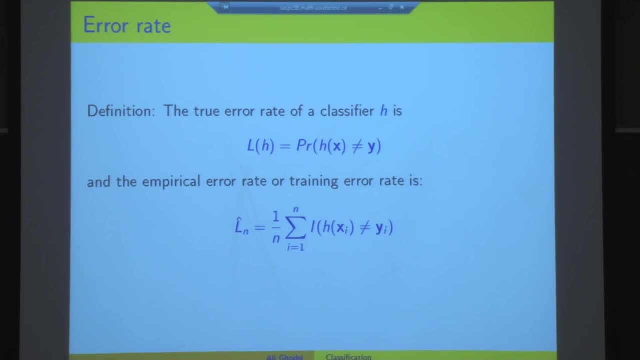 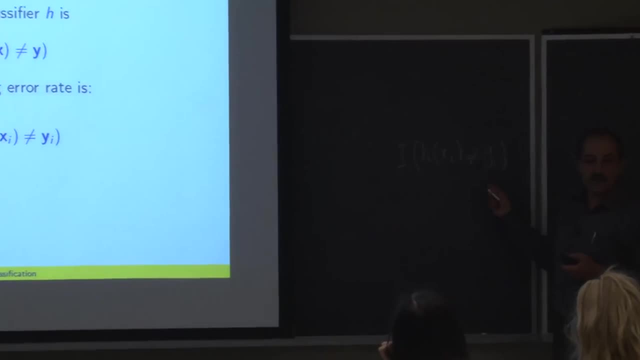 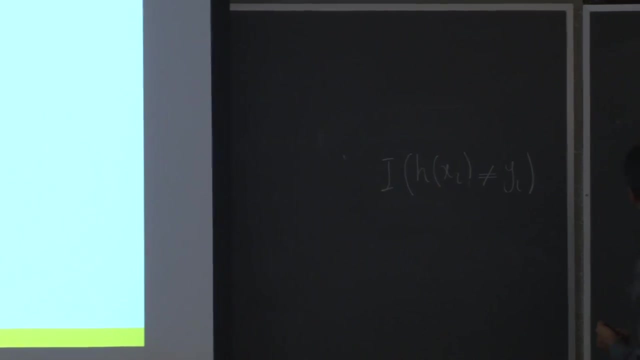 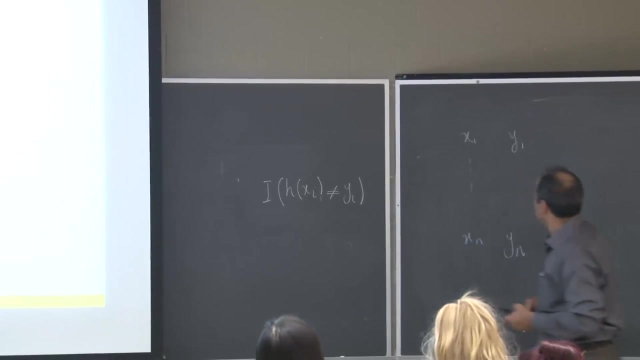 If these two are not equal, it's going to be 1.. Otherwise, it's going to be 0.. So, basically, this summation simply means that when you have N data points and you have N labels, you compute H. Okay, Okay. 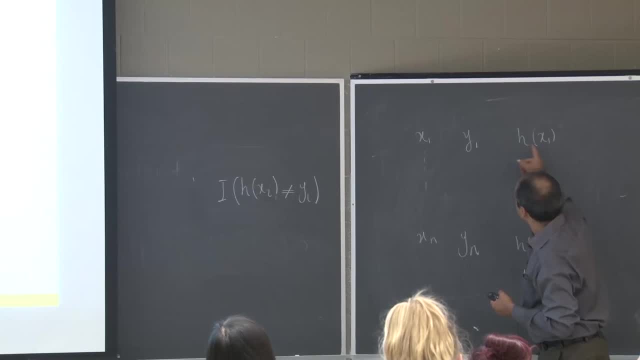 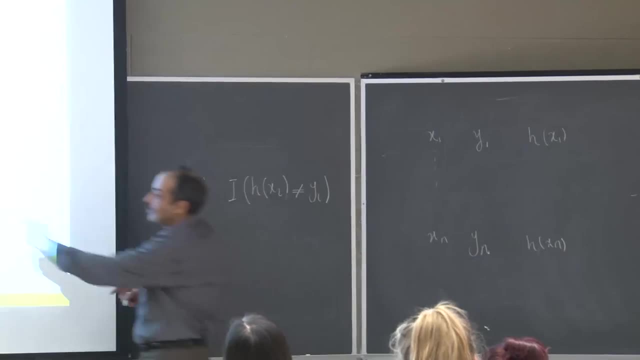 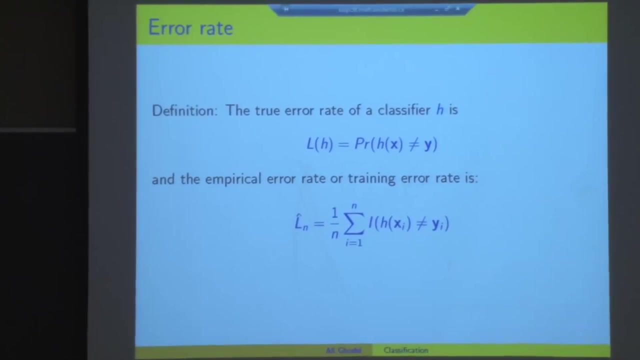 Really fast and you count the number that HX1 is not equal to true Y. So you count this number through this sum and then divide it by the total number. So if among 100 points 10 of them are not correct, 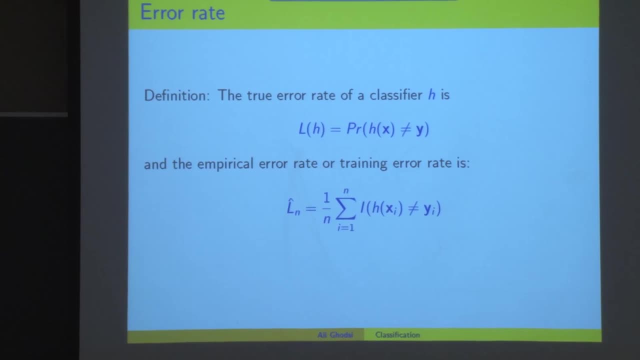 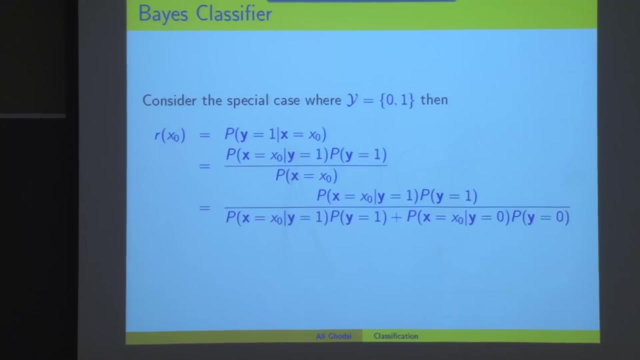 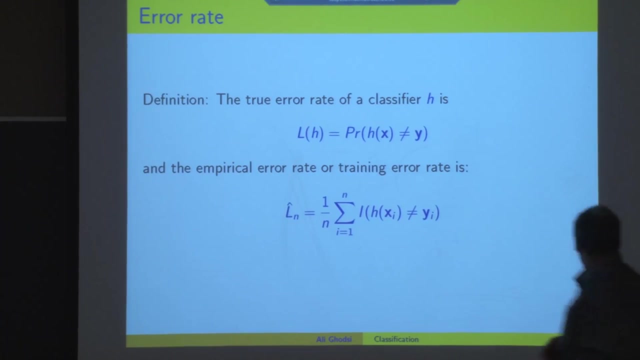 then 10 over 100 is my estimation of the true error, So it's also called training error, okay, Okay, now we come to a very important concept in this course, which is called Bayes classifier. But before I tell you about Bayes classifier, 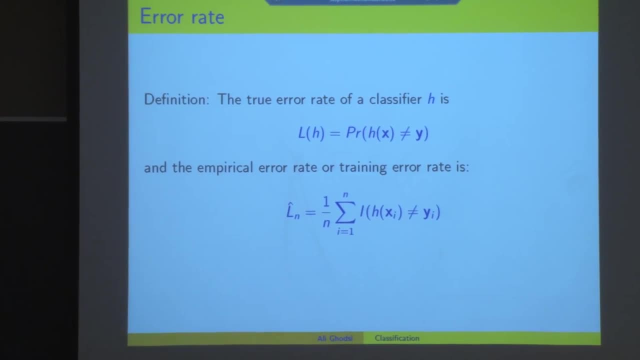 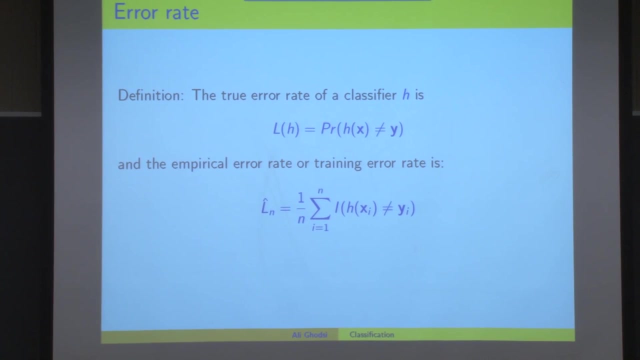 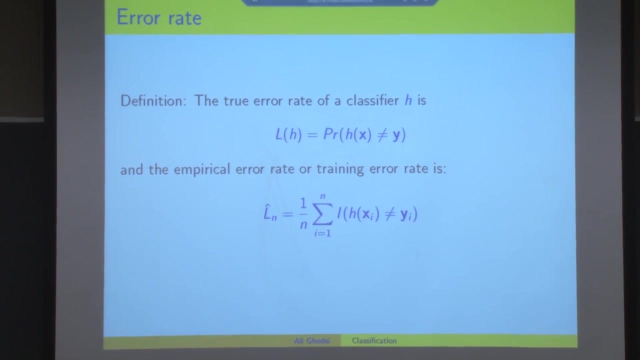 let me ask you a question. You know, suppose that I have labels and I have data, points X, and I would like to compute probability, conditional probability and use conditional probability as a way to do classification. So I would like to know that my set is. 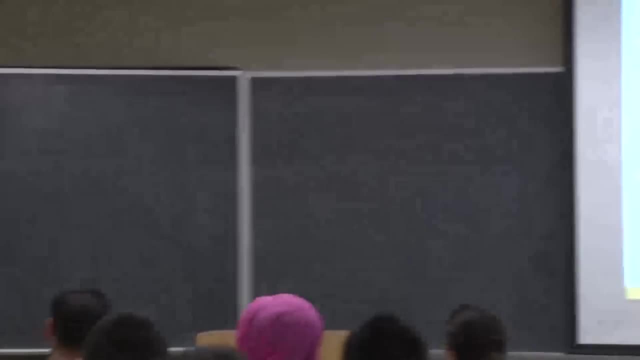 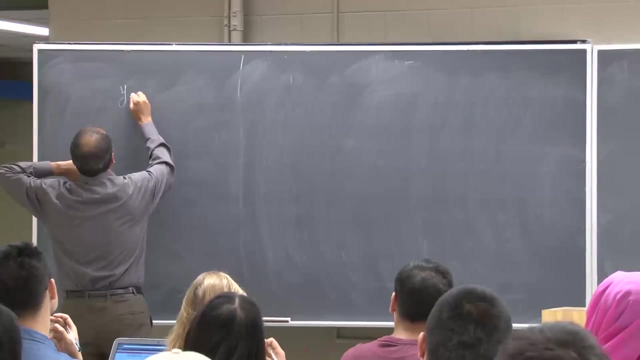 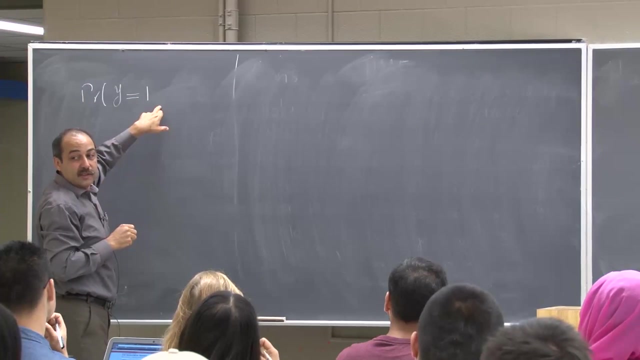 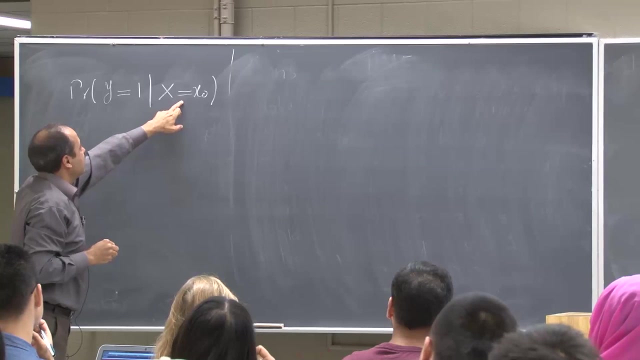 suppose that I have only two class. So you give me an image, and this image is either the image of a picture of Ali or it's John, right? So I can compute the probability that this image is Ali. So you give me this image. what's the chance that it's Ali? 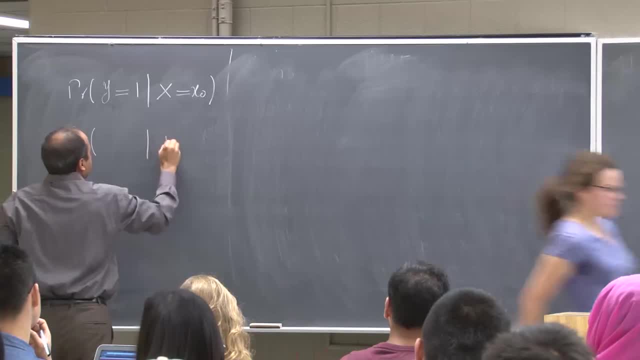 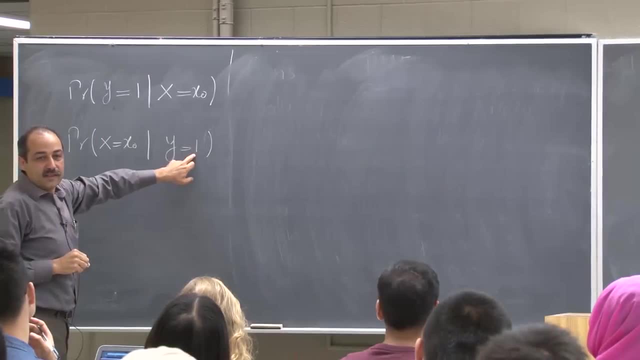 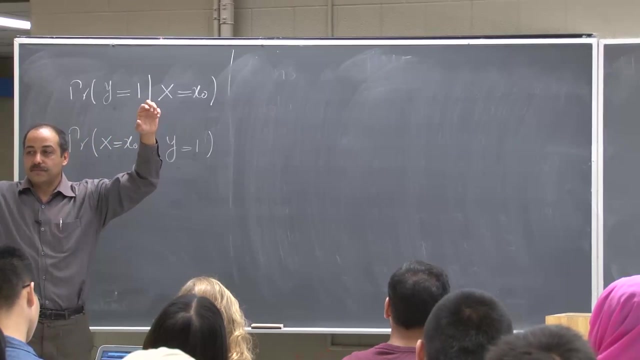 Or I can compute this probability. So, given that this is Ali, what is the chance that I observe this image? Okay, both of these two are meaningful, You know, given that you know, in a stuff two person, let me say Ali and elephant, for example. 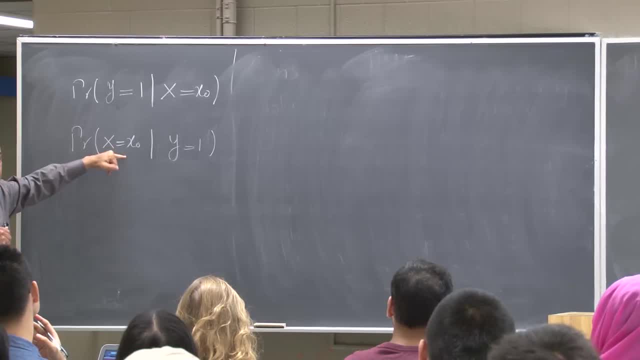 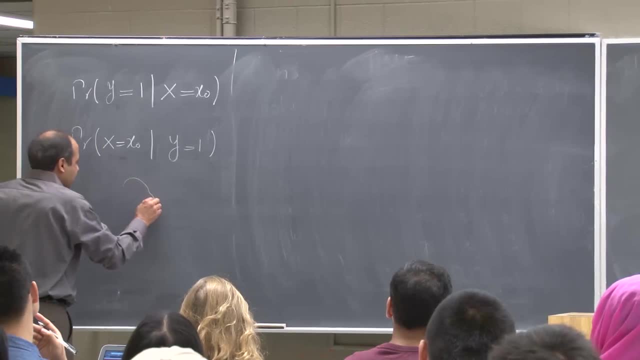 Given that this is Ali, what is the chance that I observe this image? So the chance is very rare that you observe, you know, something like this. given that this is Ali, Right, And here, given that you have observed this image, 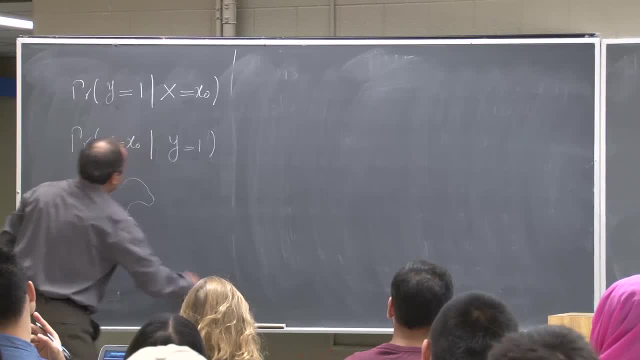 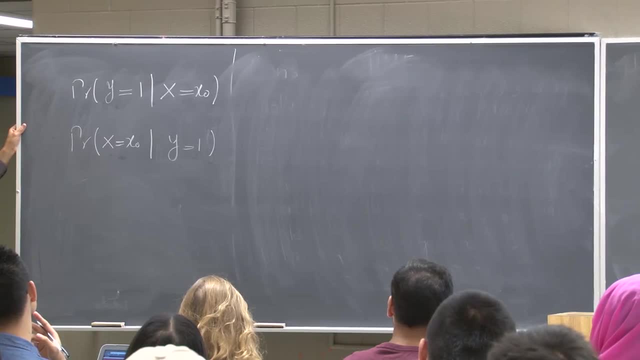 what's the chance that it's Ali? Which one of these two scenario you go for? If I want, if you want to do classification, you go for this one or you go for this one. Who go for the first one? The second one? 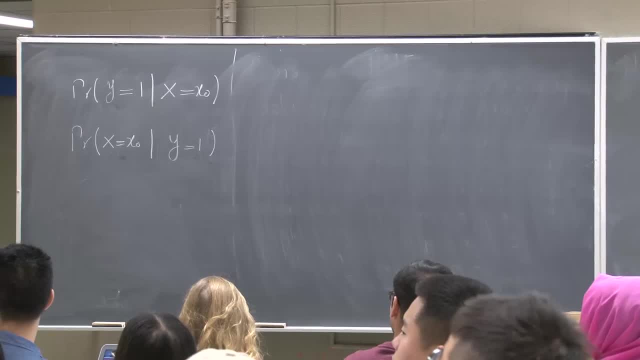 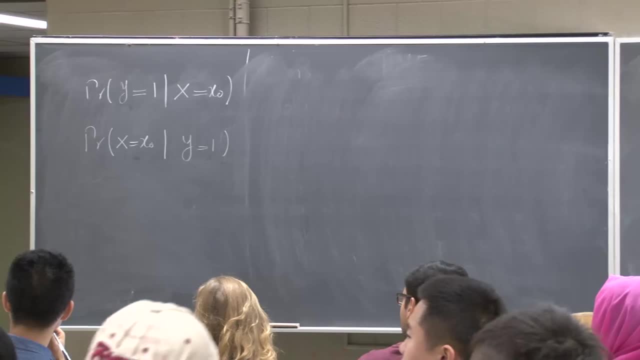 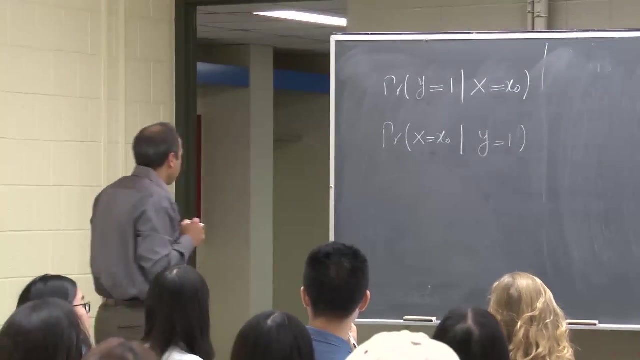 Yes, You go for the second one. Why Can you use the second formula, base formula- and reach to their first? It's better for us. So, yeah, we can reach the first if we use base formula. We can reach the second if we use the first one. 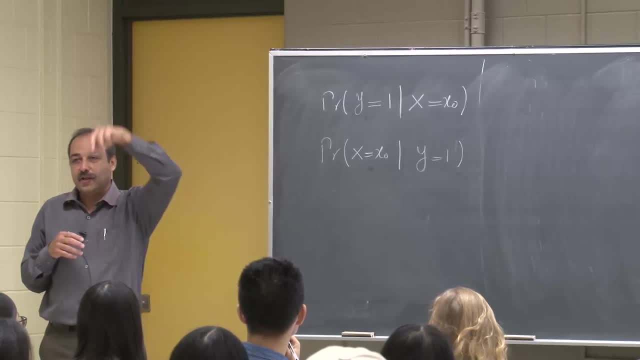 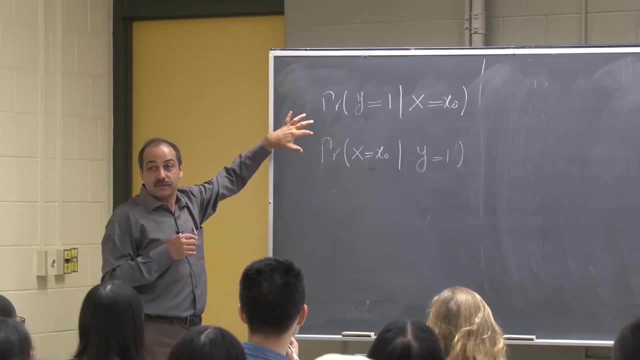 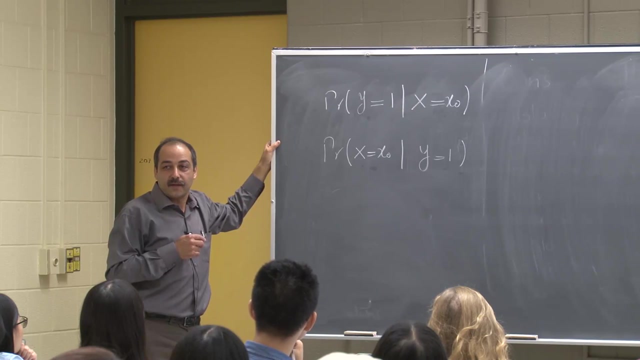 So in this case, you know, we can reach the other one just using base formula. But conceptually is there any advantage from these two? Can we just choose the one that we like, or one of them is better than the other? 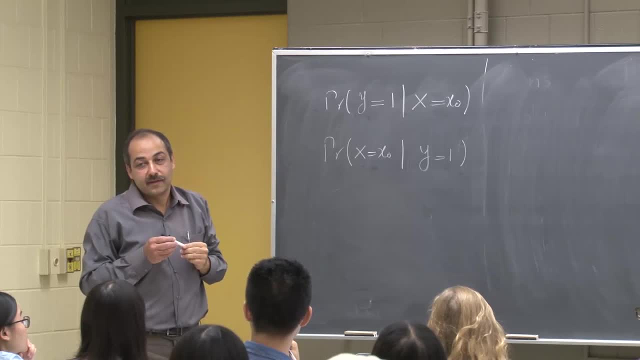 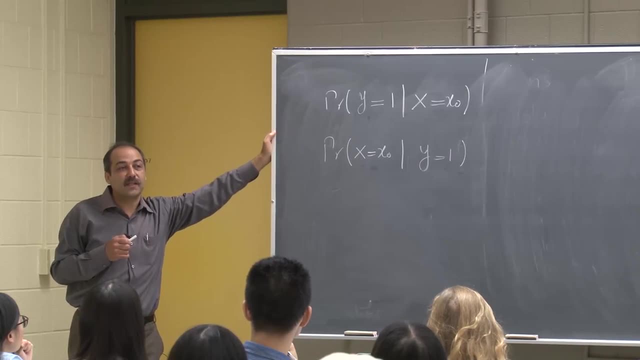 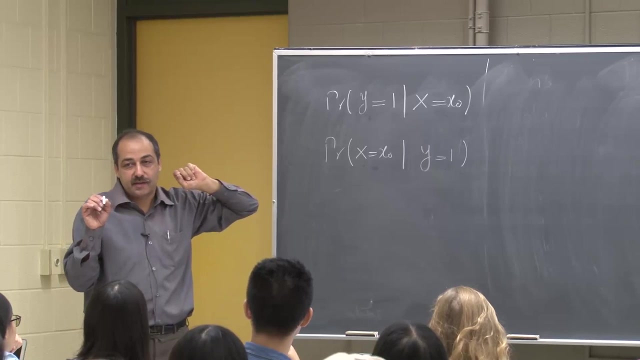 Sorry Isn't easier. Might be, But besides being easy or hard, conceptually, I mean we can. we can talk about easiness. if we think both of them are correct, Then we can think which one is easier to compute and we go for that one. But 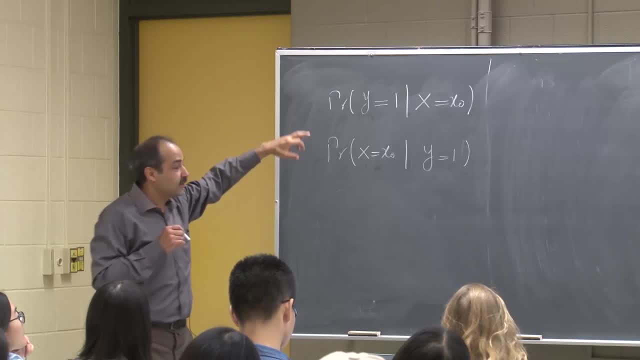 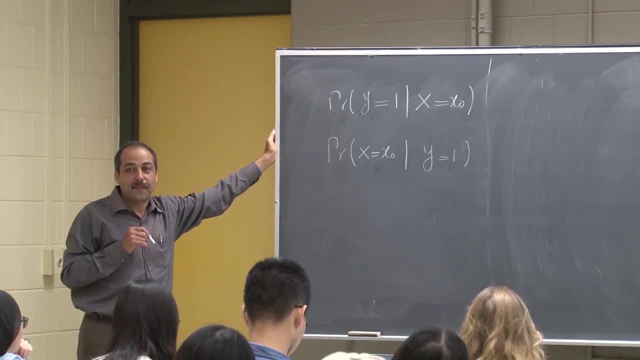 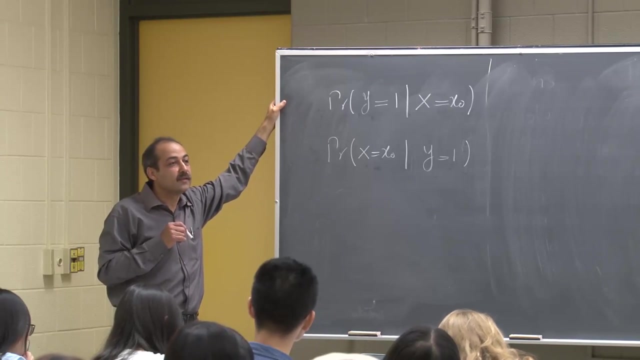 before we get to that stage, we have to make sure that either one is good, But eventually, which one you're going to decide based upon? Yes, Which one? because you're going back to the labels When you're doing like a new classification on unlabeled data. 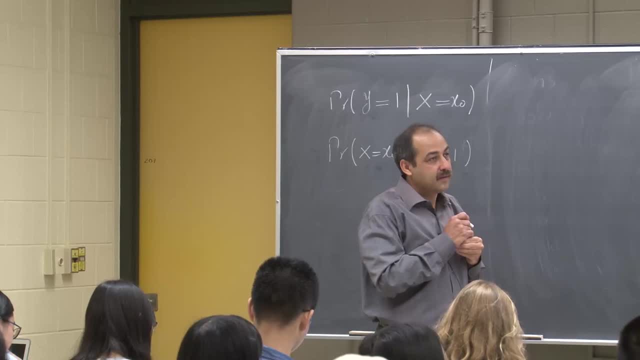 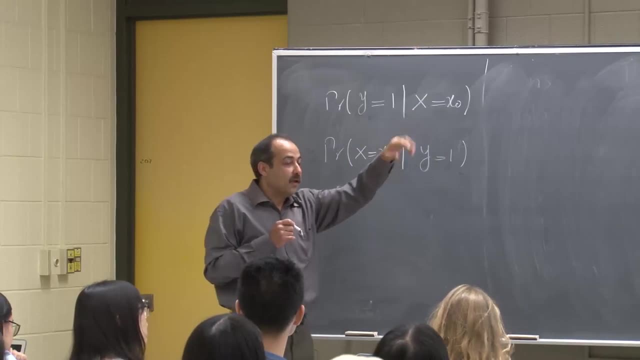 once you turn your classifier, you want to take the probability of the label from the data. so all you have is the data from the new label. No, I can't do that, you know. So you give me an image. you know, I compute what's. 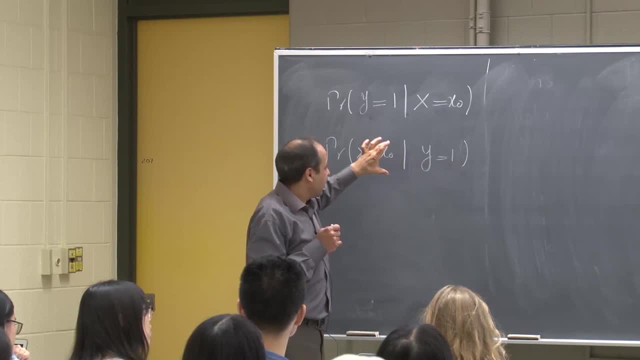 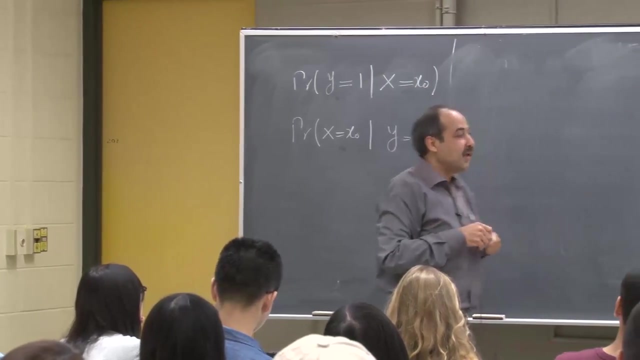 the chance of being elephant and having this picture. Okay, What's the chance of not being elephant and having this picture? I compute both of them and I go for the one which is large, So I can assume both cases of labels. right, That's the same here, actually. 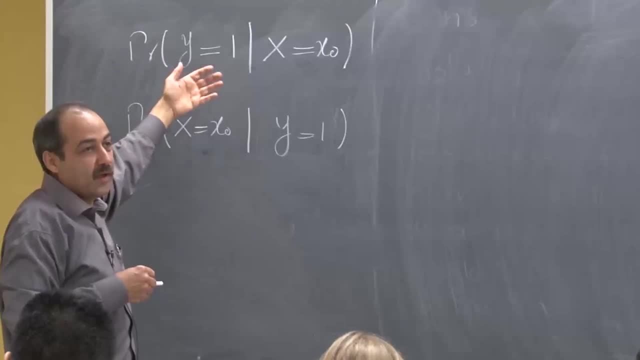 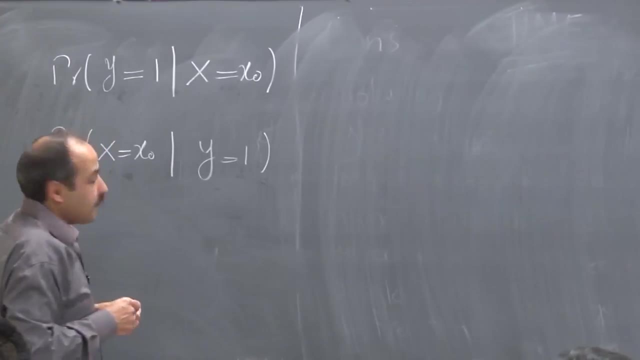 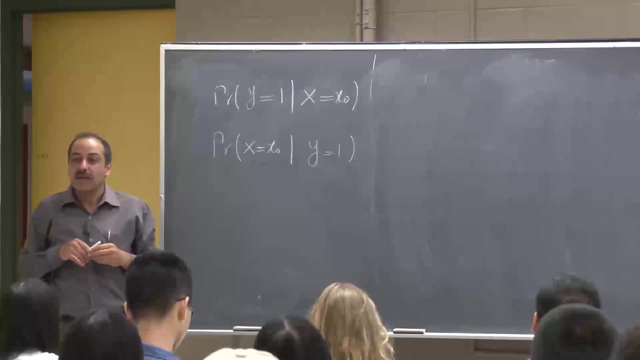 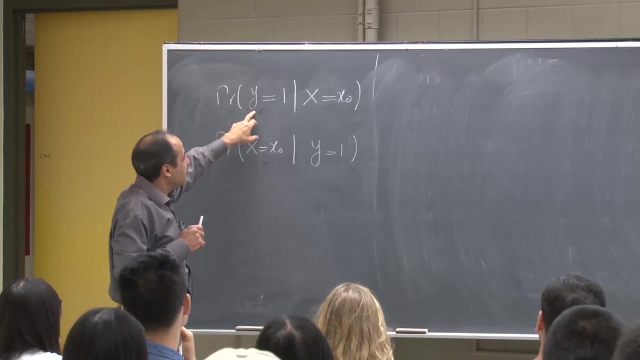 I have to assume something about y and then compute the probability. I can assume both cases. So you know, we can have debates about these two in many different ways, you know. Okay, Even I can argue that you know this one here. actually, y is not even a random variable. 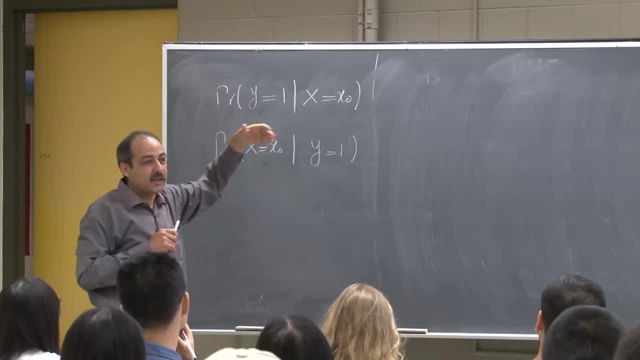 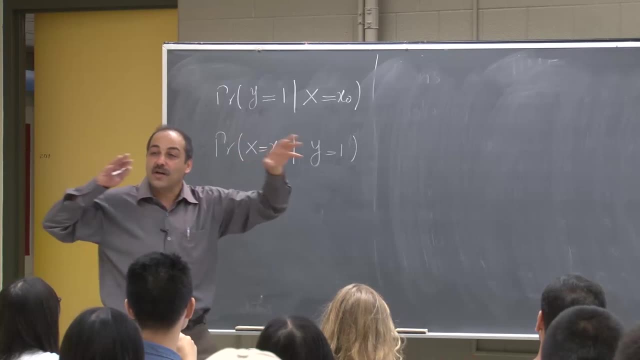 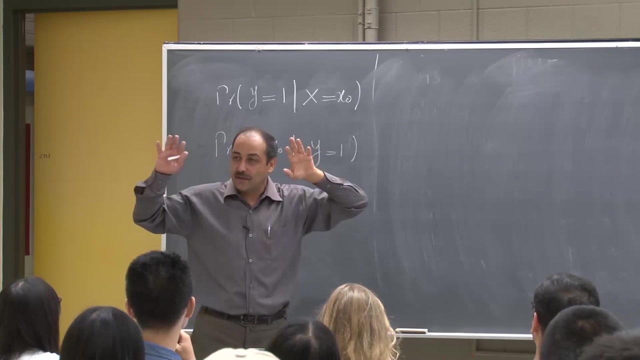 You cannot define probability for y, because it's a label of you know I'm either elite or I'm not elite. There is no randomness here, but there's randomness about images. So we can have arguments from many different aspects. but these philosophical arguments aside, 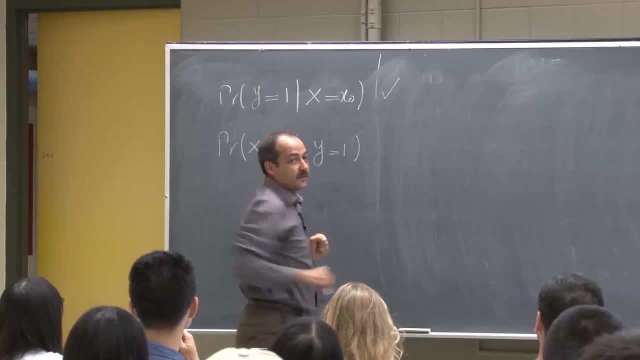 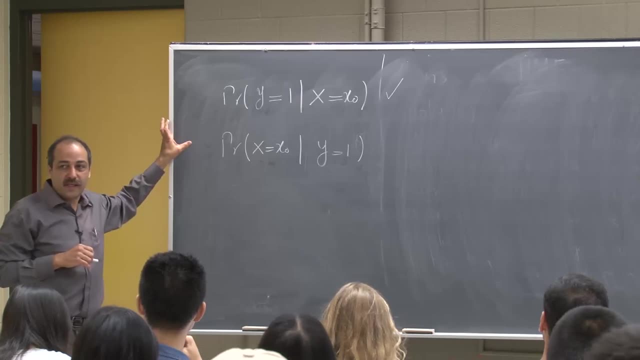 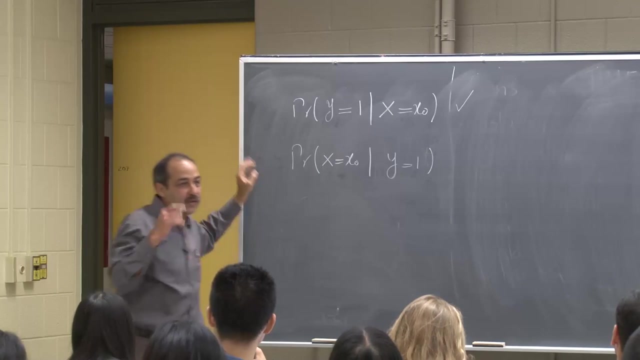 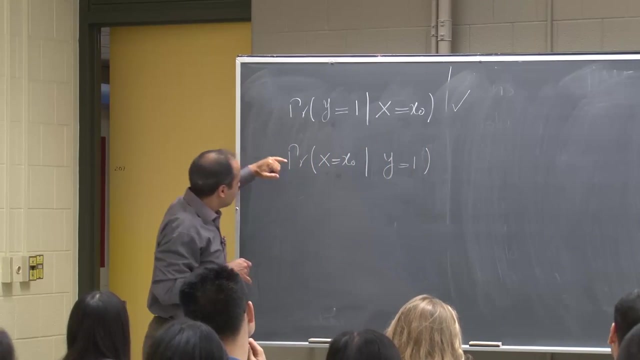 you have to go for this one, not the second. You know there is a very famous mistake which is called the persecutor's fallacy. So it happened in courts in UK and in US many times. There are papers about that that in court they decided based on this probability instead of this one. 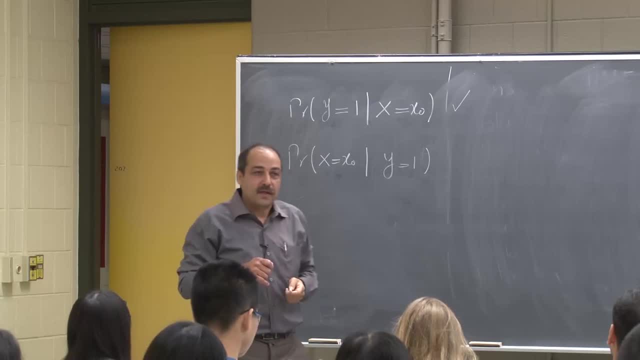 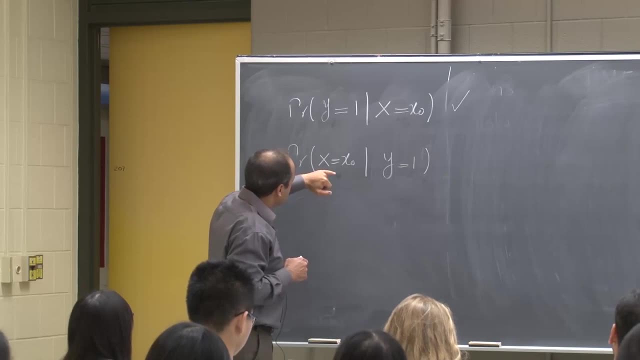 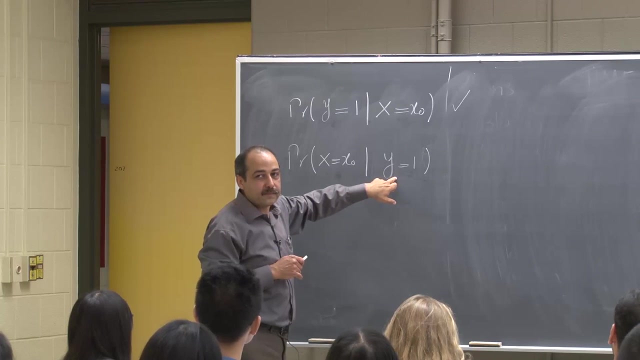 And it's wrong. You know you have a person who is accused for a crime and you have some evidence, So this basically tells you what's the chance of observing this evidence, given that this person is innocent? What's the chance that this person is innocent, given that I have observed this evidence? 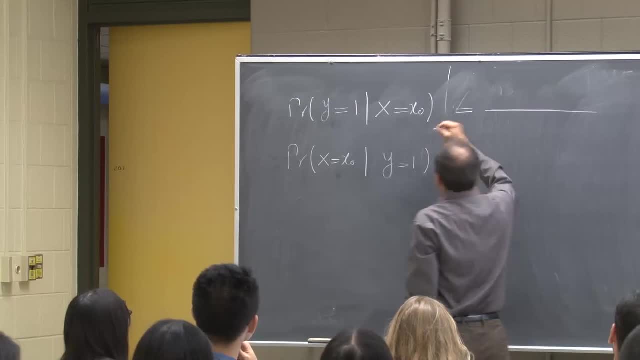 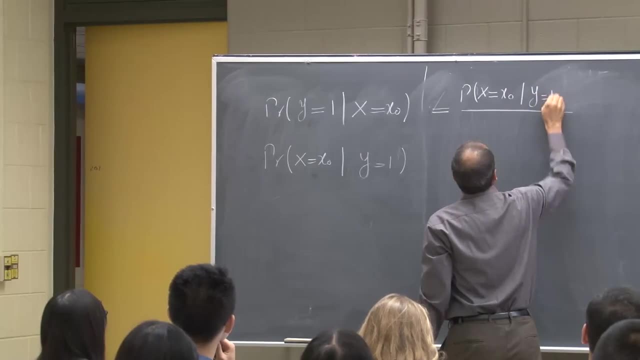 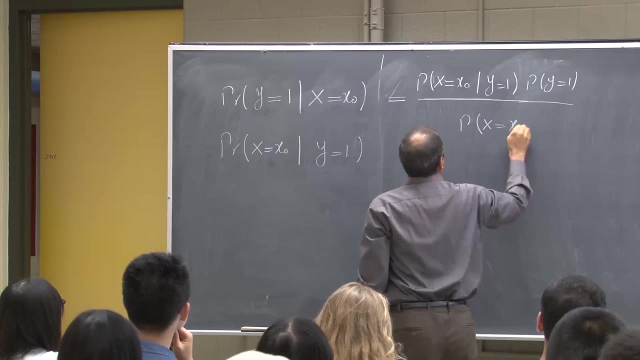 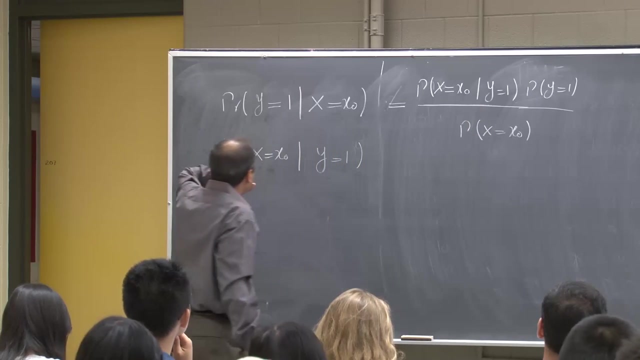 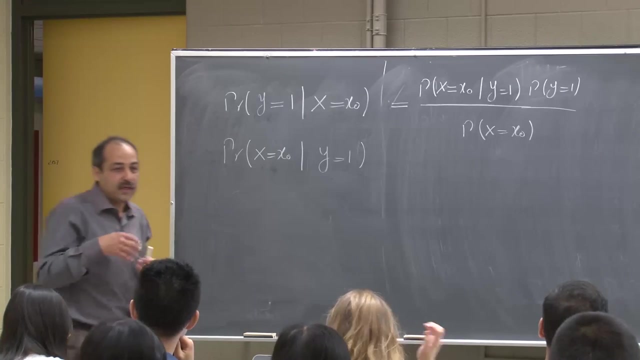 According to Bayes' rule. you know this probability is px. According to Bayes' rule, I can write this probability this way: Okay, And so what happened in many cases is that you know there's a very famous court in the 90s that a lady was accused of killing her own children. You know, one of them died after 16 weeks, The other one died after 8 weeks And a witness in the court, who was an expert, testified that the chance of two children in the same household or died is, I think, 1 over 75 million. 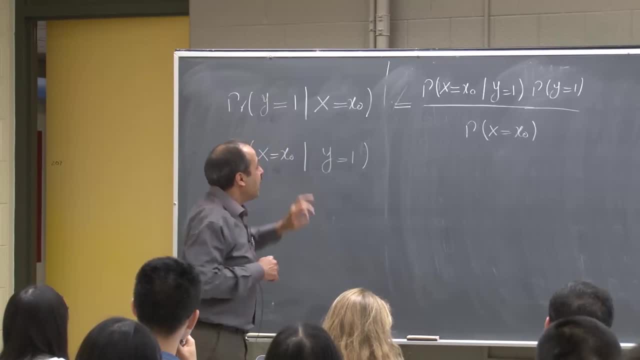 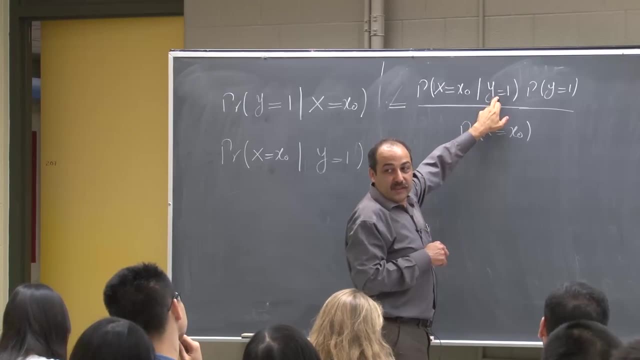 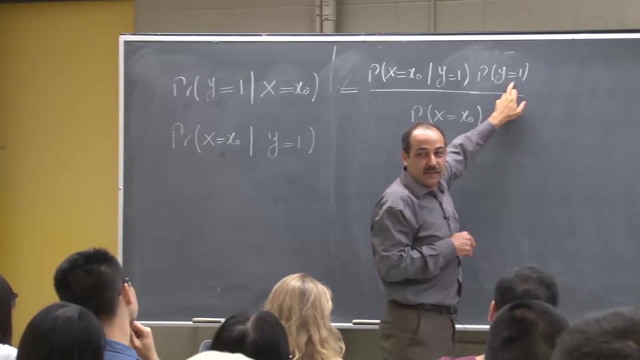 It's very, very small And court decided based on that. But you can see that. you know. suppose that the chance of observing an evidence given that this person is innocent is very small. It's still the prior. The chance that the person is innocent could be quite large. 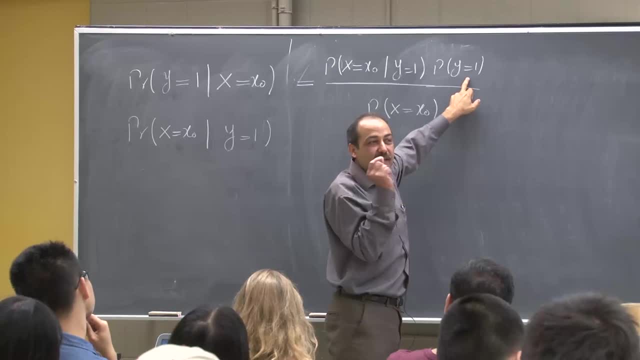 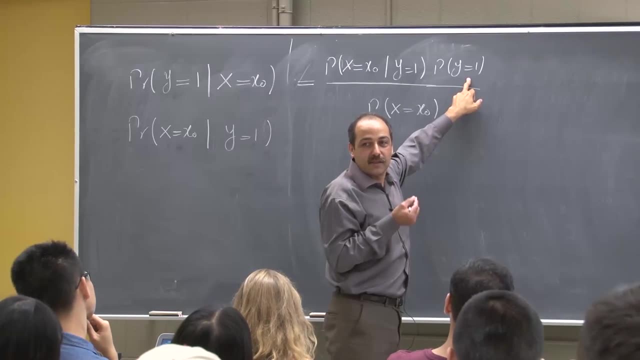 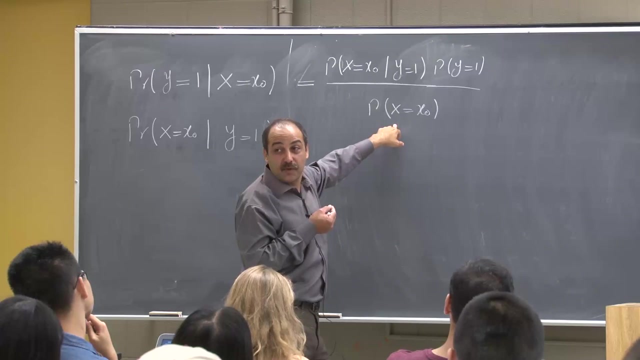 If you look at the whole population, only a very small proportion of the whole population are guilty or criminal. Most of them are innocent. You know this could be pretty large. Even the marginal probability could be pretty small. You know the chance that you observe such evidence without you know condition or anything. 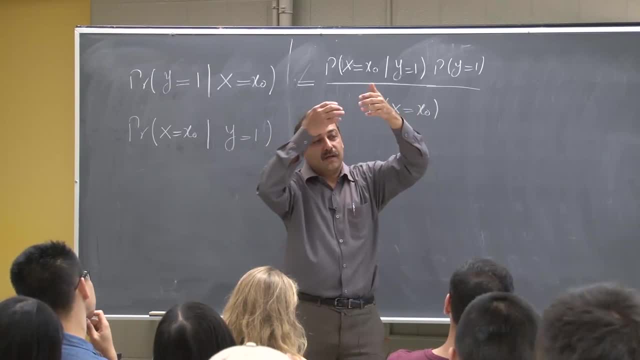 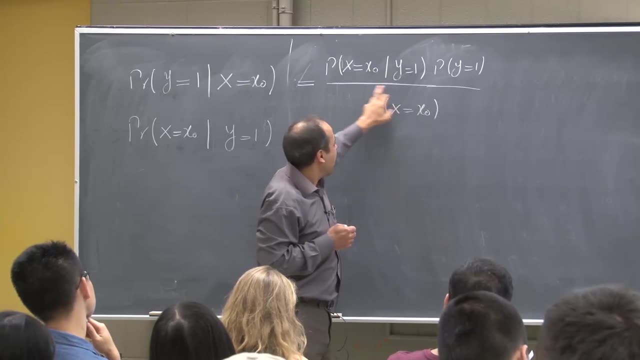 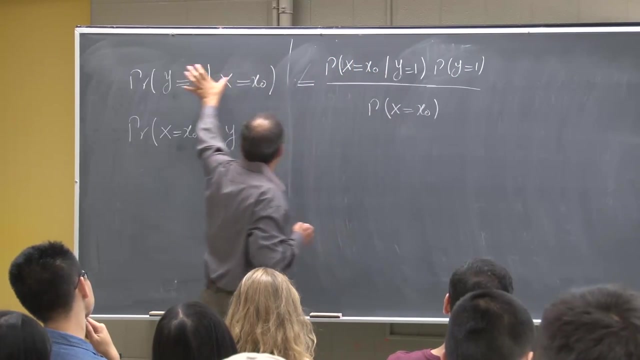 regardless that the person is guilty or is not guilty, was the chance that you know two children died. It's small, So having this small denominator, having this large amount here, even this, if this is small, this could be large. 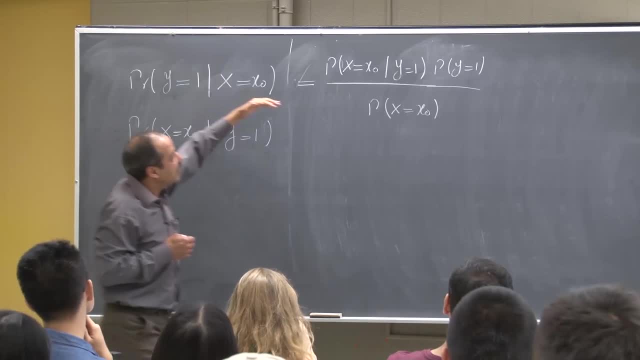 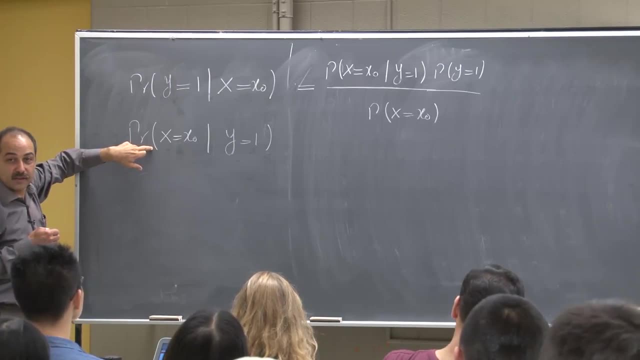 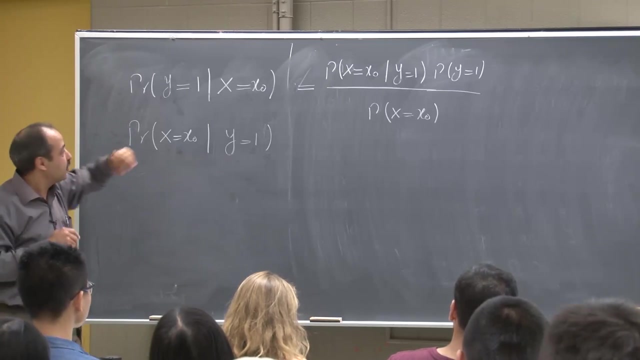 So the chance of a person is innocent, even if you have a very rare evidence, could be quite large. But many courts went for this decision by mistake in the past. So I mean, in your first assignment actually, you're going to prove that this is the best thing that you can do theoretically. 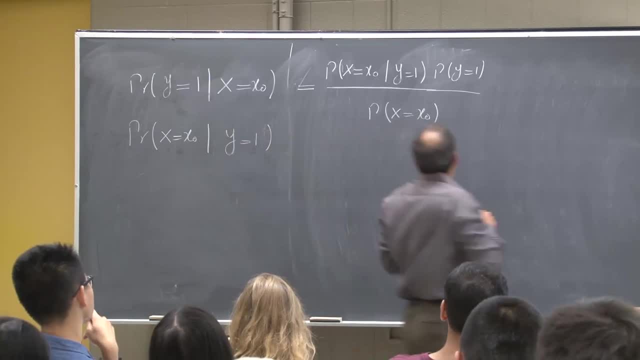 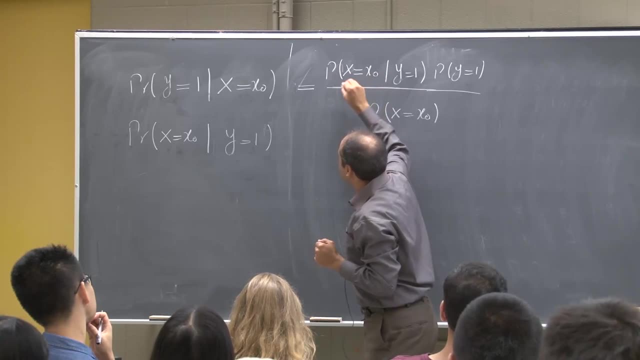 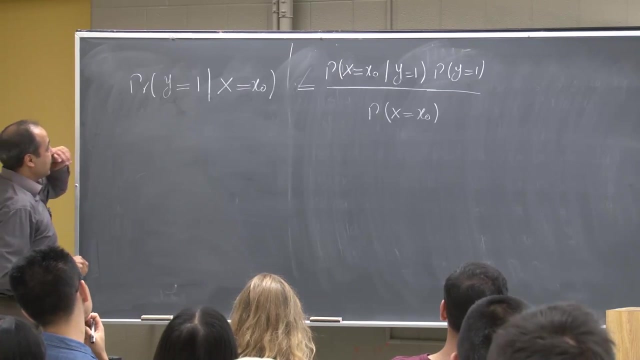 You know you will see the mathematical argument, but at intuitive level. So at the moment, accept and believe that this is actually what you have to do. So if you want to do classification and you have, say, for example, two classes, 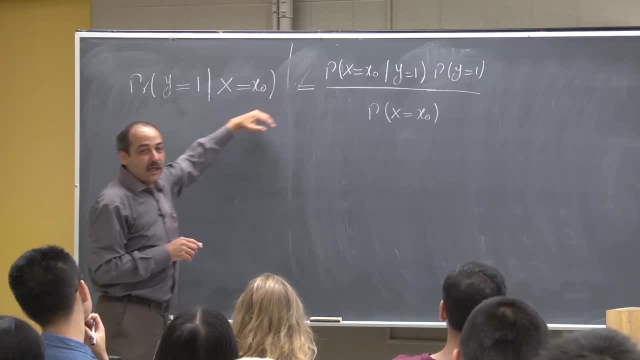 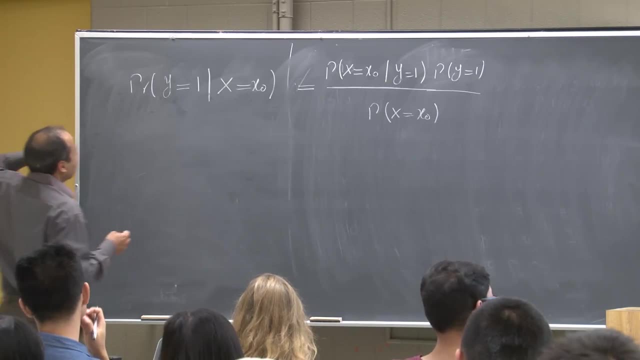 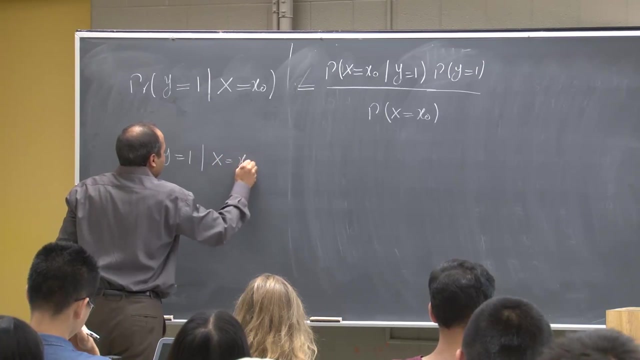 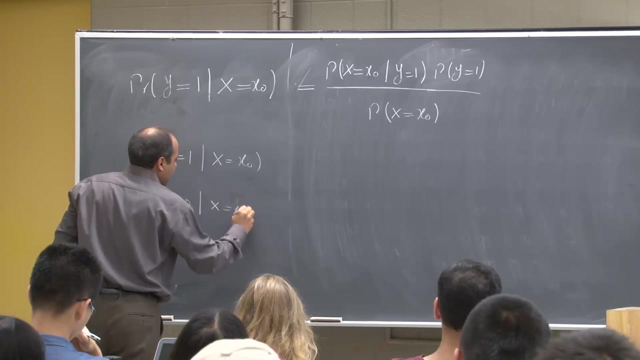 that's the probability that you have to compute, And this is called base classifier. Okay, So basically, base classifier means that I have two classes. I compute py equal to one given x. I compute py equal to zero given x, And I go for the one which is large. 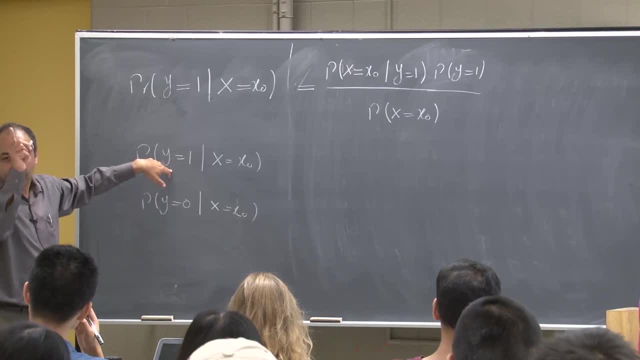 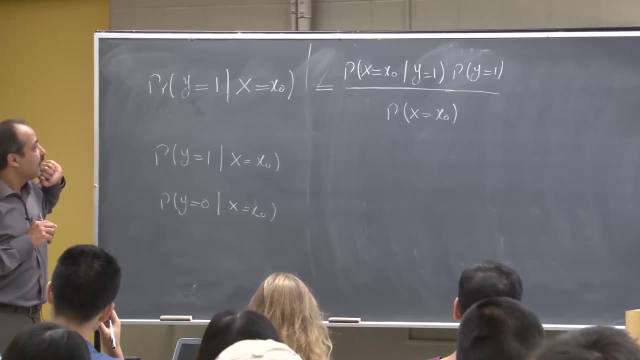 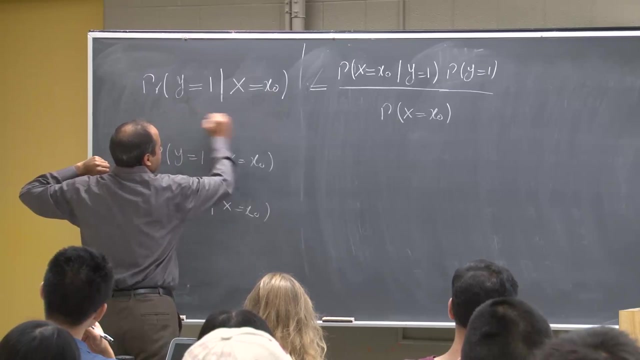 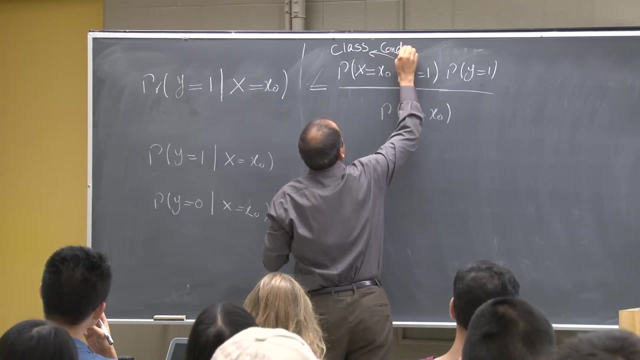 If this is more than half, I will decide label one. If this is more than half, I will decide label zero. This is called base classifier. Okay, And again a little bit of terminology. So this is called posterior, This is called class conditional. 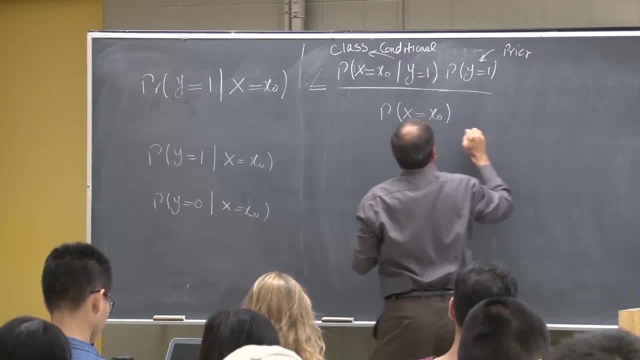 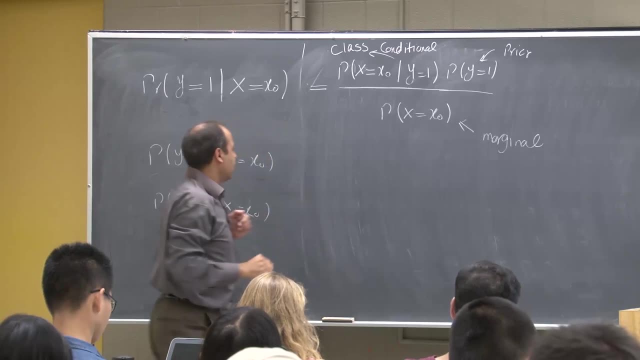 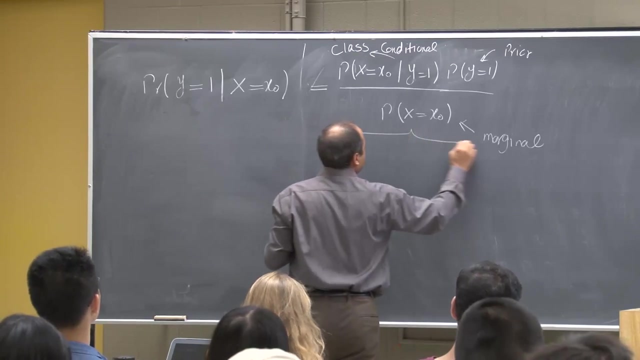 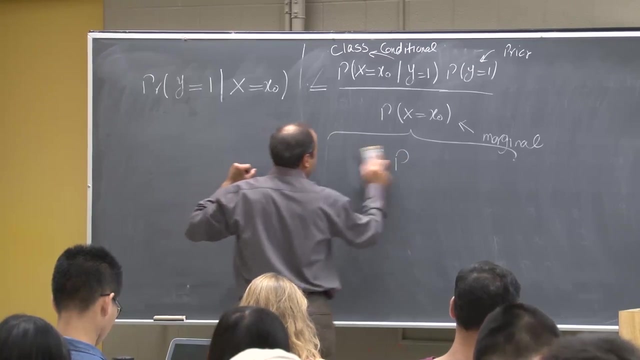 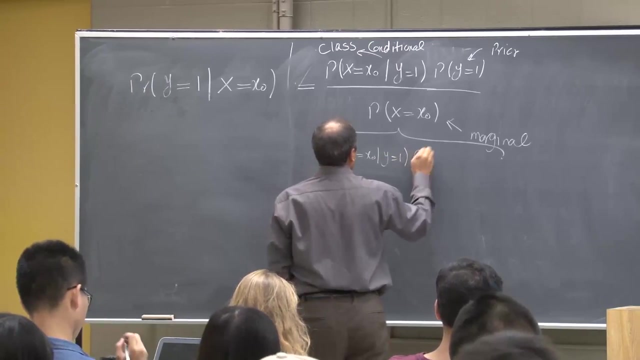 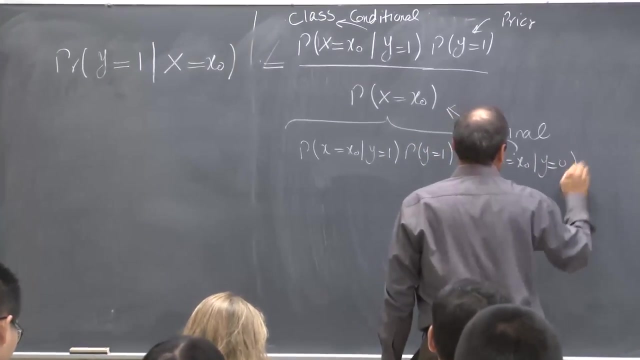 This is called prior And this is called marginal, And you know that this Marginal is in fact, you know, summation over. Let me write it because we have only two classes: It's p, x being x zero, y equal to one times y, one plus p being zero times. 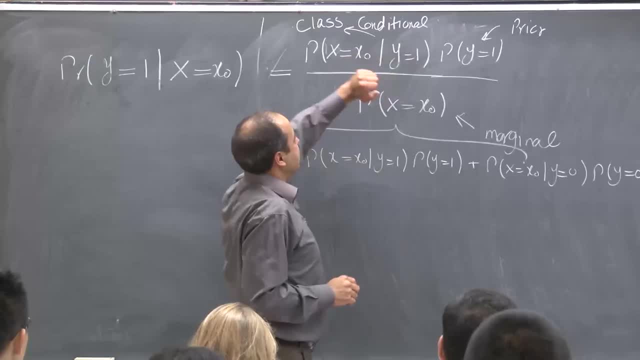 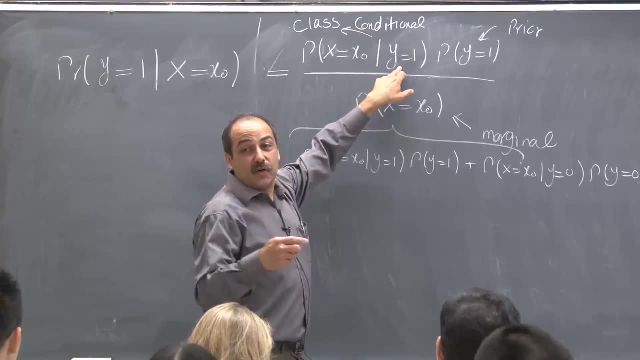 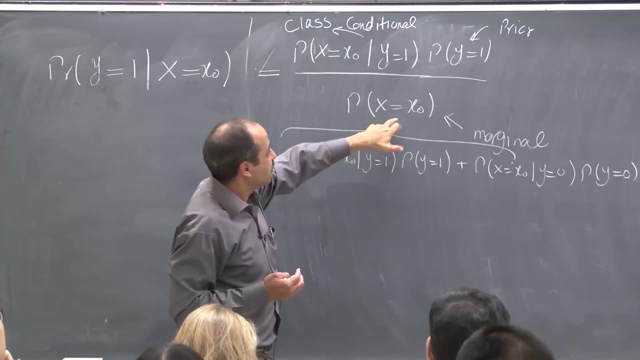 Okay, So it's not an independent quantity. It depends on class conditional and prior. So class conditional, because if I conditional only on one class class that has label one, what's the distribution of the date? And this is marginal, because if I don't condition on any classes, 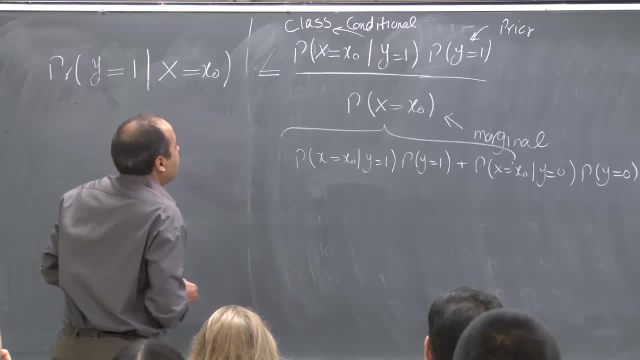 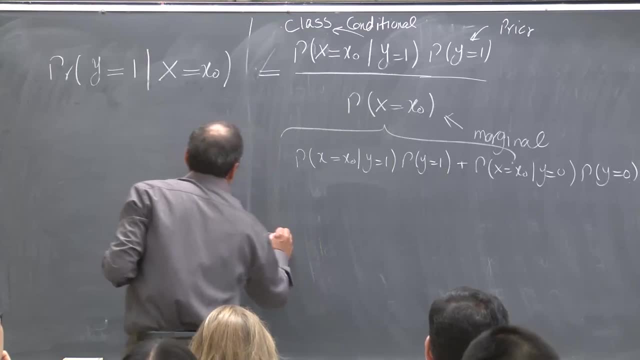 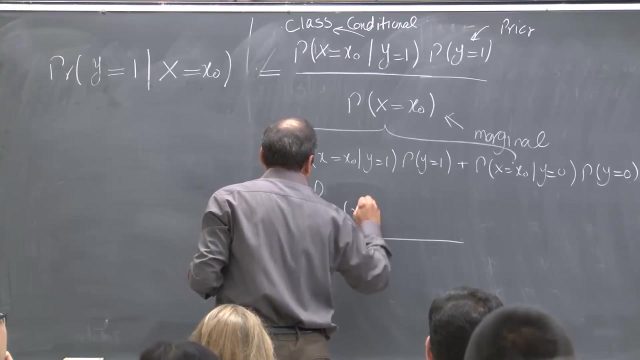 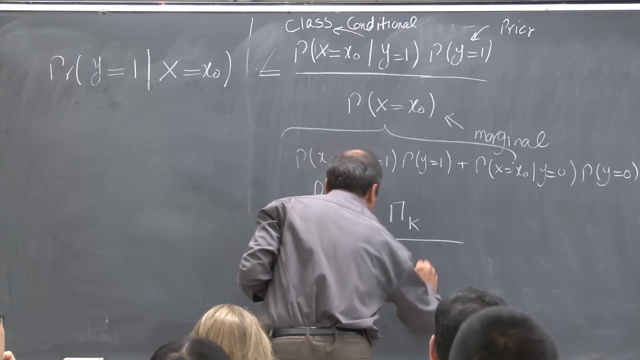 what's the distribution of the date, And this is prior. What's my belief about being in class one, Or what's my belief of being in class two, And usually we use this notation. So I use this for class conditional, I use this for prior. 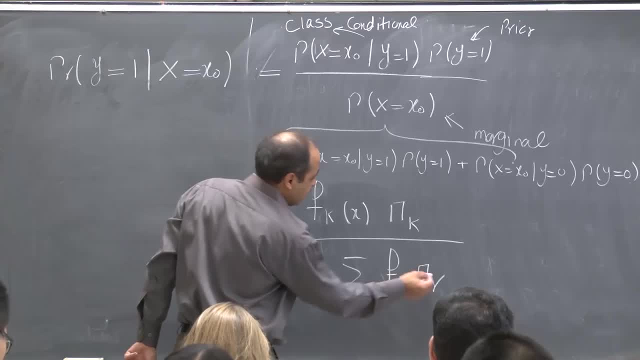 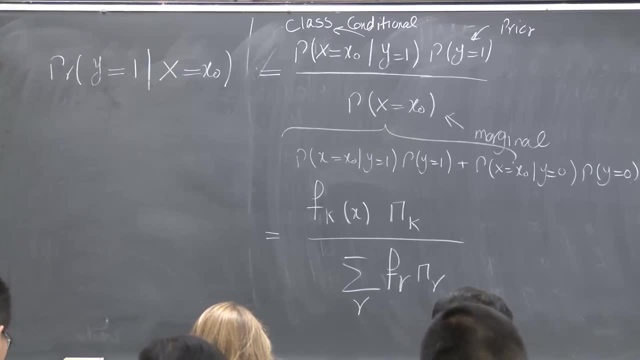 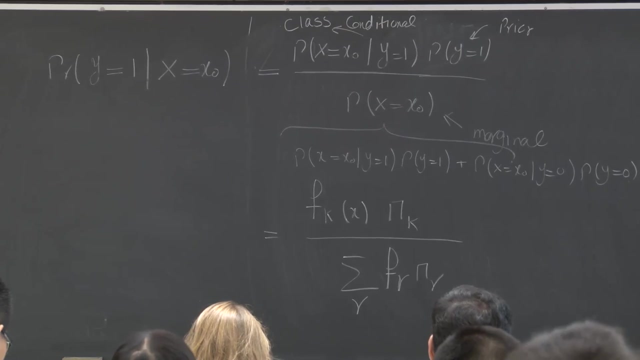 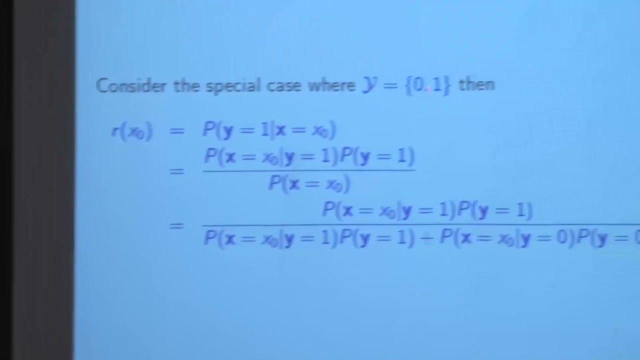 And this is my marginal, which is just summation of class conditional times, marginal over all possible values of y. Okay, Any questions? So this is the definition of base class. Suppose that I have two classes, as I said, and then you compute this conditional probability. 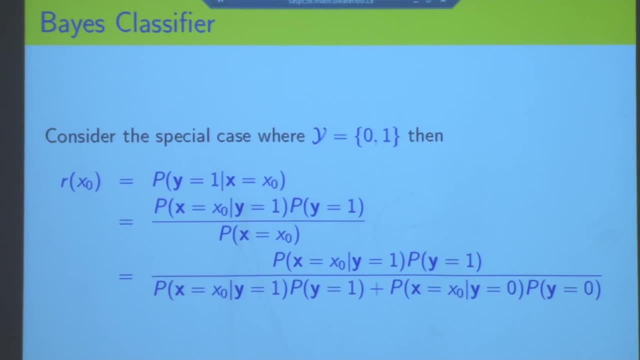 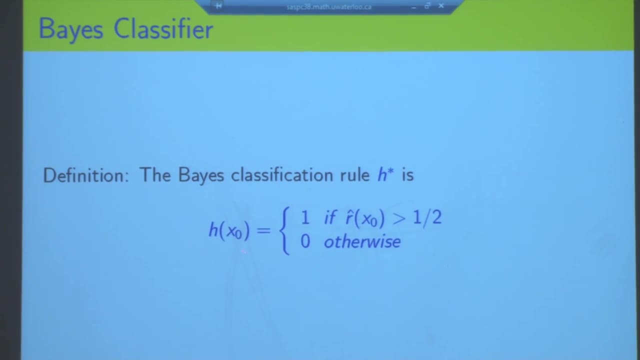 and you can write this conditional probability as base rule And then you know if this quantity is p, y being one, given the observation, then base classifier can be defined this way: If this probability is more than half, I will label this to class one. 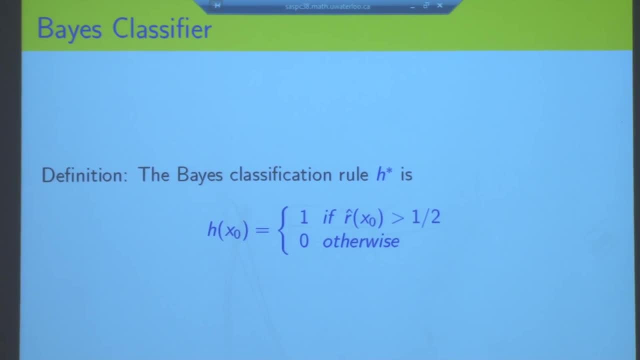 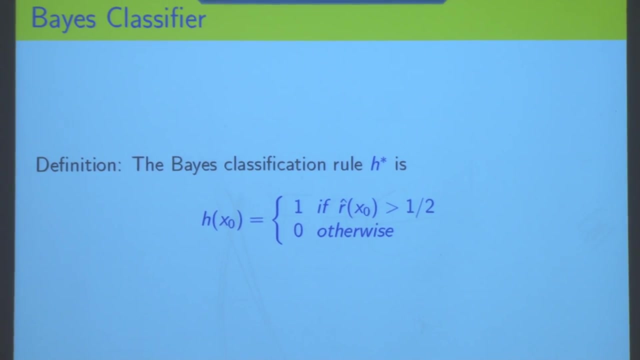 If it's less than half, I will label it to class zero. So simply, I compute the conditional probability y given x, And for two cases- either y is one or y is zero- I go for the one which is larger and label the data that way. 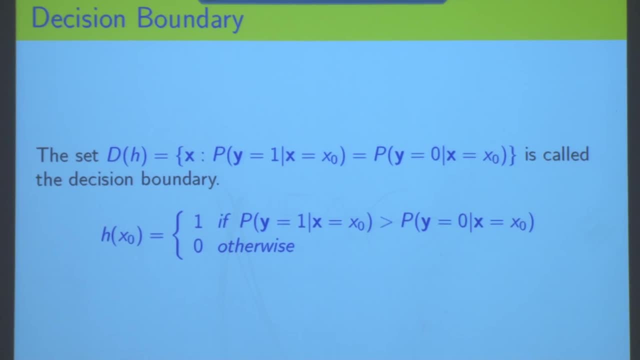 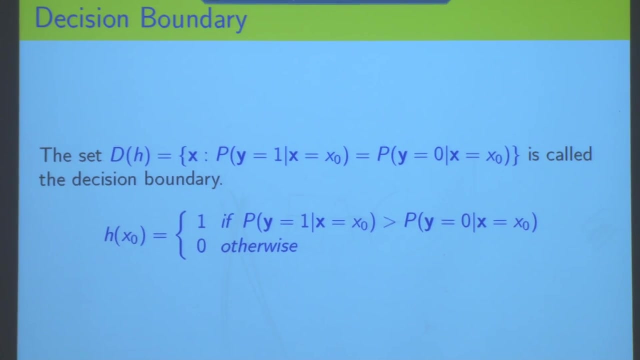 Okay, Another definition: decision boundary. So decision boundary is set of points such that the probability of being in class one is the same as probability of being in class zero. So in base classifier we would like to assign one to all points that are in class one. 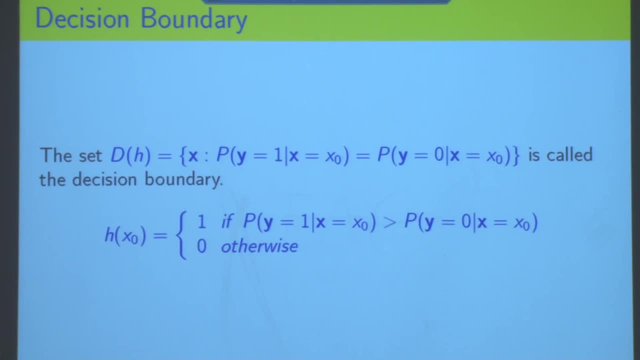 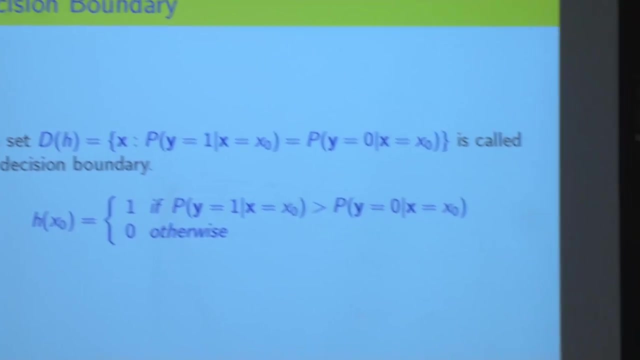 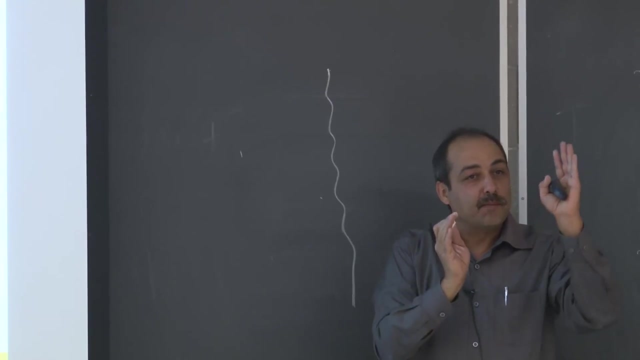 assign label zero to all points that are in the other class. But there is set of points such that probability there is set of points such that probability of being in class one is the same as probability of being on the other class. So it's important geometrically because it's sort of a boundary. 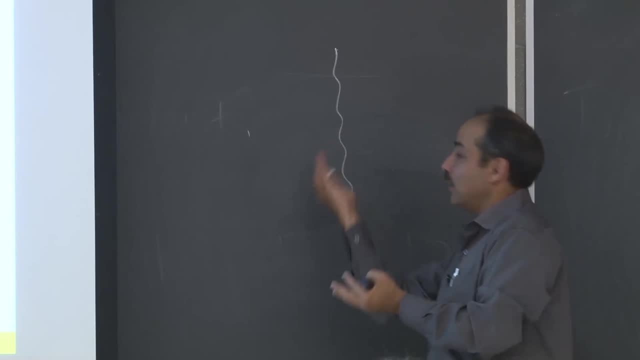 that I can make my decision upon this boundary. You know, any point on this side have larger probability for class one, Any point on the other side has larger probability for class zero And anything on this boundary have the same probability for both class. 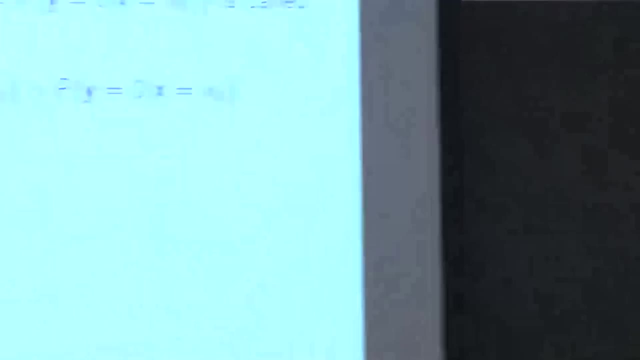 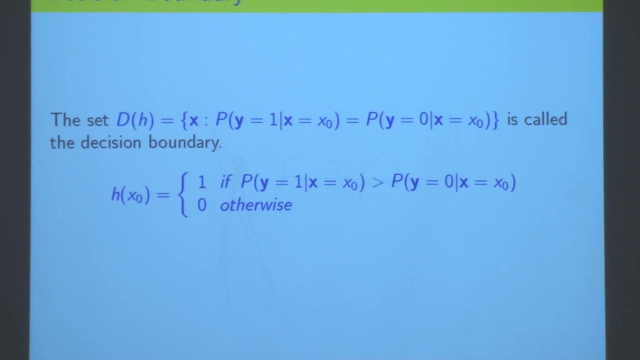 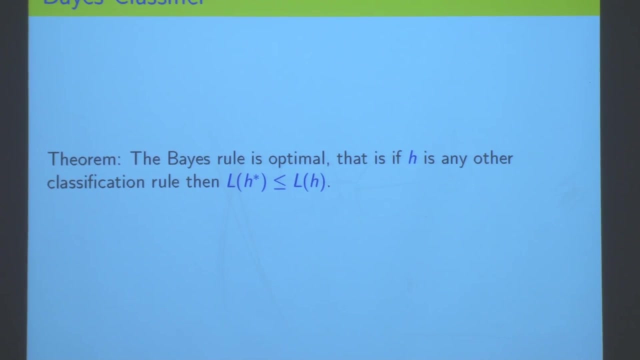 So this is called decision boundary. And then if you have decision boundary, then the base classifier assign label one. if you know you're on one side of this line, Okay, And zero other way, Okay. There is a theorem that you're going to prove in your first assignment. 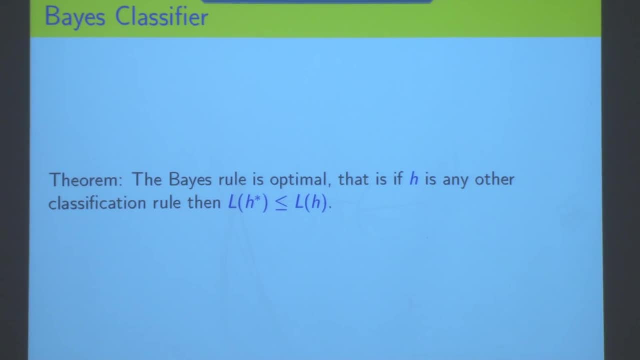 that the base rule is optimal. What does it mean that it's optimal? It means that if you compute the true error rate for base classifier and compute true error rate for any other classifier, So H is any other classifier And H star is base classifier. 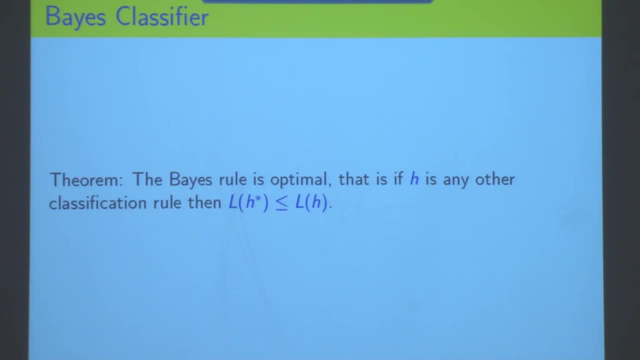 Then the true error rate of base classifier is definitely less than any other classifier. So that's the best thing that you can do for classification. Okay, Yes, Well, maybe, Because that's my question- What do we need any other method? 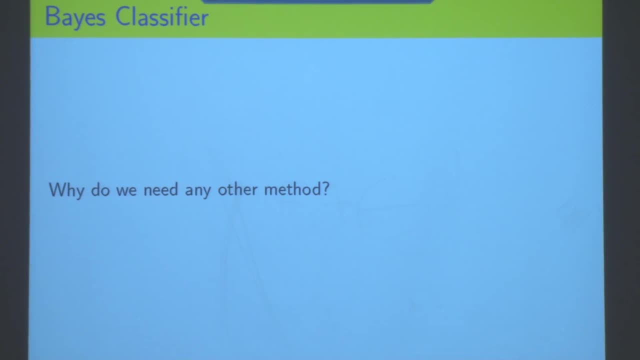 I mean we are done. you know Classification course is done. So we learned about base classifier. We can prove that the base classifier is the best classifier And you can't beat base classifier. Not because we don't know any better method at the moment. 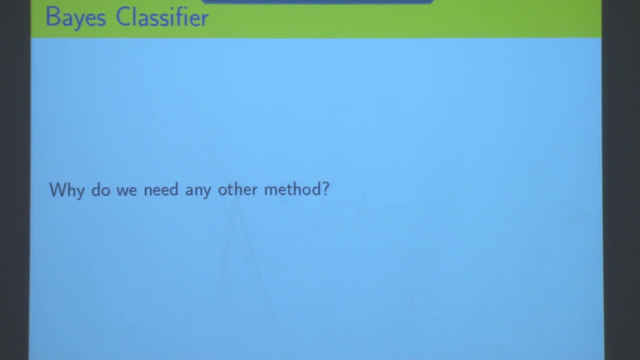 It's mathematical bound. You know You can't beat this bound. Not now, Forever, From now, under the day of judgment. there's no better classifier Guaranteed Okay. So why do we need any other method? Why don't we just use base classifier for everything? 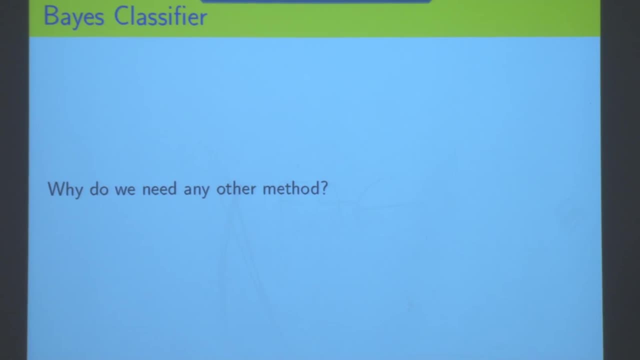 Yes, Sorry Time. What type of time? complexity, I don't know. Like you can't like solve, like using the bias rule in the computing, computing powers that we have so far, Probably Okay. Any other idea? 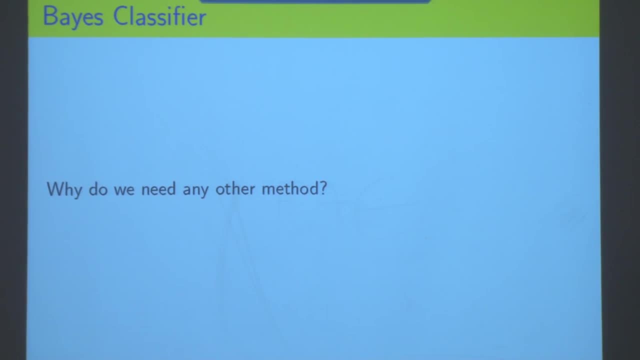 Yes, Yes. So number of dat computation. I think you have seen, you know, many competitions. Some of them even get news coverage these days, You know. 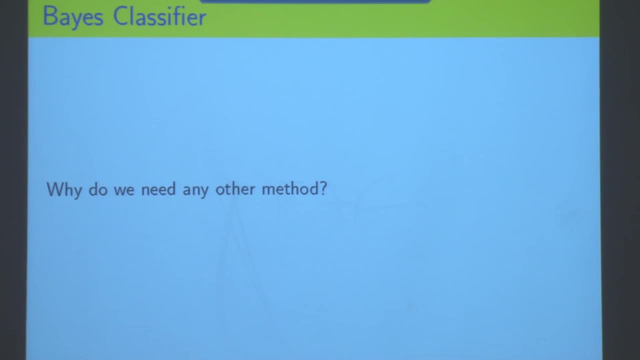 That there's a competition on ImageNet, for example, They had millions of data points. still, you know the Wiener is. you know a model that has been trained by deep network, for example. no one use base class for you don't have priors in advance. 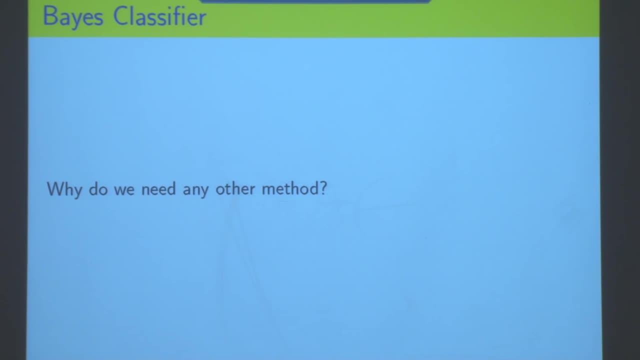 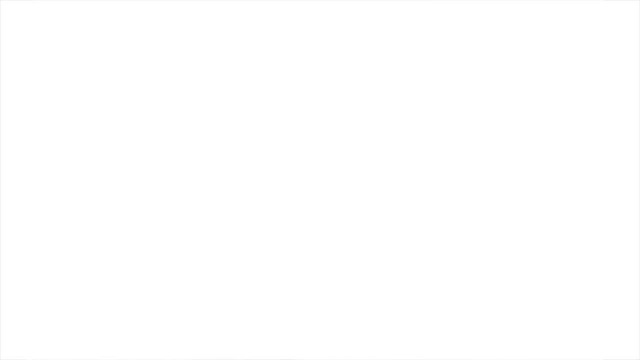 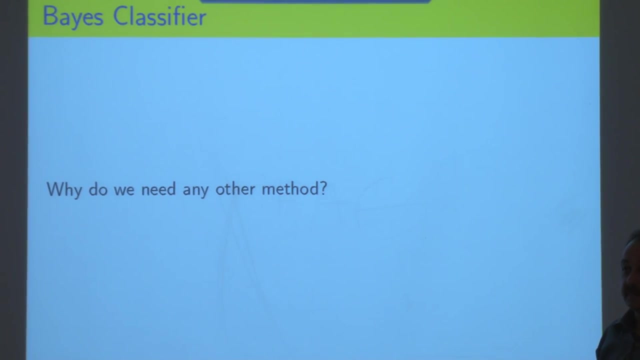 mm-hmm. no, you can extend it to multi-class. easy you just, if you have K classes, you just compute priority of being in class one and two, three, four up to K and you go for the one which is large. so, yes, you don't have prior, not only prior. actually. the problem is that we don't. 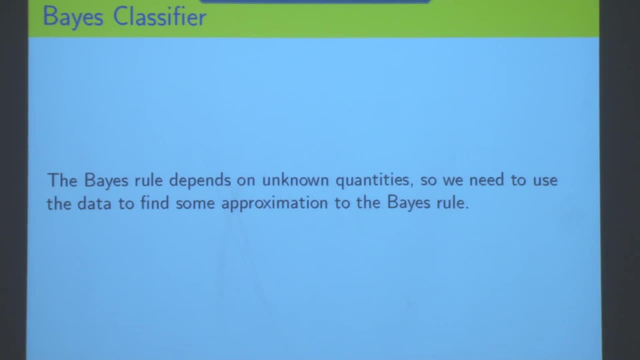 have any of these quantities. you know we don't have distribution of class conditional, we don't have marginal distribution and we don't have the prior. prior is the most easiest one actually to compute. you know prior, you can estimate it very easily because if I have 100 data points and 50 of them are class 1 and 50 of them are 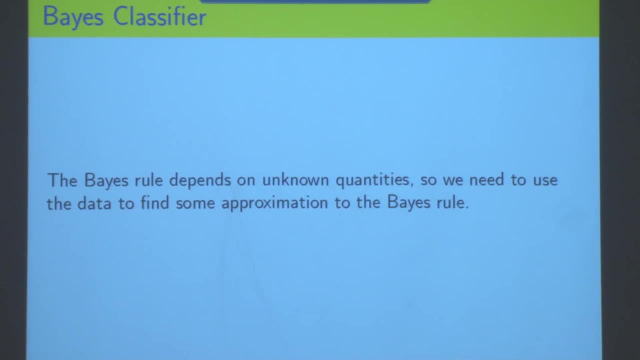 class 0, I can say my prior is 1, half, you know, I believe, is that half of the time. there. it's a very good estimation. so just assume that there is Bernoulli distribution here. but what about marginal? or what about class conditional? you know, you give me a set of images which the distribution of this image is. 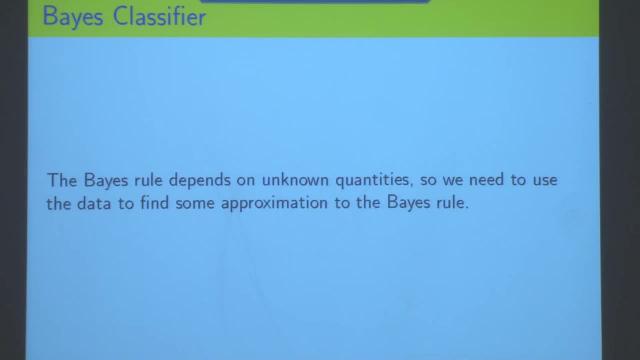 what's P of X? I don't know, you know, if I know what the distribution of this images is. it means that they can sample from this distribution and generate new images that look like elephant, look like Ali or whatever. so I don't have this distribution with the class conditional distribution. if you give me, I'm in this. 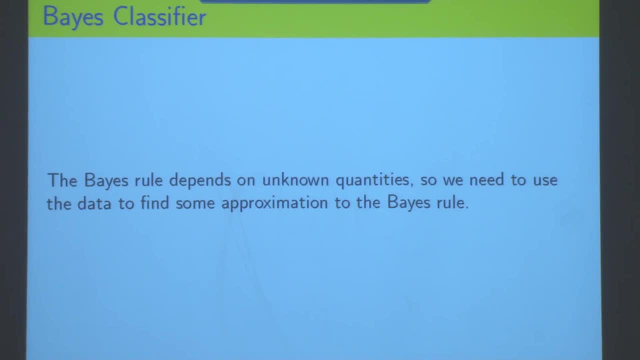 class. can you tell me what the distribution of the points are, and imagine that this points are in very high dimensional space? you know so. we know very, you know, we know what, what distributions we are familiar with. you know Bernoulli, we know uniform, we know Gaussian, so on. they are, you know. 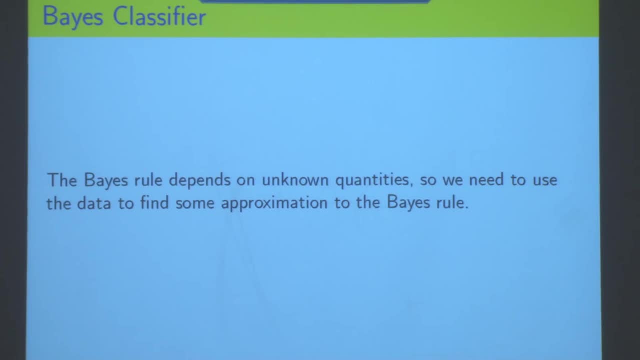 pretty simple distributions. but who can say that? you know, the distribution of images is Gaussian, the distribution of images is uniform or whatever. you know they are not that simple. they're very more complicated distribution. so the main problem is that we don't have distribution. we don't have this. 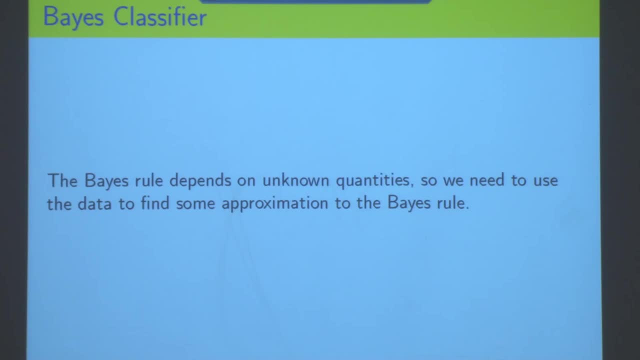 this way. if we do, then we are done. we can do better than base, definitely. so that's the main problem. so, because we can do this, you know there are many different methods, you know. so one method would be: so we don't know this. let's to estimate them. let's to 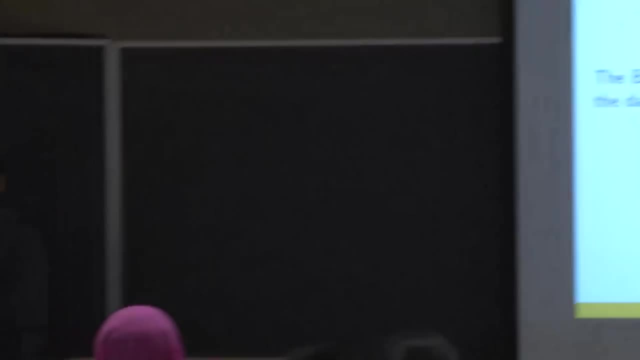 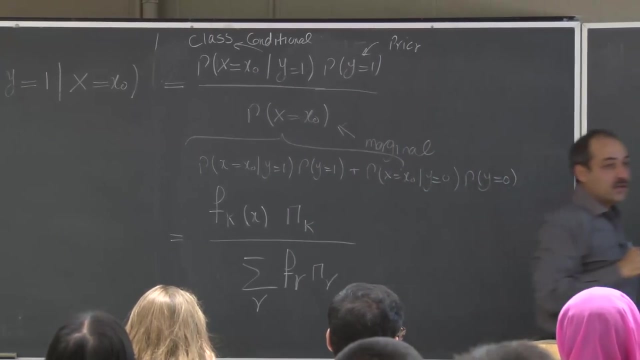 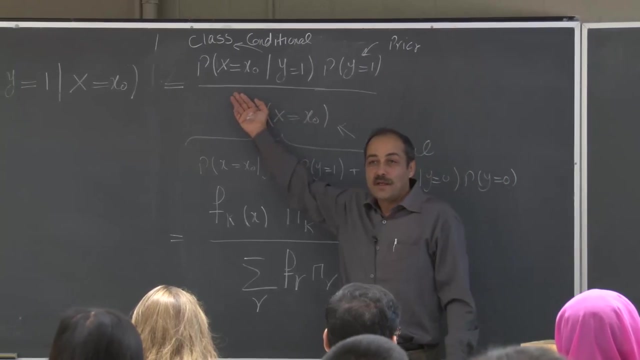 estimate this distribution so we can estimate this prior easily. you know, just by counting the number of points in this class and the other class. let's estimate this one, let this one. so there are techniques for density estimation statistics. we can use those techniques you know for density estimation. why don't we do that for? 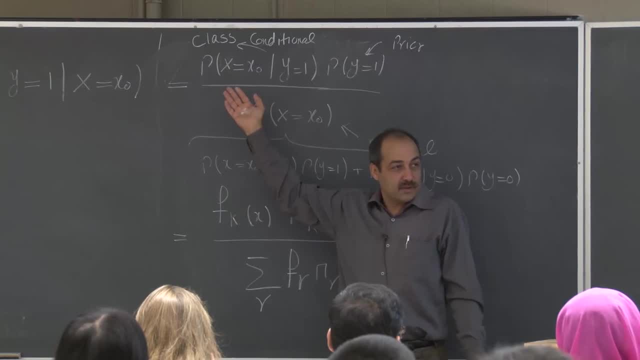 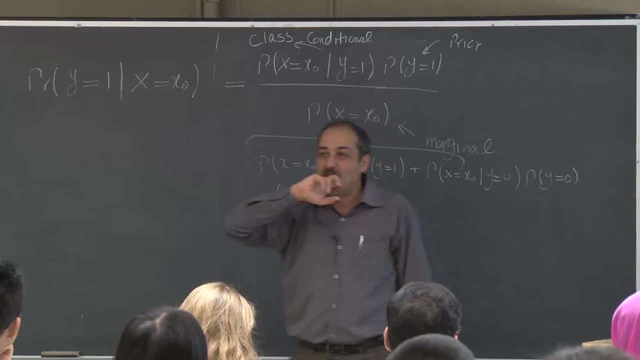 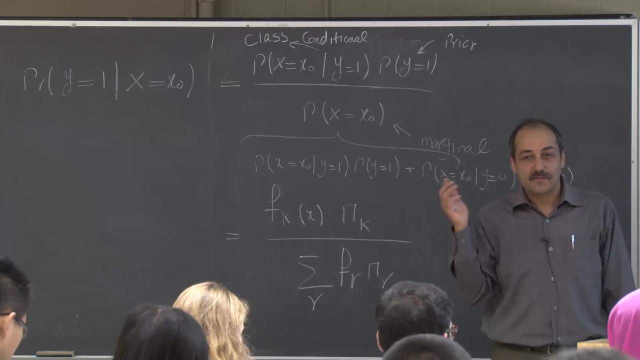 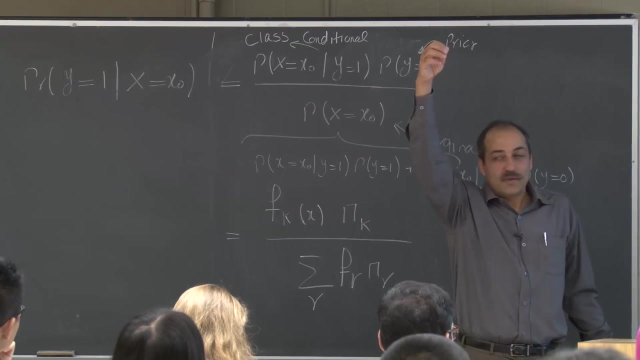 different reason, because density estimation techniques are usually are usually are not good techniques, especially when you are in high dimensional space. you know, in high dimensional space, no way that you can. you know you have images, this like resolution of six megabytes. you know how many pixels do you have. your vectors are of the order of millions and you 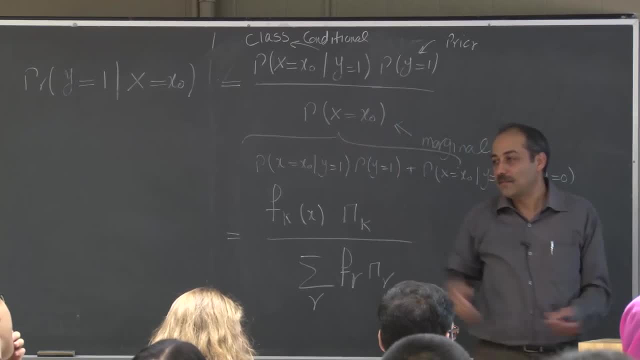 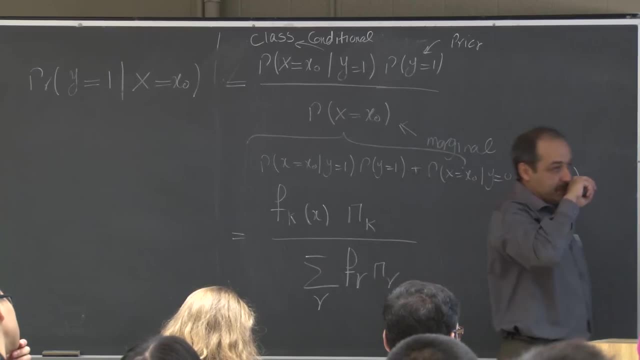 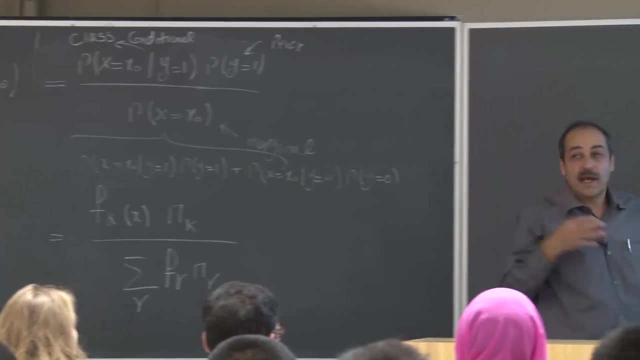 want to estimate the distribution in this high dimensional space. no way that you can get it correct. so, because there is no good way to estimate this distributions, this density, so there are different approaches to classification that in this course we are going to see some techniques in any of these. 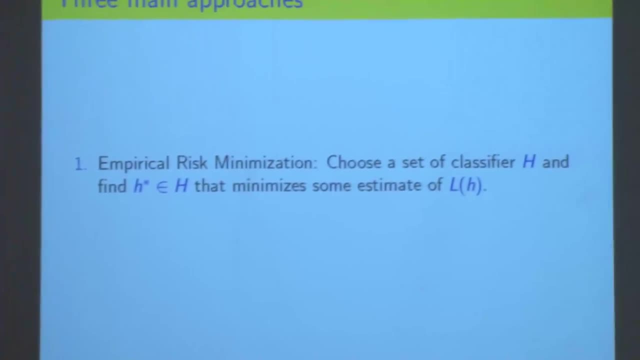 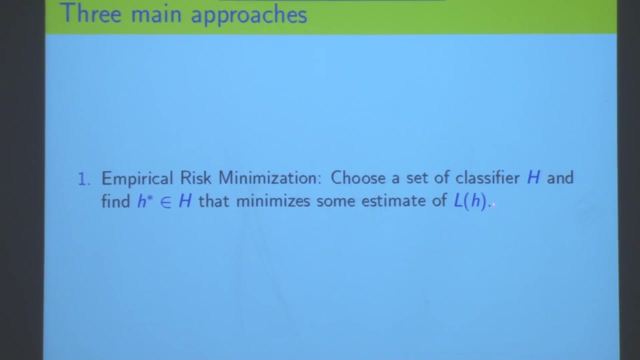 approaches. so is one approach. So one approach is empirical risk minimization. So in this approach we choose a set of classifier H, capital H, and we find one member of this set that minimize some estimation of the error rate. Okay, so what does it mean It? 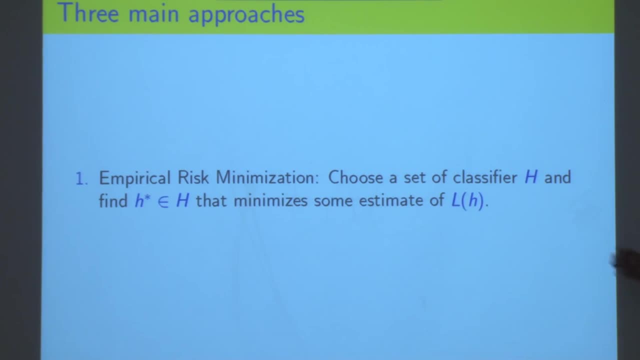 means that I'm going to assume that my classifier comes from a class. You have to make this assumption all the time. There is a term in machine learning: no lunch, no free lunch term. There is no free lunch. It means that no assumptions, no learning. So if someone tells you that without making any 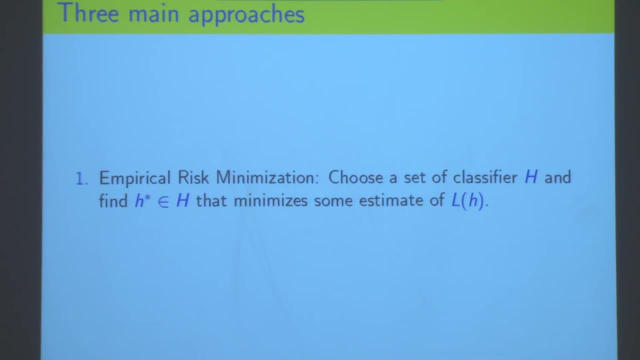 assumption, without any prior, we can elegant something from this data. don't believe it, you know, because you, mathematically you can prove that it's not possible. you need to make assumption. so I give you data for classification. you have to make assumption about the data. so my 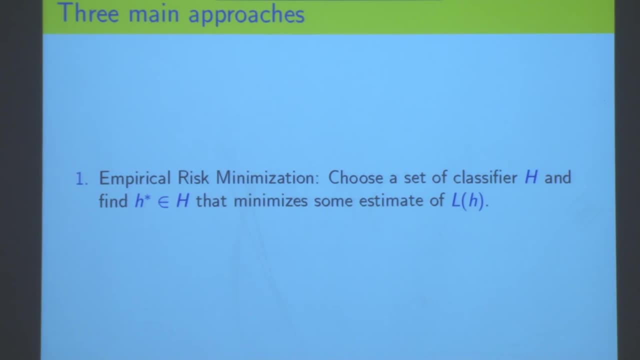 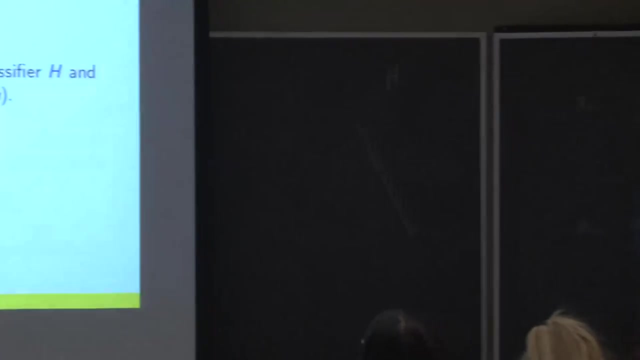 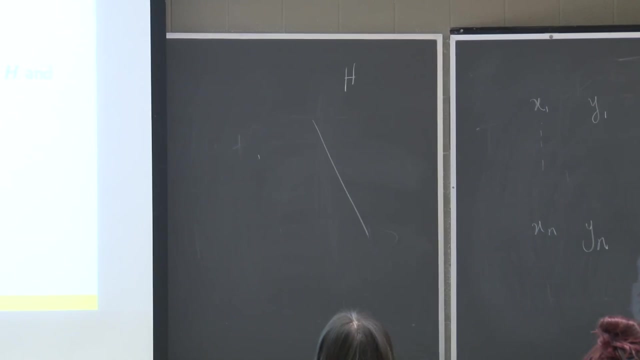 assumption is that there is a linear classifier. here means that my assumption is that a line can separate these two set of class. then I can in in the capital set of all lines or all half a space. I can choose the one which minimized the true error rate. I can assume that my classifier can be: 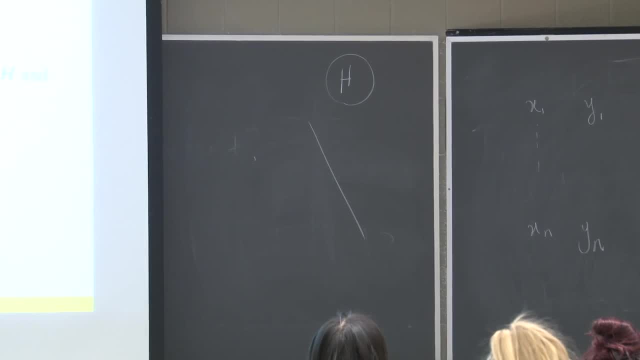 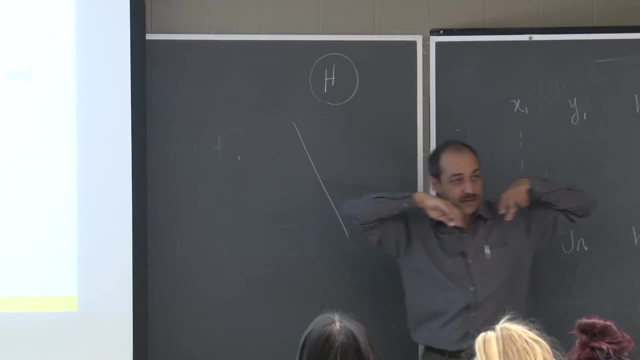 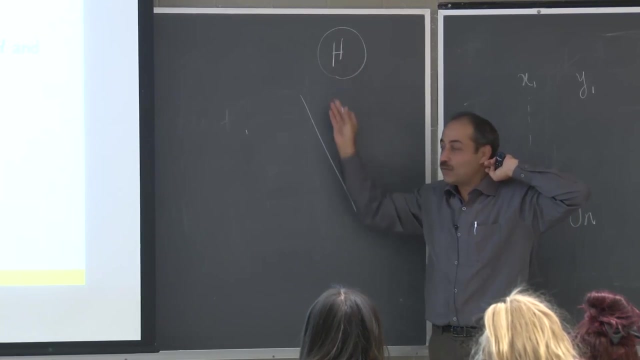 represented by neural network. then among all neural networks that has this type of structures- you know three nodes in the first layer, ten nodes in the second layer, and so on- I will choose, I will search for the one which minimizes the error rate. so that's one approach to. 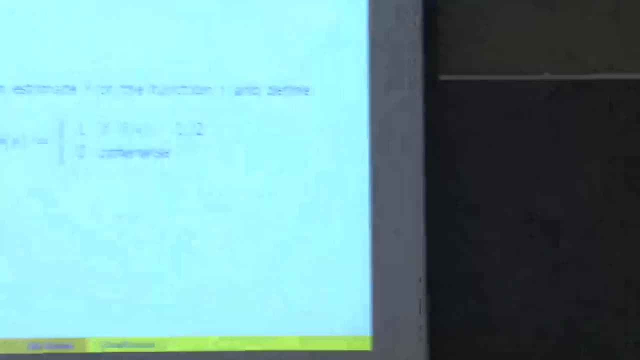 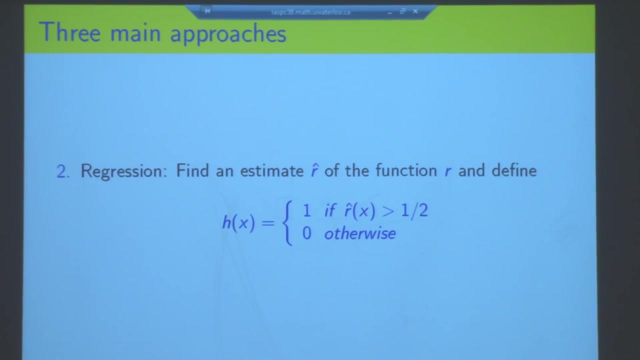 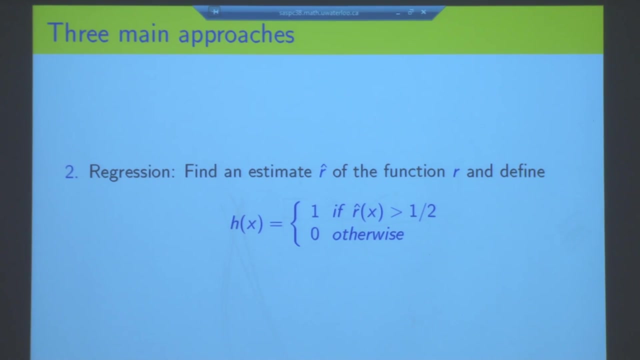 classification. so another approach which could be in some cases have overlapped with the first approach is regression approaches. you know, I told you the difference between regression and classification. you know, in classification we have this type of data points: y comes from a finite set. in regression, you 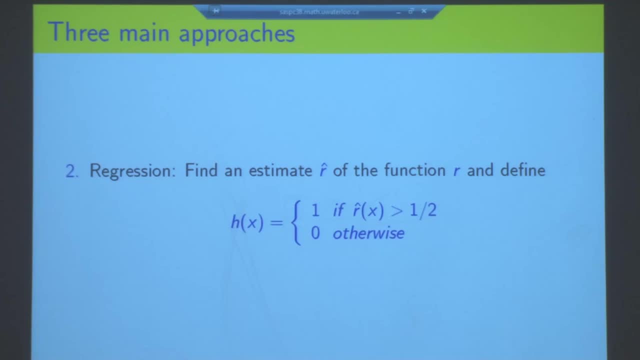 relax this assumption that y comes from a finite set. y could be real value. you know, that's the difference between classification and regression. so regression is easier problem because you don't have this additional condition and y and there are methods to solve this problem. so it's hard to. sometimes it's 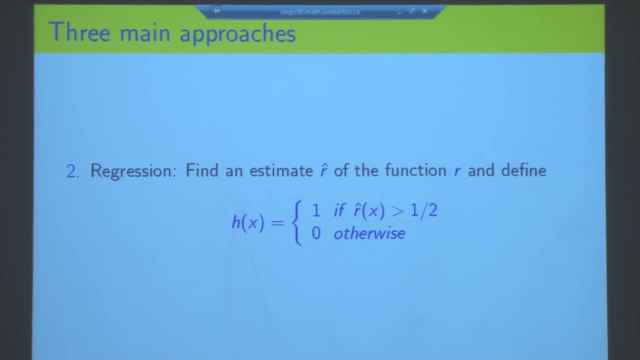 hard to calculate a function H to map a vector to only two distinct labels, either zero, I mean the output of this function should be either 0 or 1. sometimes it's hard to do that, but it's easier to estimate a function which map my, my. 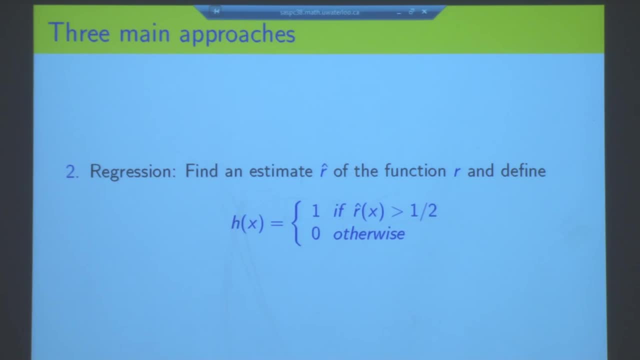 vectors to a real value, say between 0 and 1. but this is not classification anymore, it's the regression. but that's fine, I solve the problem using regression methods. then I put a threshold here. so my function maps everything between 0 and 1, but I 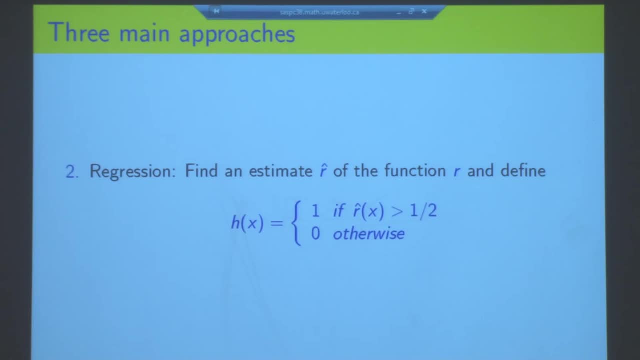 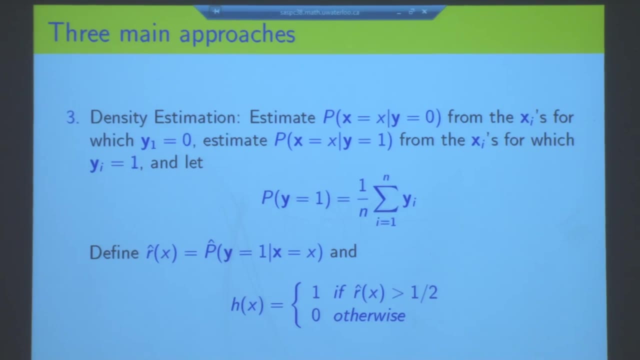 decide. if it's more than half, I would decide that it's one. if it's less than half, I decided to zeal. that's another approach. and the third approach is the one that I just mentioned, that you can do density estimation. you know, I can estimate this density for class 0. I can estimate the density for class 1, I can. 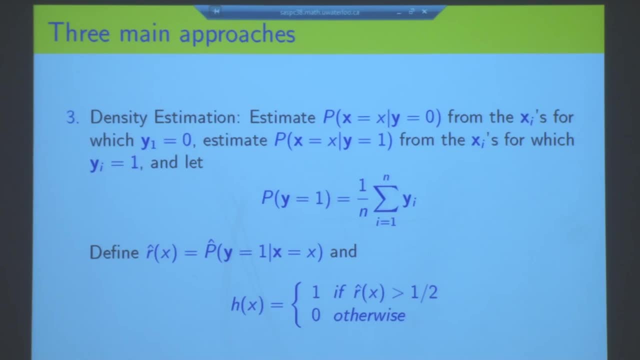 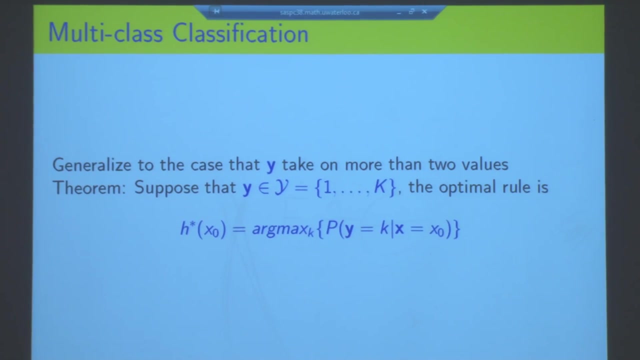 estimate priors and then I can do basal for classification. okay, so the first real classifier that we are going to learn is actually based on this third approach. but before I go through the details of this classifier, let me just tell you that easily you can extend this technique to multi-class problem. so 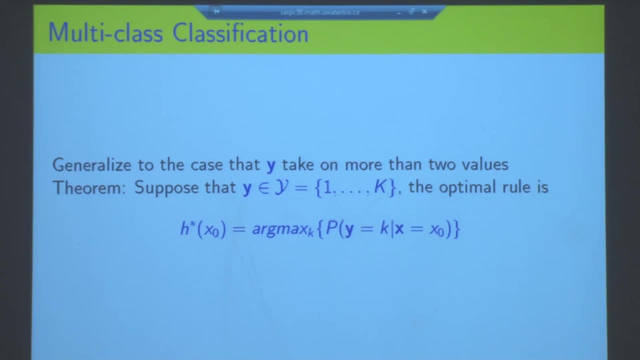 I all of the examples that I gave you for was for two classes, for multi-class problem. if you have K classes you can compute P? Y for each class for class one, two, three, four, up to K and go for the one I mean label according to the 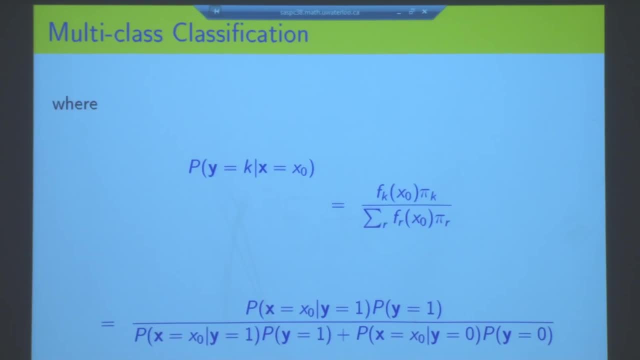 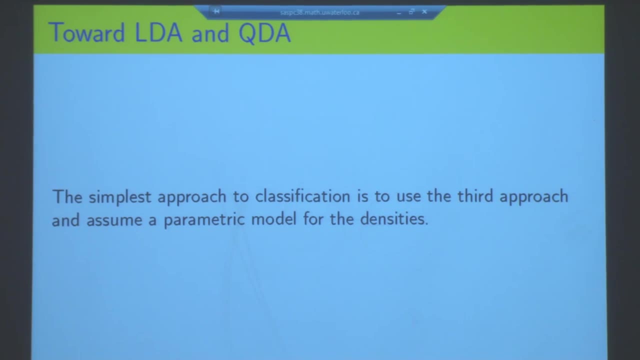 maximum value, go for the one which has maximum probability, okay, okay, we are going to use the third approach- means density estimation- and learn the details of our first classifier. this first classifier is called LDA- linear discriminant analysis. okay, so let's see how linear discriminant analysis works. 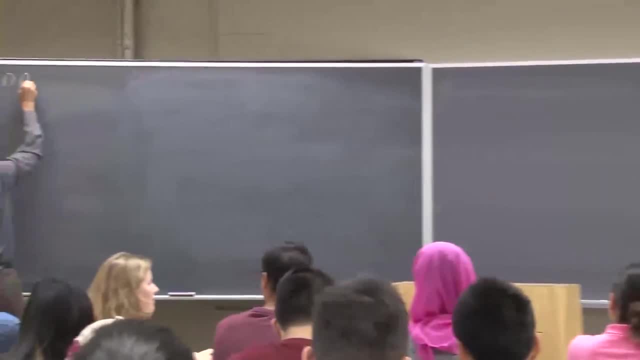 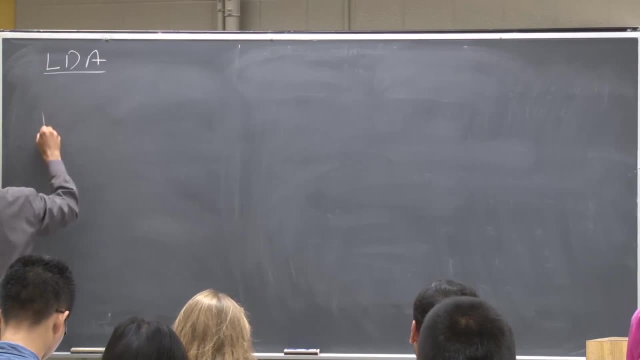 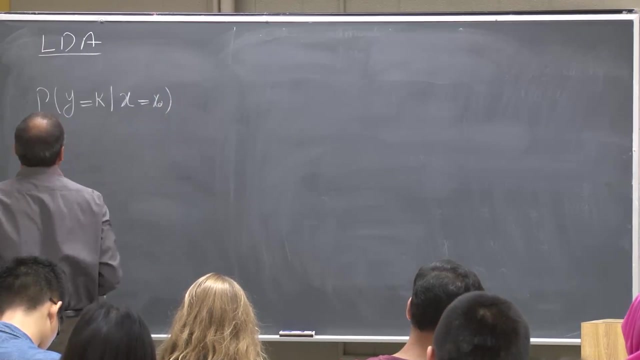 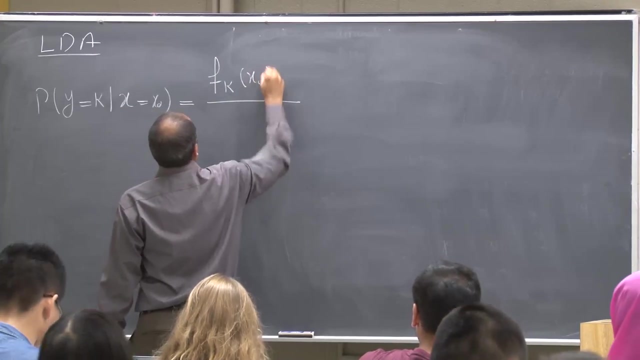 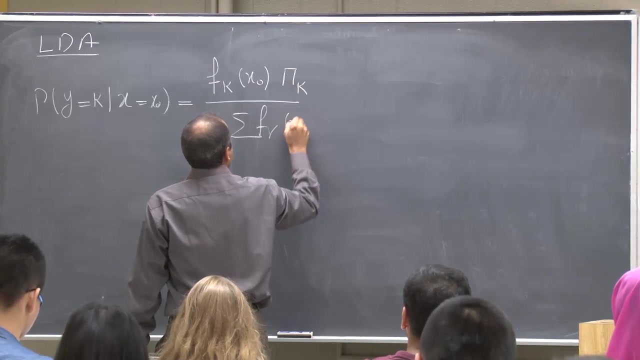 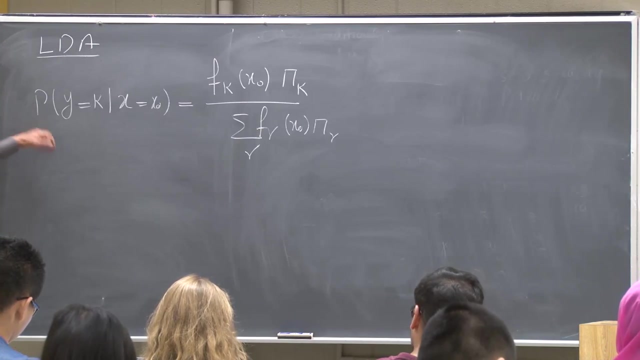 okay, linear discriminant analysis. we just learned that. you know I can compute this as balance L, DA. uh, one D for order, both. I can google that so I can see that this formula is based on. I can compare value to environment and counter so I can apply Bayes rule, compute this posterior and go for the class which has larger posterior probability. so let's assume that we have two class problems for simplicity. then we can see how it can be extended to multi-class L, DA. I'm talking about LD. so I assume that we have two class problems for simplicity. then we can see how it can be extended to multi-class L, VA. I'm talking about LD, so I assume that. 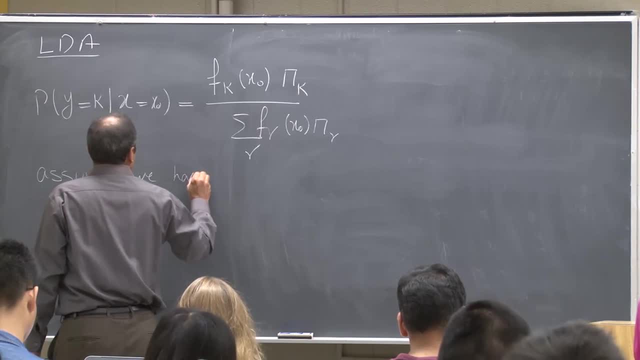 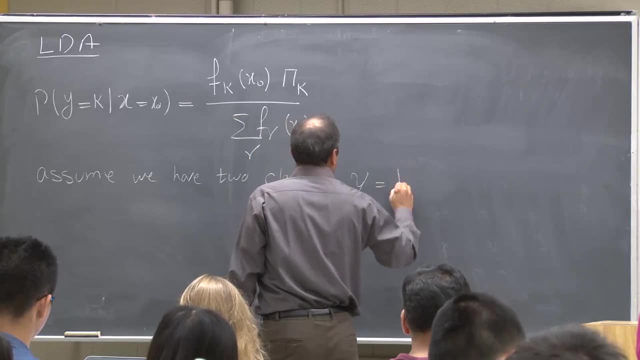 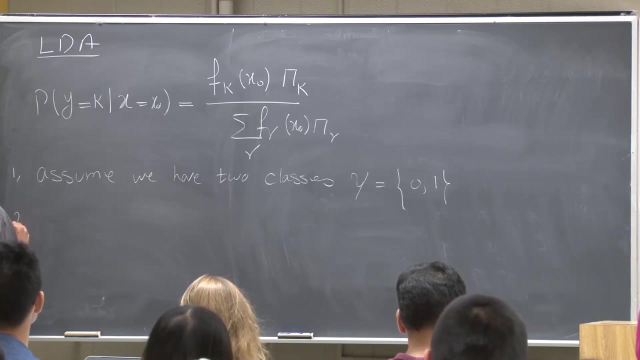 you can apply base rule, compute the one properties of摩, Neymar, jeux and Anil's societies over three classroom to multiple class, L DAvy, teachers of PYs, Sinovac and other people like special classes. we have two classes, so it means that Y comes from this set. so then I make 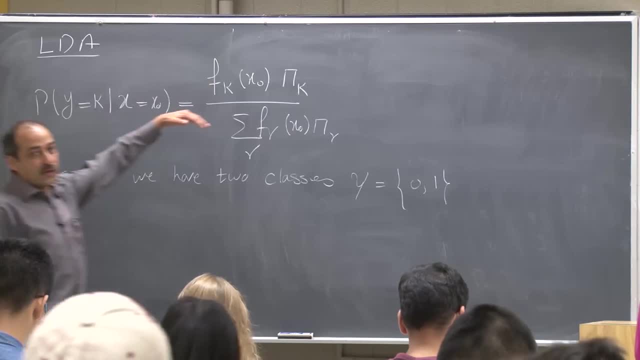 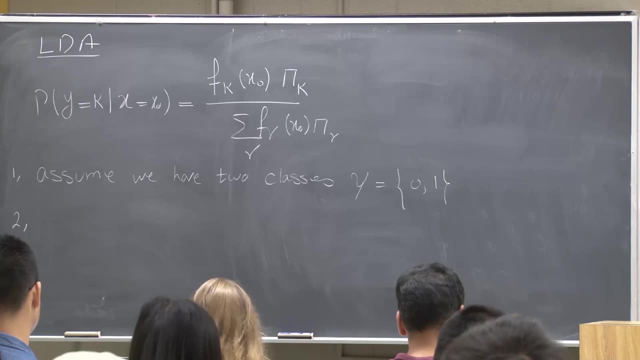 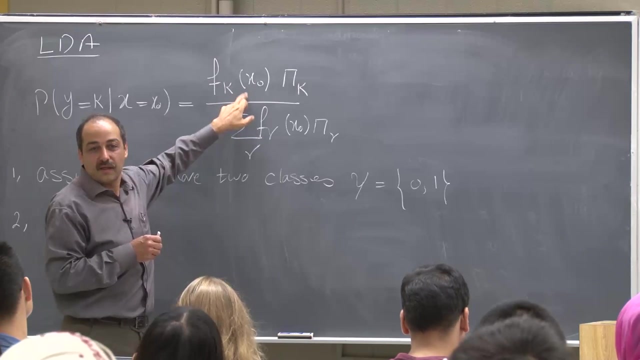 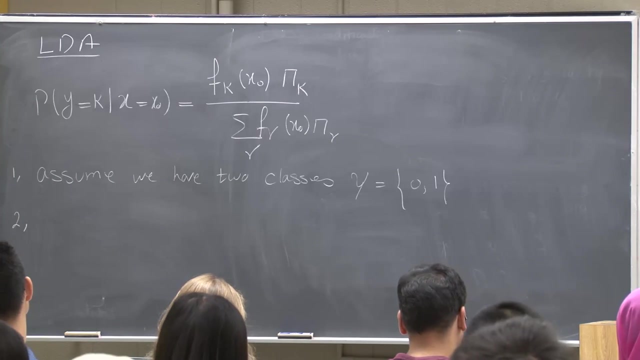 another assumption. so I would like to go for the third approach for density estimation. okay, for density estimation I can just look at the data, try one of the general density estimation techniques to estimate this density, or I can assume a parametric form for this density and then go find the parameters from data. so 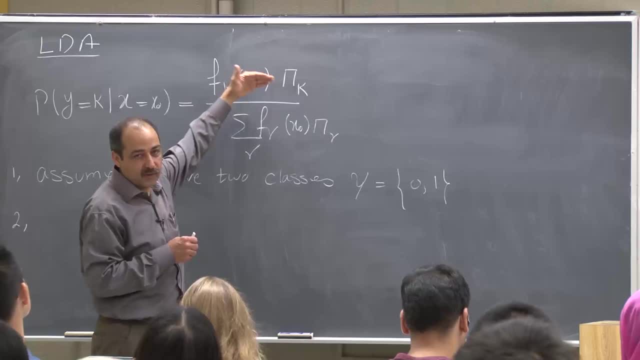 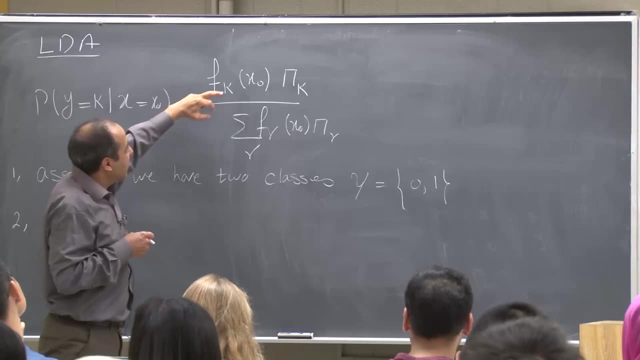 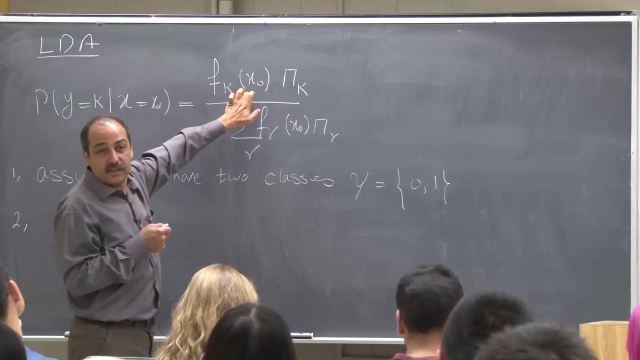 I can assume this is uniform, this Gaussian, this is whatever, and then look at the data and compute the parameters further. so in LDA, our assumption is that class conditional distribution is Gaussian. so Gaussian is one of the easiest distribution that you can work with. okay, so my assumption is that this is Gaussian. so this is my second. 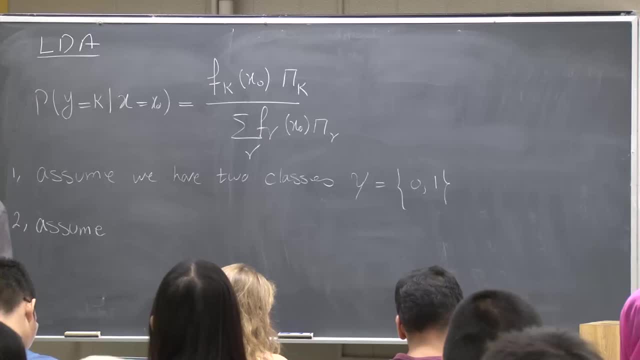 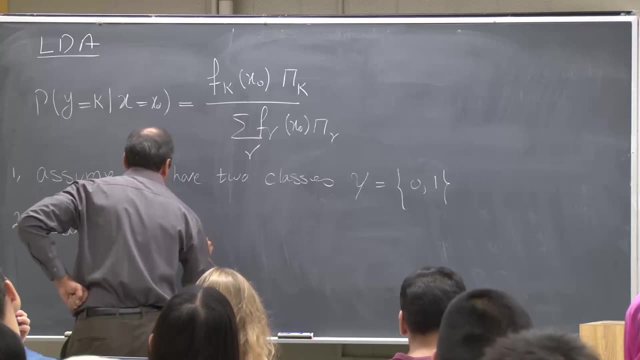 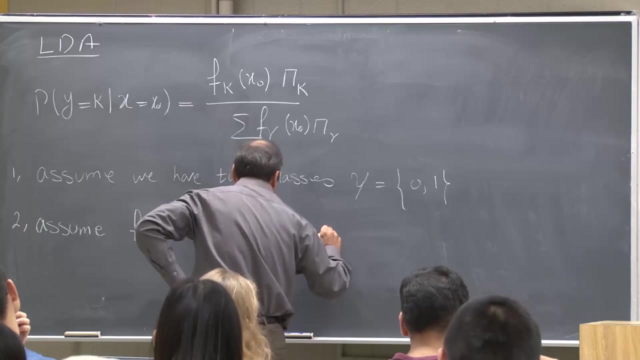 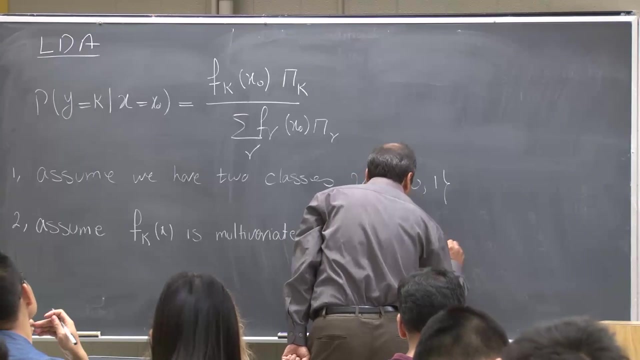 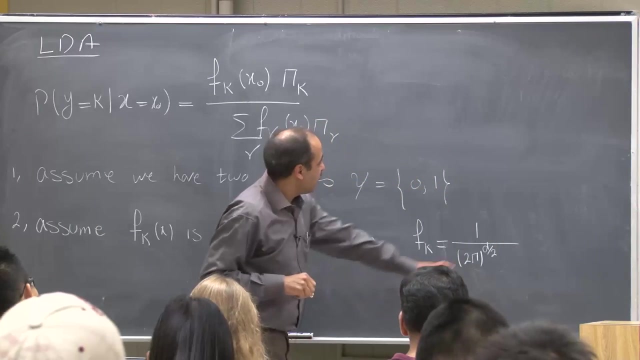 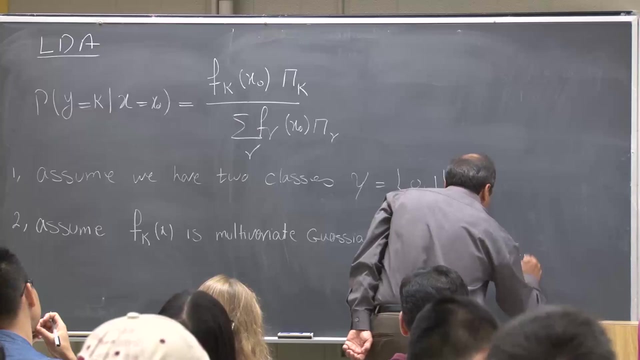 assumption in LDA. so assume fk is multivariate Gaussian. being multivariate Gaussian means that fk is 1 over 2, pi to the power of d. this pi is not the prior, it's three point fourteen, you know. and sigma, which is my covariance to the power of 1, half e to the power of minus. 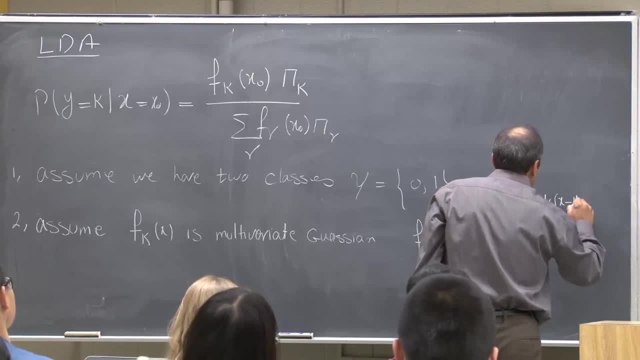 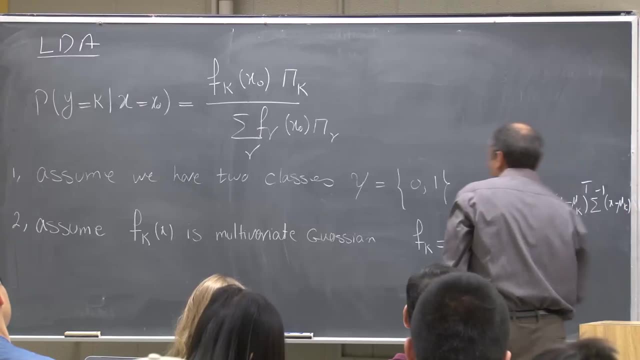 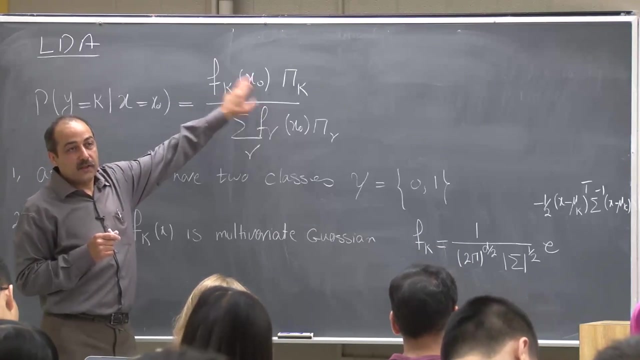 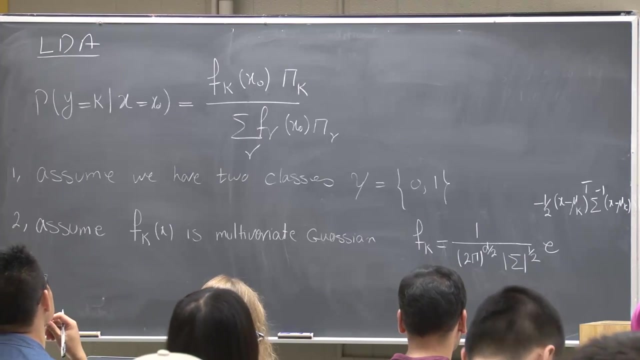 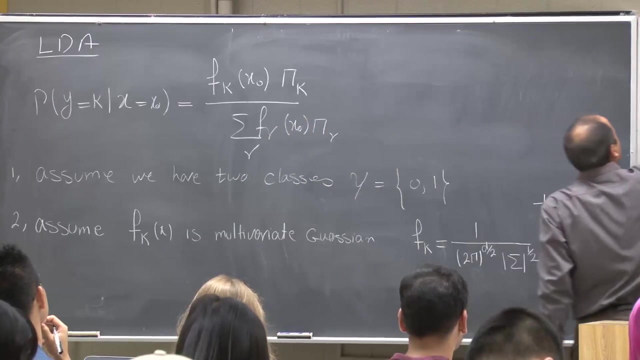 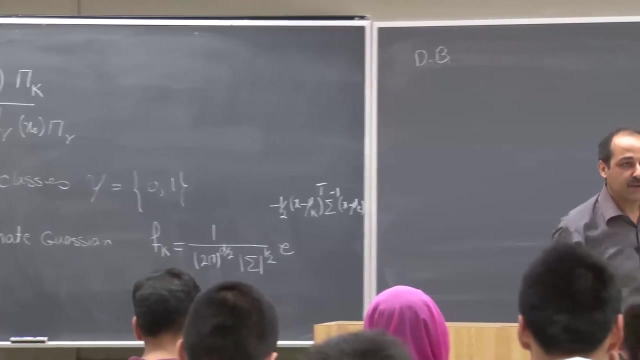 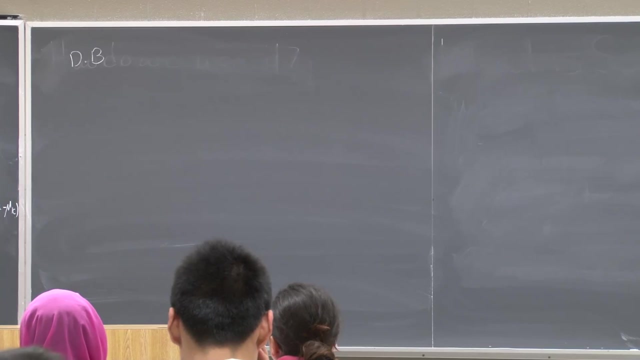 one half X minus mu K. Sigma inverse is transposed: X minus mu K, that's multivariate Gaussian. so that's my second assumption that my conditional distribution here is Gaussian Jamir. okay, what would be my decision boundary? so what was the definition of decision boundary? decision boundary was set of points such that probability of being in 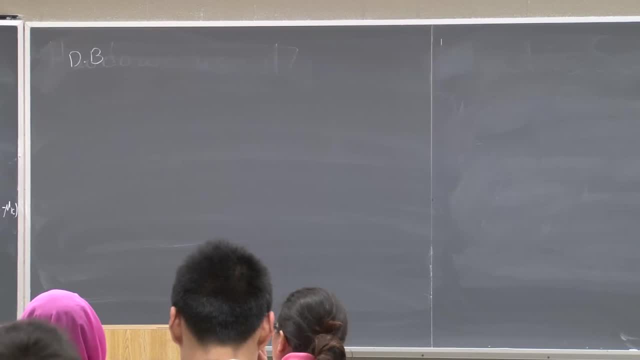 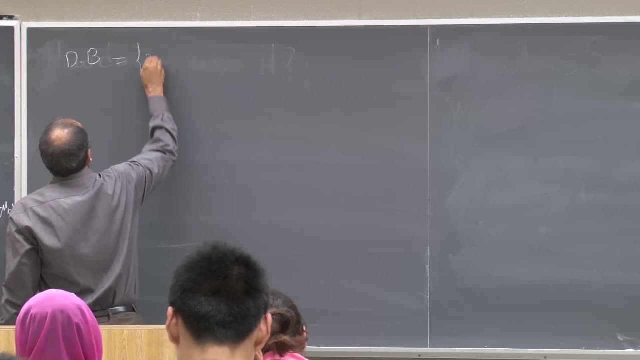 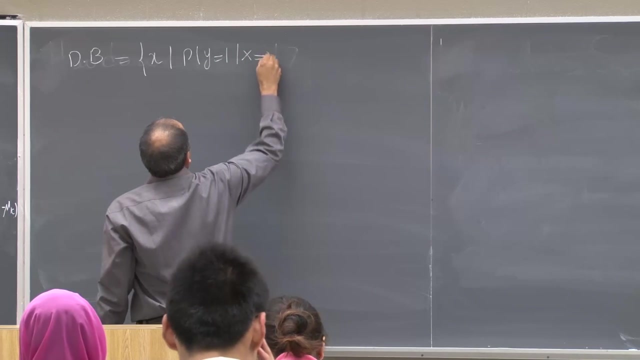 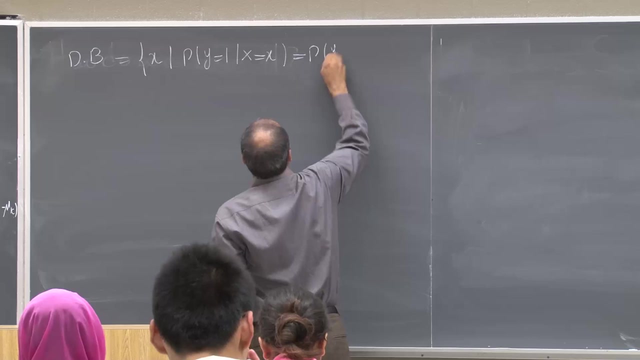 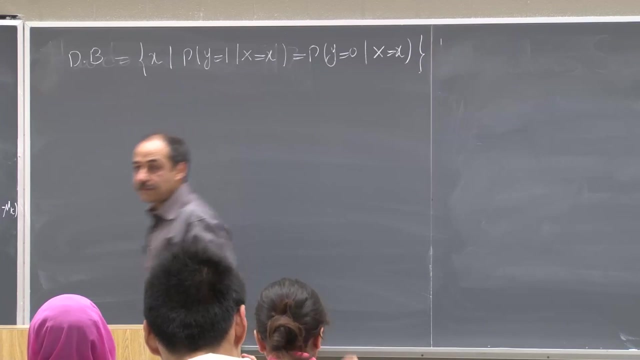 one class is the same as Sedro to have being on the other class, right? so decision boundary is not chopped in half. and this assignment- how did I get this? the set of points such that probability of being in class 1 is the same as probability of being in class 0. So I would like to compute the decision. 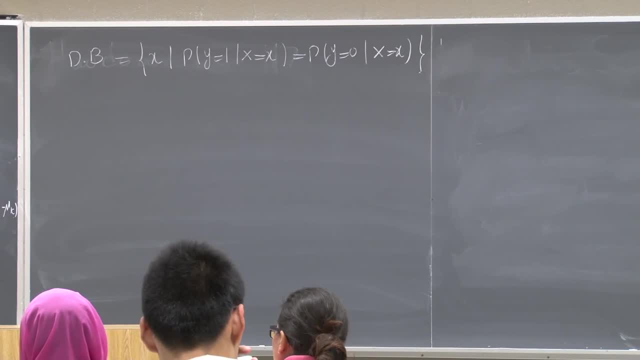 boundary. You know, based on the assumption that my class conditional is Gaussian, I would like to geometrically know what are the set of points such that the probability of both classes are the same, Means if I'm on one side of this boundary, I have more probability. if I'm on the other side, I 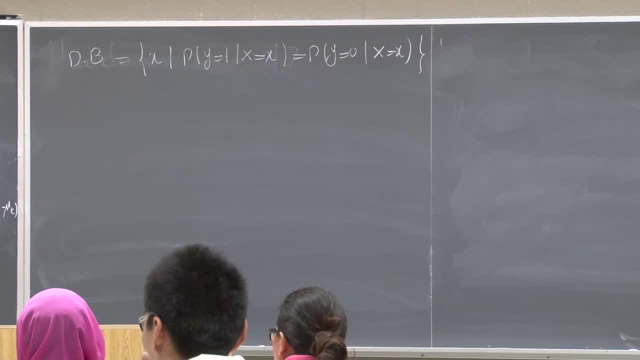 have less probability. Okay, is that clear? Okay, so basically I need to solve for p y equal to 1, given x equal p y equal to 0, given x. I need to solve for this, Okay. so p y being 1 given x is basically f 1 x, pi 1. 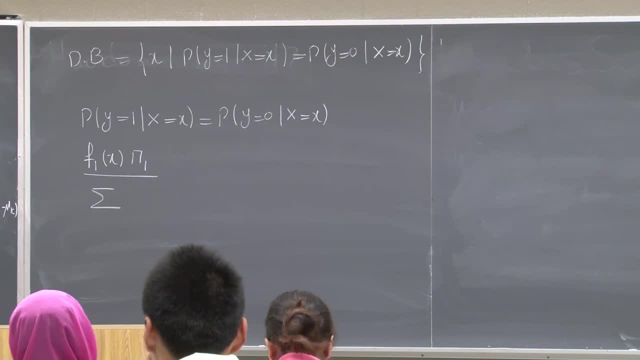 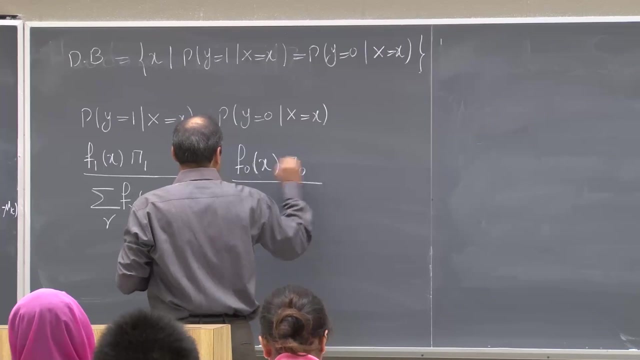 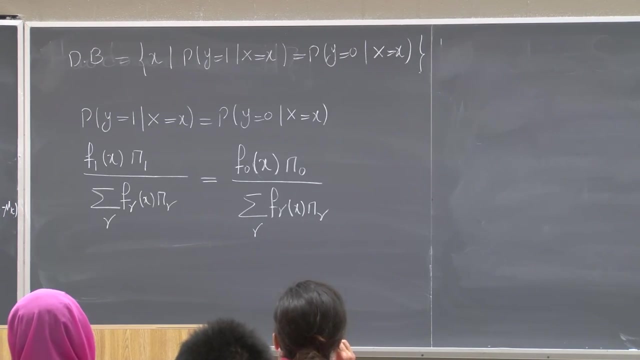 divided by marginal, This should be equal to being in class 0.. f null x pi null divided by marginal. Okay, happy so far. So this marginal is the same right, So I can cancel the marginal. So what I need to solve is f 1x pi 1 equal to f null x pi 0. 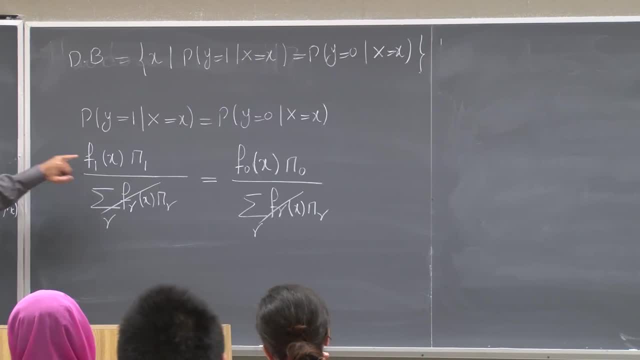 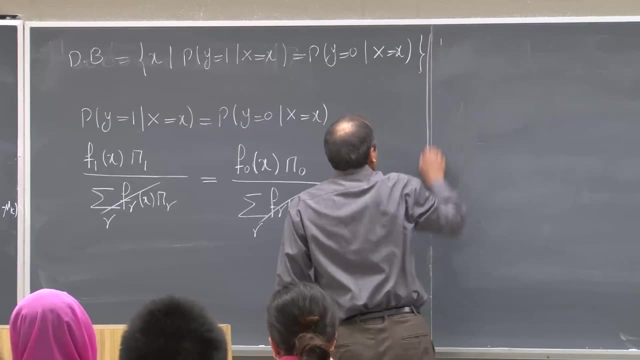 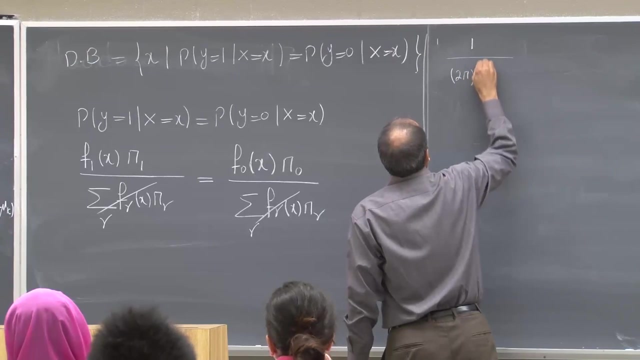 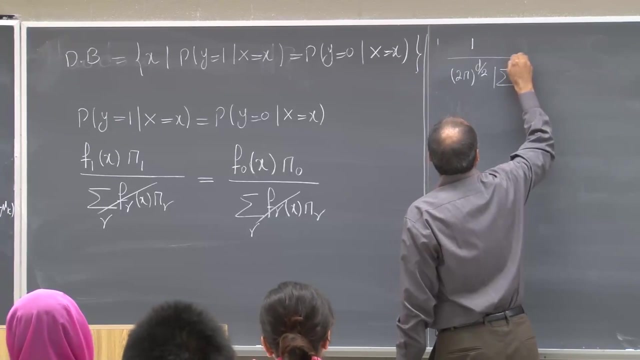 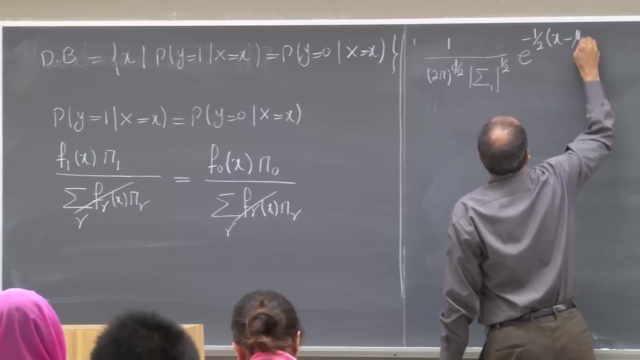 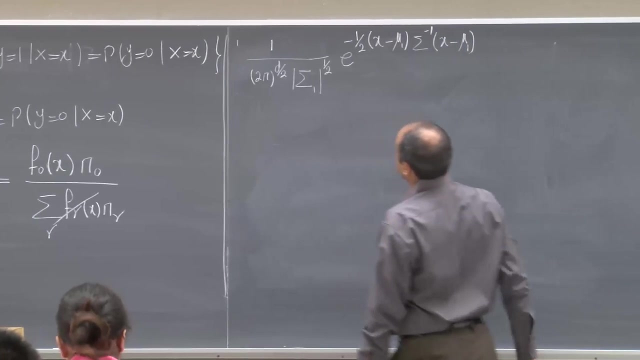 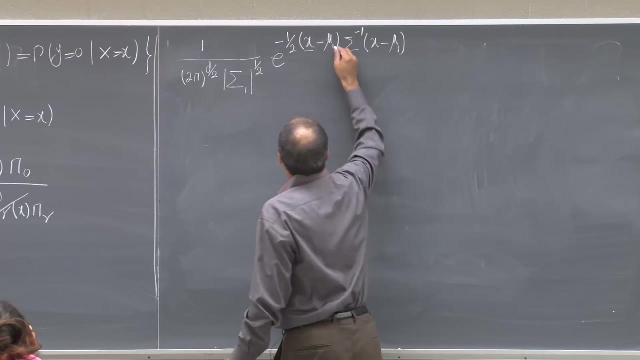 But f? I assume that f is Gaussian And I Okay. So basically I need to solve for this equation: 1 over 2, pi, d over 2, covariance matrix of class 1.. And this x is a vector, d-dimensional vector, And this mu is: 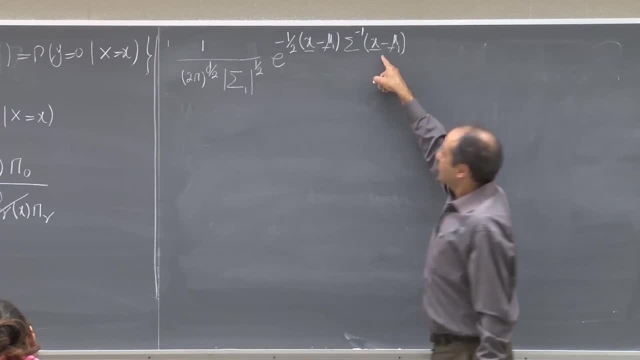 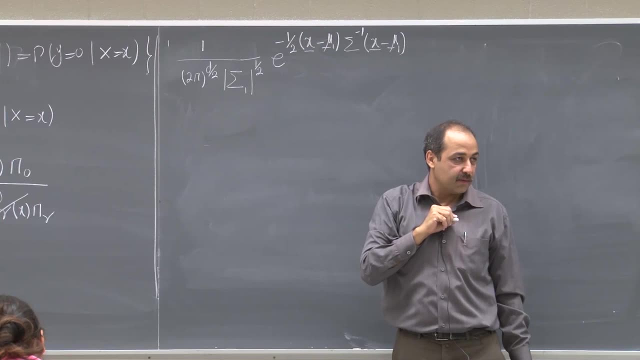 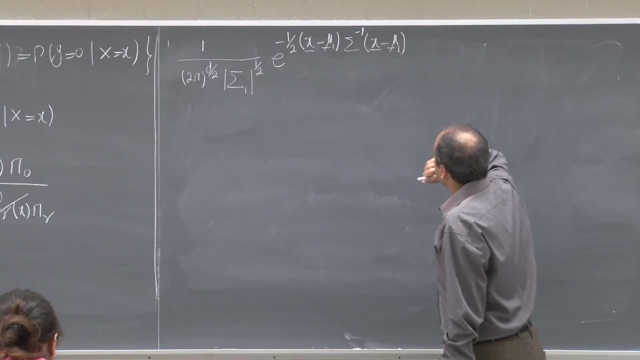 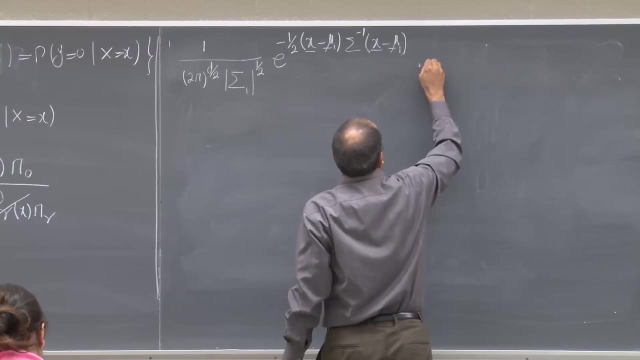 also d-dimensional. you know, That's my notation for vector In slides. you know it's bold. When it's bold it means it's a vector. Okay, So that's f1 x times pi 1.. We haven't estimated pi 1 now, Let's just assume that we know. 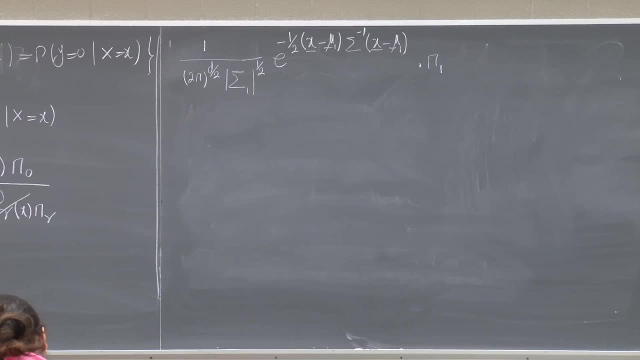 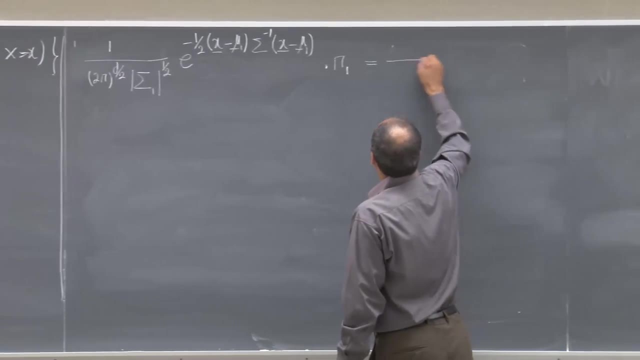 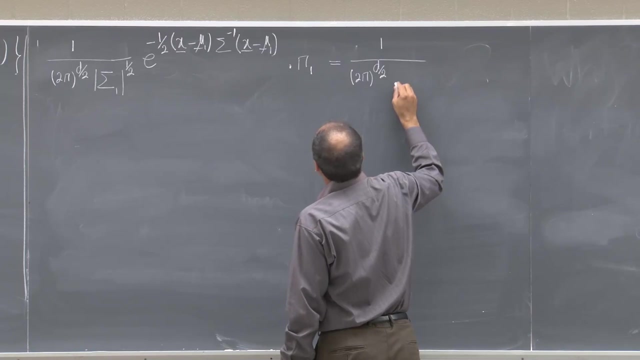 It's a scalar. you know it's a value. Let's assume that I have it. I have something. I believe that what's the chance of being in class 1.. This should be equal to 1 over 2 pi times sigma of class 0.. 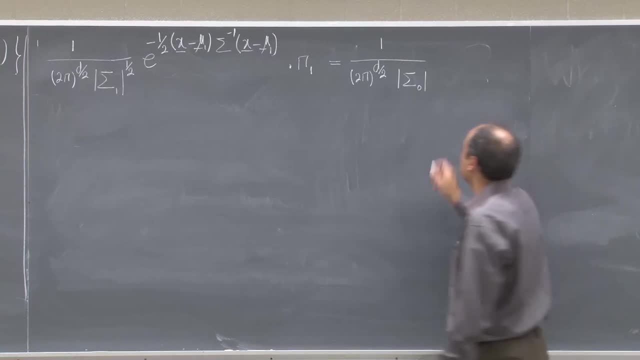 You know, covariance matrix of class 0.. 1 half e to the power of minus 1 half. x minus mu 0.. Sigma, Sigma 0. Sorry, Minus 1.. x minus mu 0.. This is a transpose. 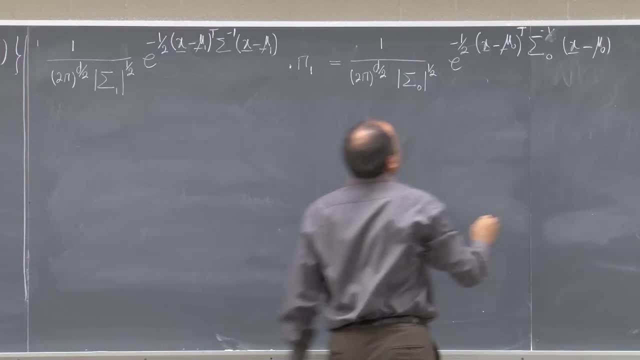 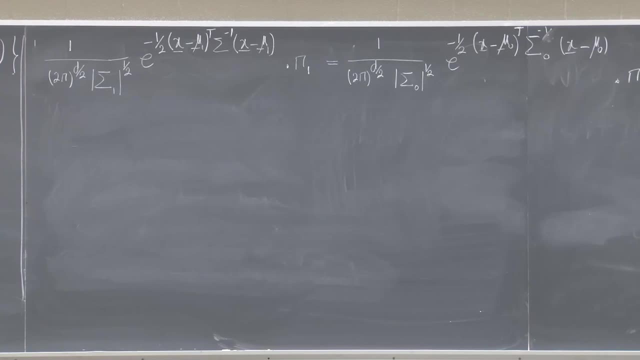 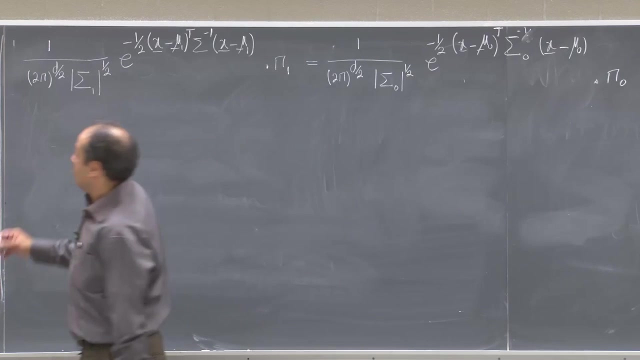 I need a transpose here. Okay, Times pz. So I need to solve for this now. Okay, For simplicity, I make this my third assumption. So so far I want to do Bayes classifier. I had two assumptions so far. 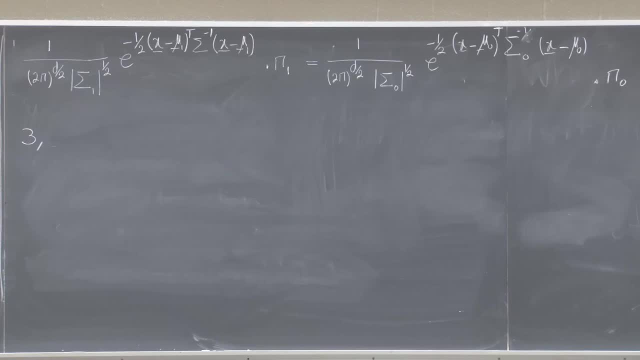 First, I assume that I have two classes. Then I assume that my class conditional distribution is multivariate Gaussian. Now I make my third assumption. And my third assumption is that covariance matrix of class one is the same as covariance matrix of class two. 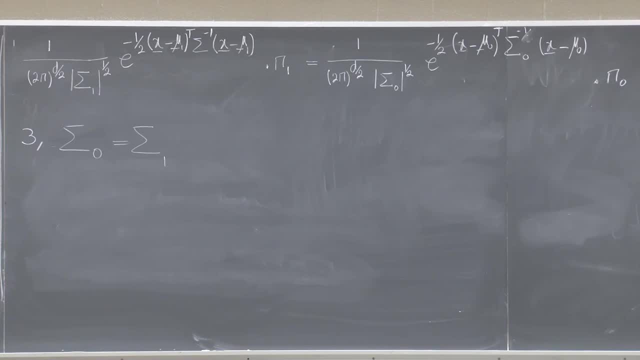 Sorry, Just for simplicity. You know, that's how. that's how our modeling works. right? Word seems to be complicated. We can't understand it. Let's make assumption: Images are Gaussian. No, I'm just going to assume that they are Gaussian. 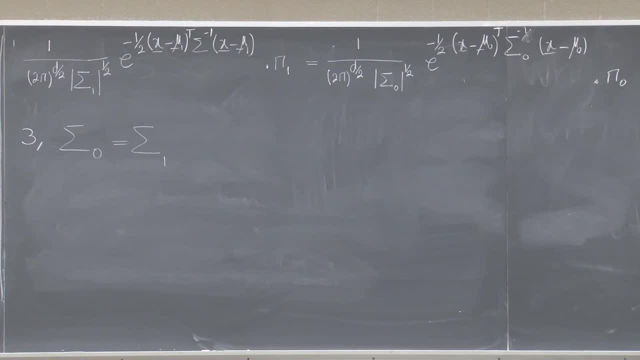 Okay, Coherence matrices are the same. No, I'm just going to assume that they are. Why? Because I can't do better than this I can't solve. So let's make some assumption in order to be able to solve the problem. 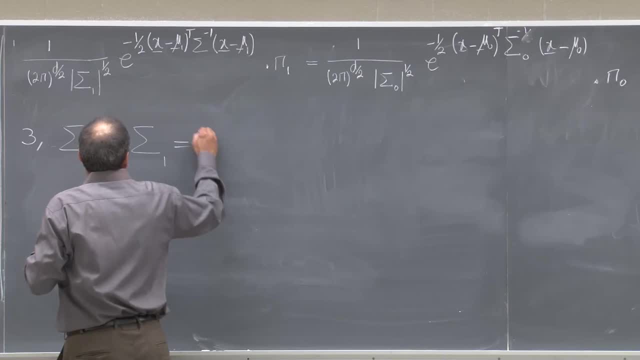 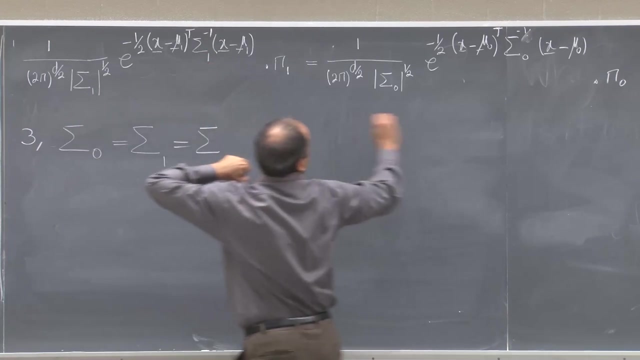 Okay, So that's just my assumption that they are the same, So I will call them sigma. In practice they are not the same, Okay, So if I make this assumption, then basically here this: you know, that was sigma one, actually. 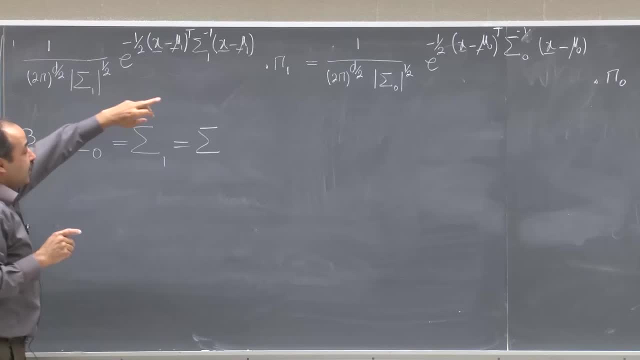 and that was sigma zero. If I make this assumption, I don't want to repeat this formula again. So this is going to be sigma, right, And this is going to be sigma, and this is going to be sigma and this is going to be sigma. 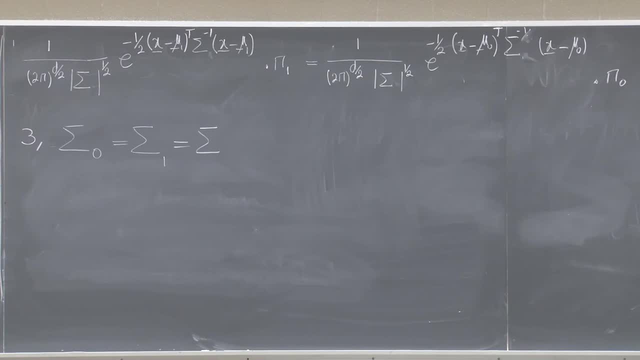 because of the assumption that I made. Okay, so denominator here on the left-hand side is the same as this denominator on the right-hand side after this assumption, so I can cancel. Okay, now I have to solve for this And to solve for this. 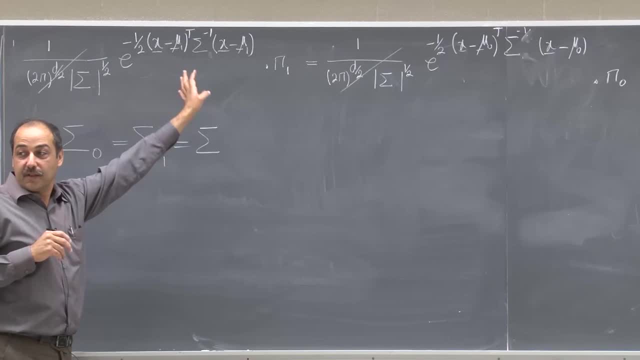 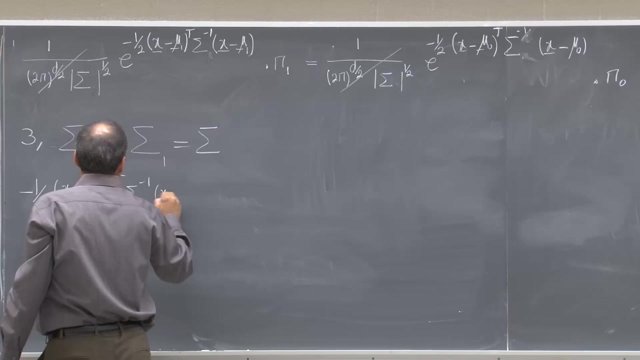 let me take log from both sides to get rid of this exponent. So on the left-hand side I have one-half x minus mu one. transpose sigma inverse x minus mu one. So plus Okay, Plus log pi one is equal to minus one-half x minus mu null. 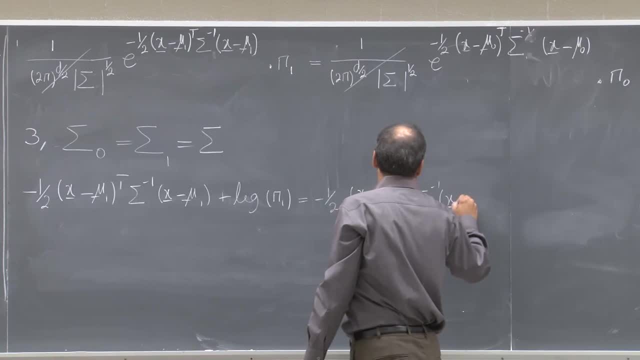 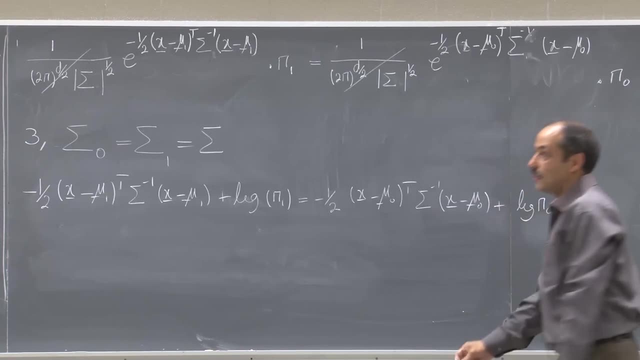 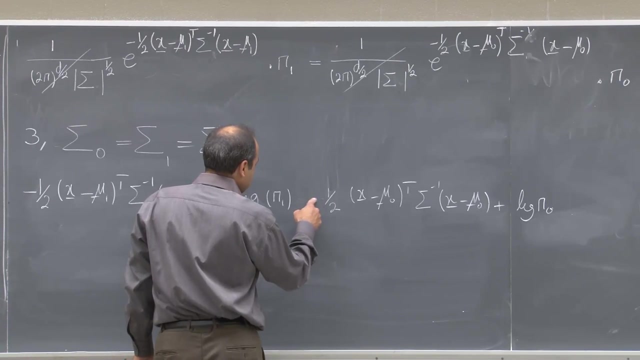 transpose: sigma inverse x minus mu, null plus log pi z. Okay, Okay, So I can take everything to one side. So that's going to be plus, That's going to be minus equal to z. Okay, now let me expand this. 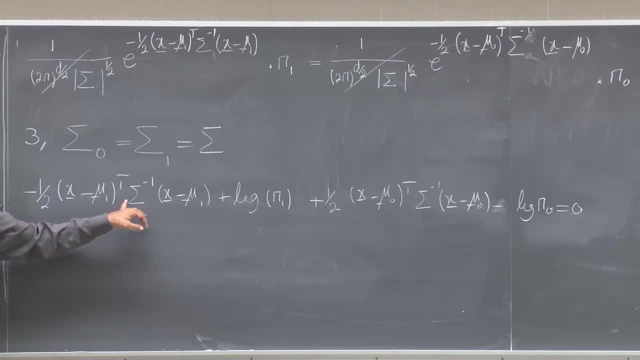 This is just quadratic form, right? If I expand this quadratic form, what do I have? I have Like this: the first term is squared, I have the second term is squared and they have minus two times first term. second, It's quadratic form. So I'm how. I'm going to have minus one half. 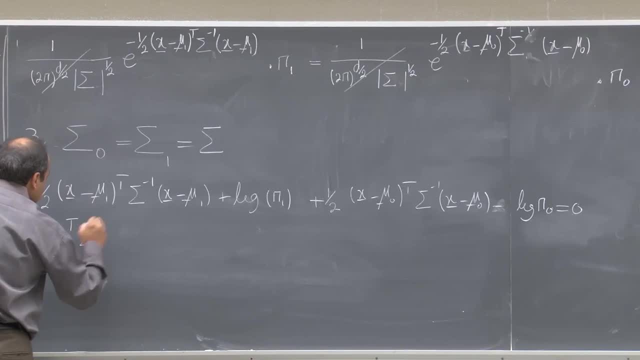 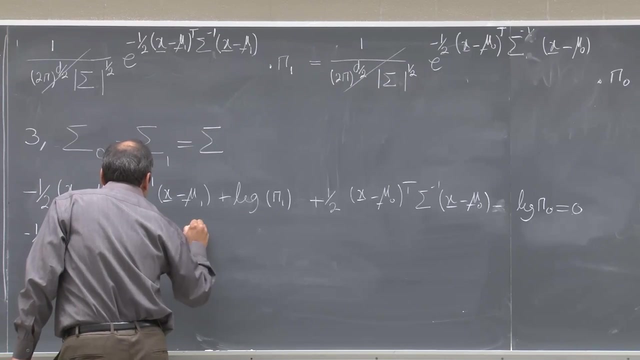 X transpose sigma inverse X. That's first term is squared Right. I have second term is squared, Which is mu 1 transpose Sigma inverse mu 1. they have minus half here, so it's going to be minus half mu 1 squared Sigma inverse mu 1. 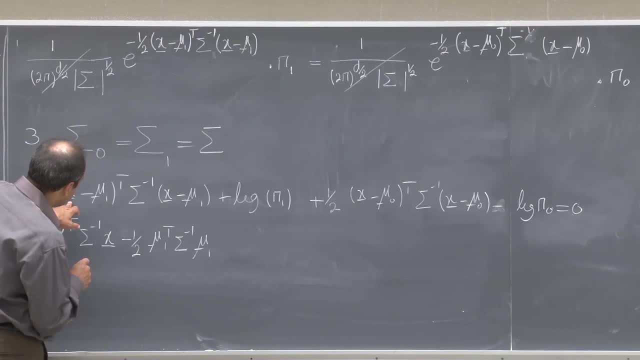 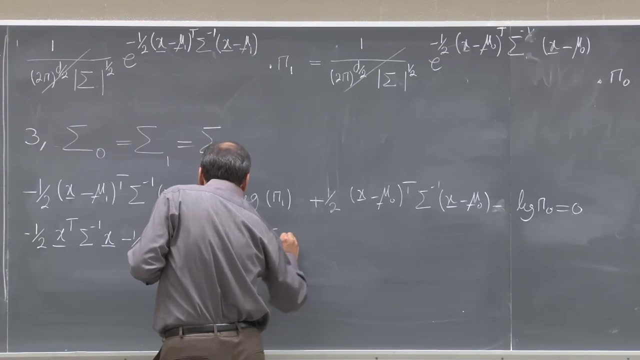 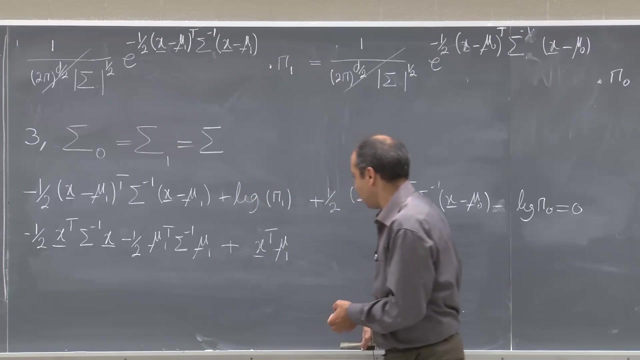 And then I have This- I'm in two times this term, this There, which is going to be Negative 2. you know, X transpose mu 1, and Then it will multiply it by negative 1 half, so it's going to be just Plus X transpose mu 1, am I right? 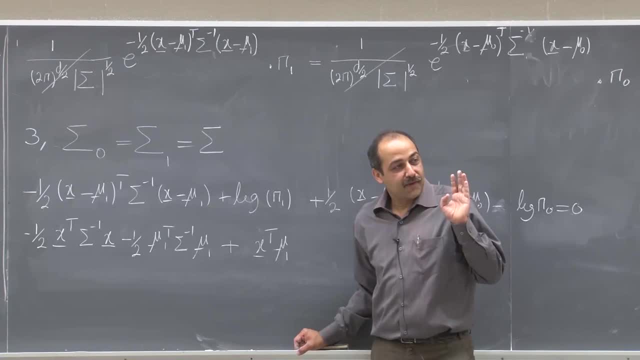 Let me warn you In the first from first lecture: be careful. I tend to make many numerical mistakes on the board, so Be aware, sorry, yes, Sigma. Okay, so that's expansion of this quadratic form, right, No, No, Sorry, No, No, we have it here, Yeah. 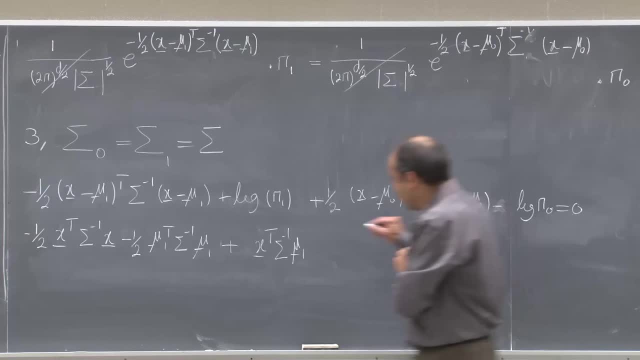 We have it here, Okay, Okay, Okay. Okay, let's expand this one As well. So I have One half X- transpose Sigma inverse X. That's for this term. I have minus one half. Oh, sorry, I have plus Mu Null- transpose Sigma inverse Mu Null, And I have 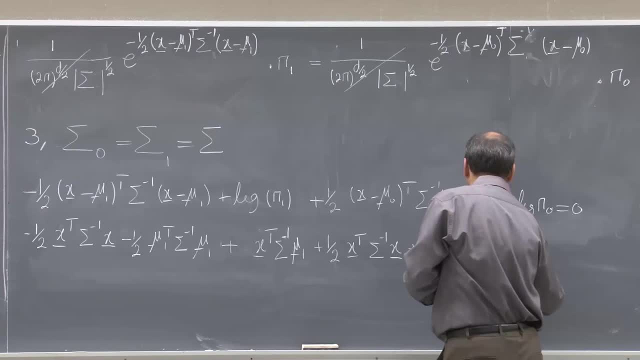 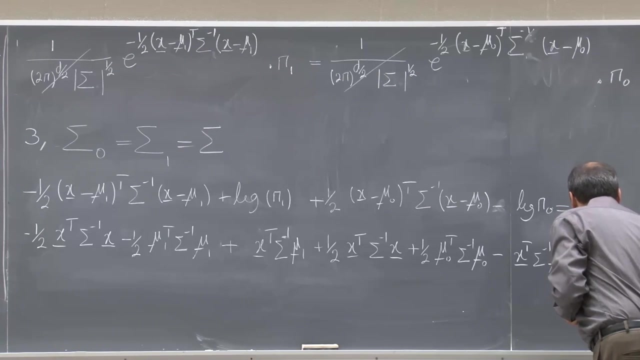 Minus Ah X transpose, Sigma inverse mu null and I have minus X transpose. So that was for this term and this term. then I have log Pi 1 and I have minus log Pi 0, so I'm going to write it as log Pi 1 divided by Pi 0, equal to 0. 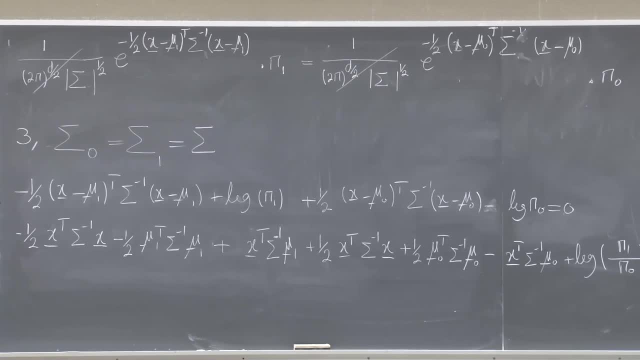 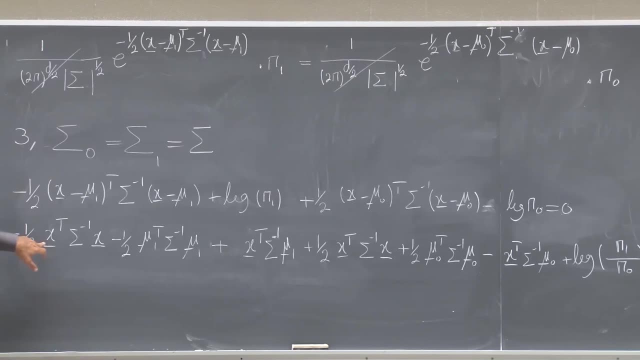 Okay, Okay, Okay. So we can do a little bit of simplification here. So we can do a little bit of simplification here. You know, I have negative one half X- transpose Sigma inverse X here, And I have positive one half X transpose Sigma inverse X here, So I can cancel. 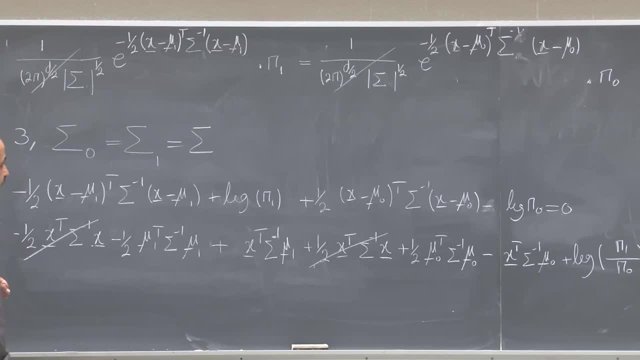 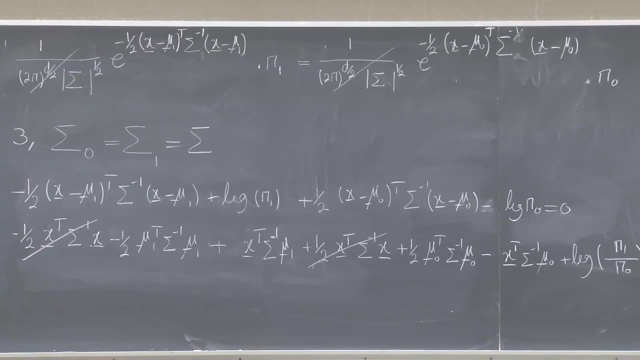 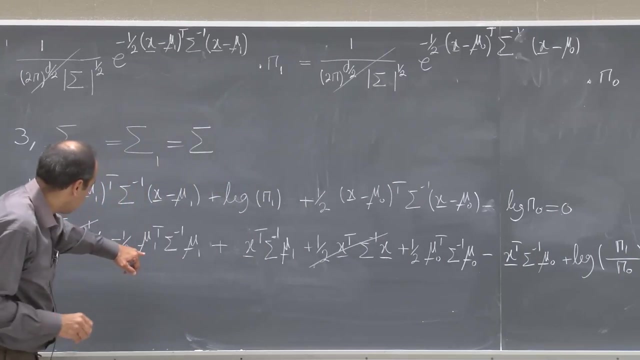 This two term, This two term, Then Then, So, So, after cancelling this two term, Then Then You know, I have this term: Mu 1, transpose sigma inverse. mu 1, Which is just And a scalar Which has nothing to do with X, so it's constant, It does not depend on X. 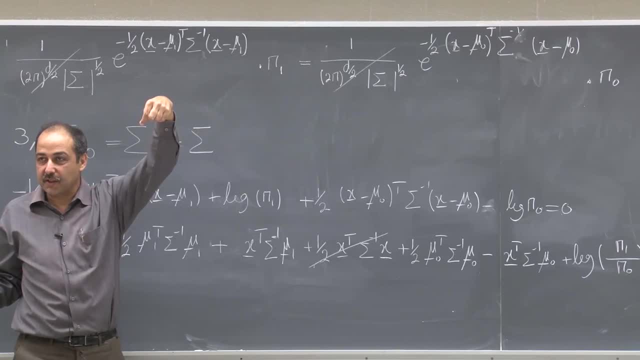 And it's a scalar because mu was a vector of D dimension, right? So mu transpose is one by D, So mu transpose is one by D. Sigma is my covariance matrix. It's d by d matrix and This is d by 1. so it's going to be a scalar, just a constant. 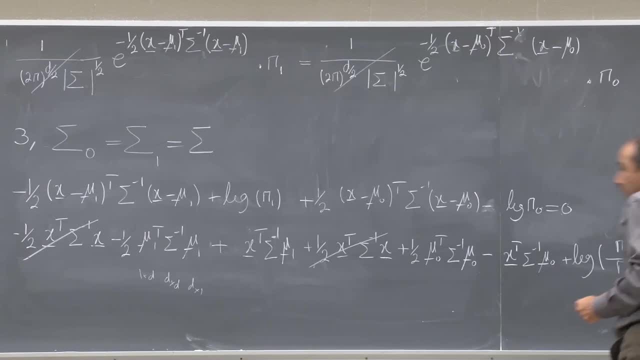 Which has nothing to do with x, so it's a constant here. So I have a term here which depends on x. So Sigma inverse mu 1 would be a vector of d dimension and x is a vector of d dimension, So I have a term here which is linear on x. 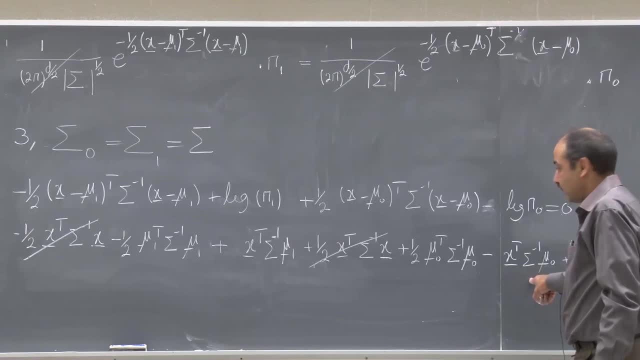 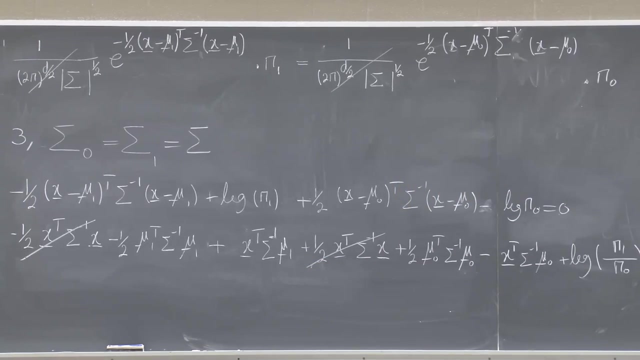 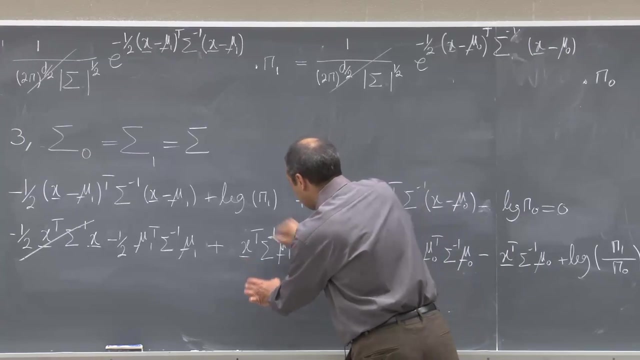 I have another term here which is linear on x. This is also a constant, and this is a constant. So if I order them, I have two terms That are linear on x. so I have, like x transpose Sigma inverse mu 1 Here, and I have Sigma inverse mu 0 here. 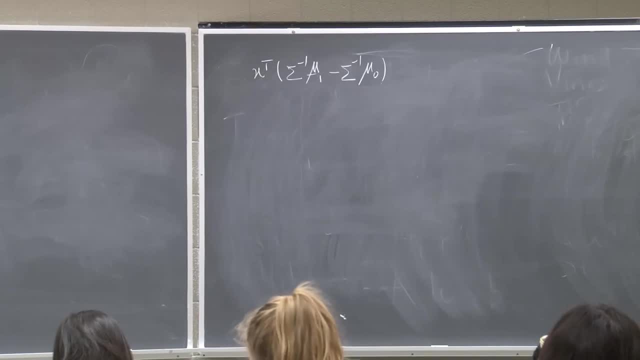 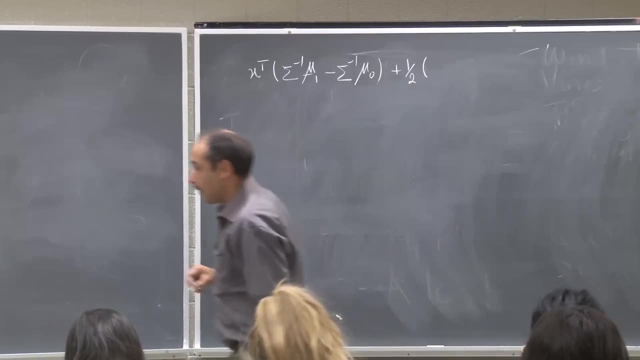 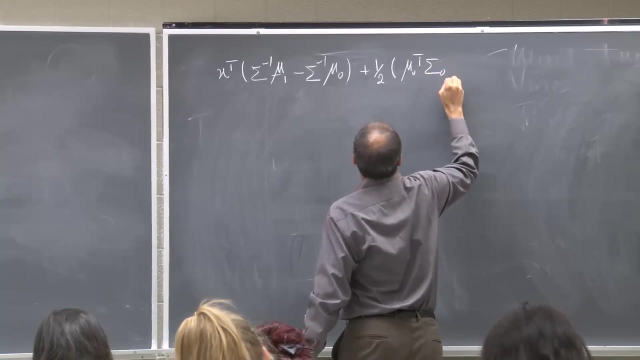 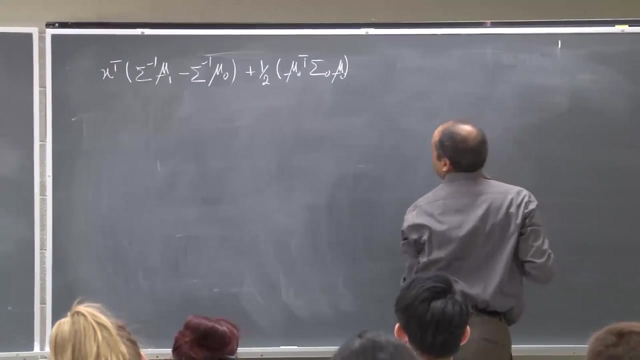 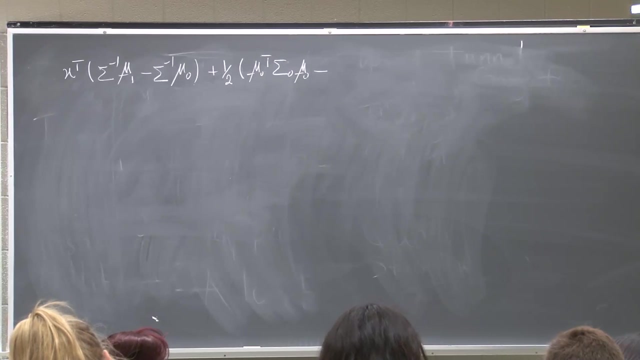 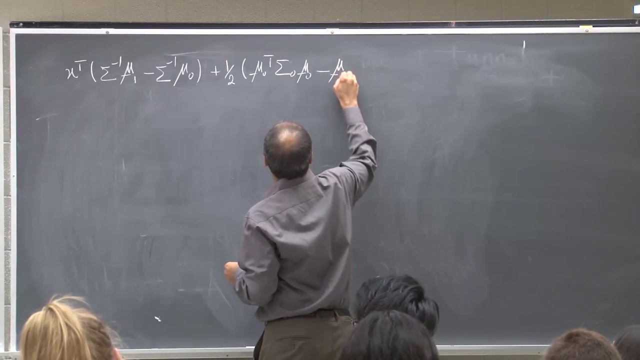 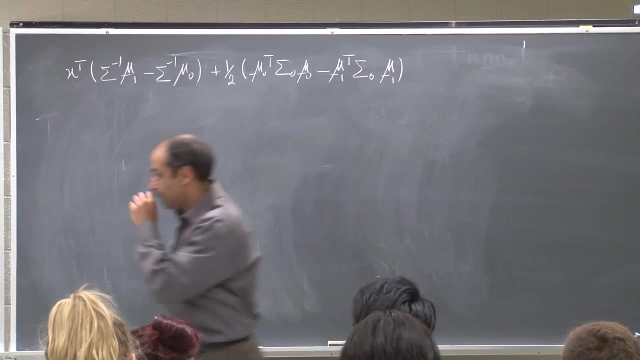 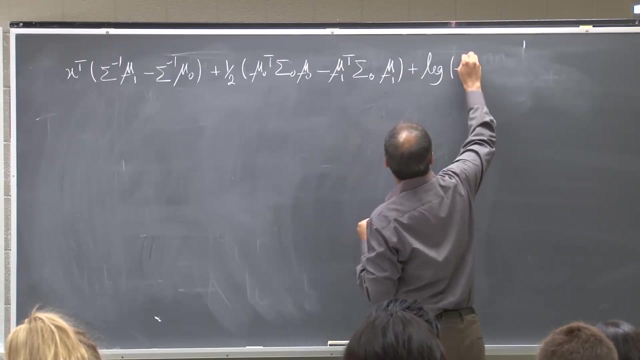 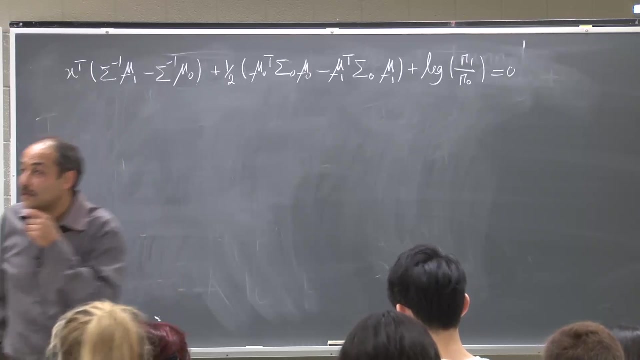 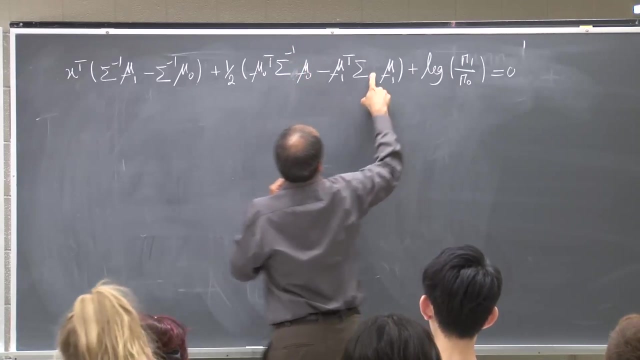 So that's my linear term. then I have constant: Mu 0 transpose Sigma 0, mu 0, Minus this term Mu 1 transpose Sigma 0, mu 1, And then I have this term, Which is again constant, Sorry: Sigma inverse, Sigma inverse. Thank you. 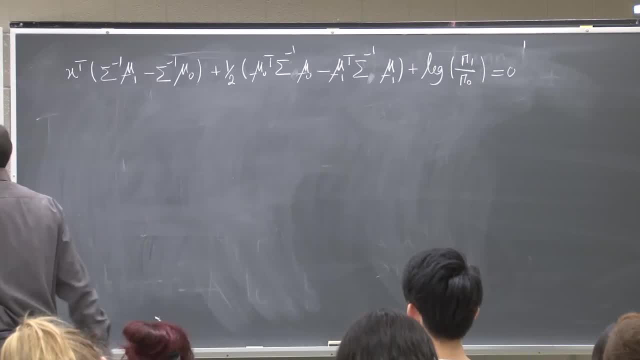 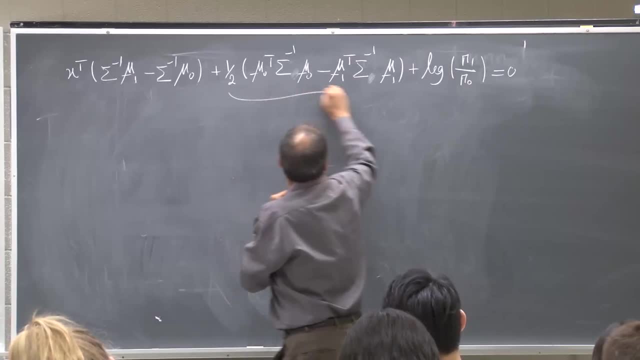 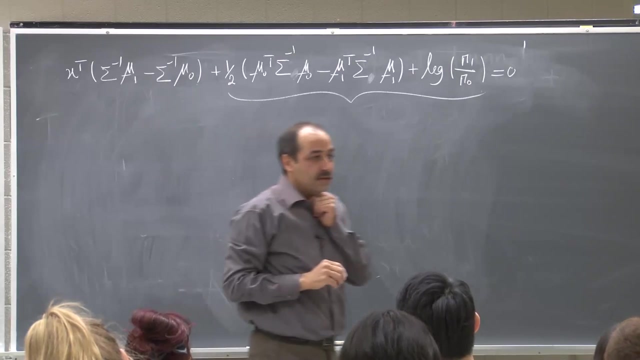 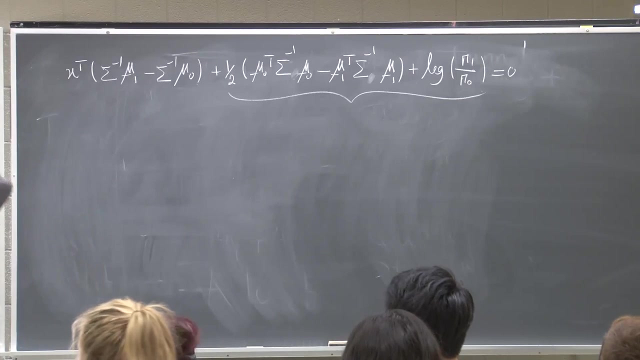 Okay, So I have a linear term on x and constant. What this equation is, I Mean geometrically. what does it look like? Sorry, It's just linear, right, it's a line, I mean in two-dimensional space, It's a line in d dimension. 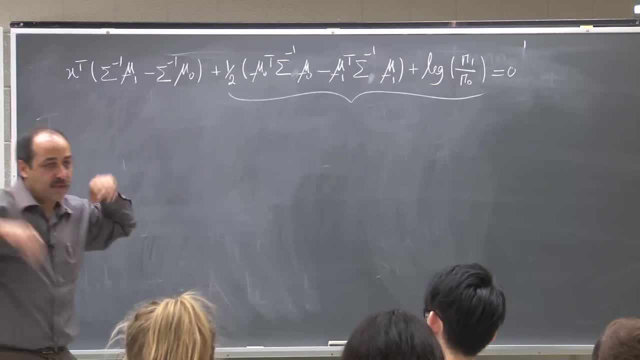 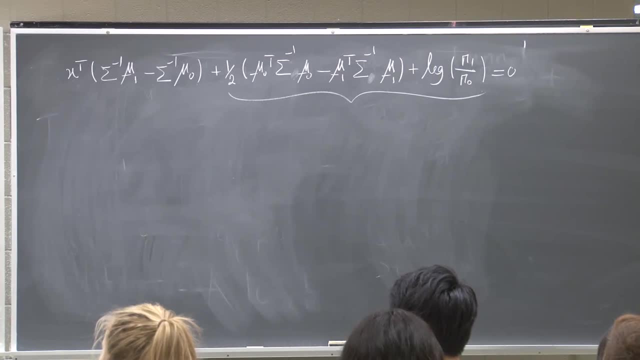 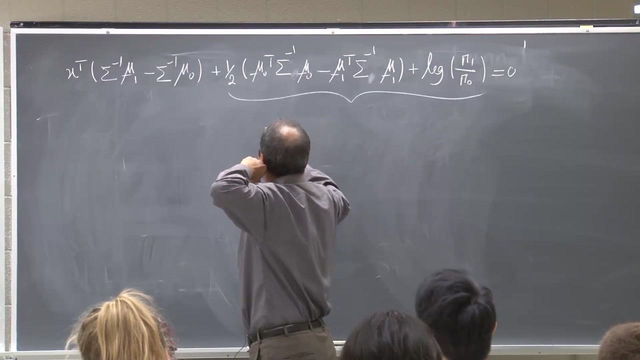 It's dimensional space, it's like d-dimensional hyperplane, So it's a linear function. so We want to compute. we wanted to compute this decision boundary and it turned out that the decision boundary, under this Simplification assumption, is just a line. Okay, so You know, it's a vector. 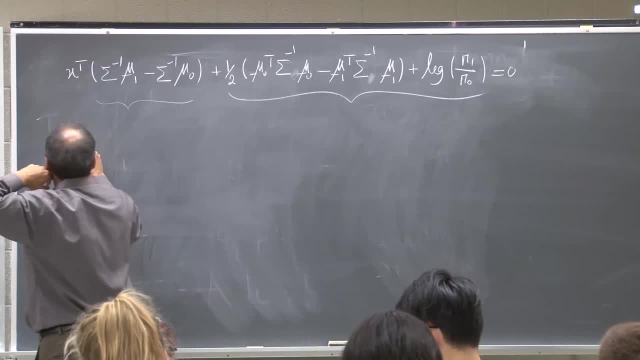 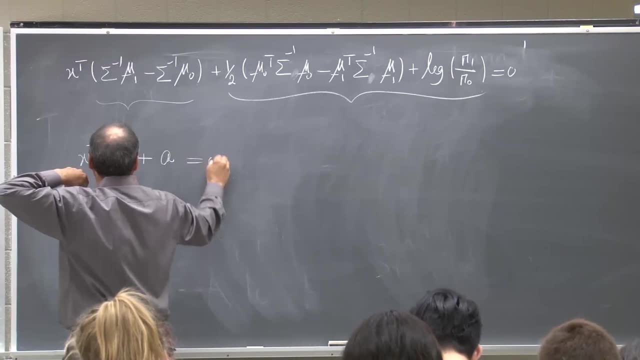 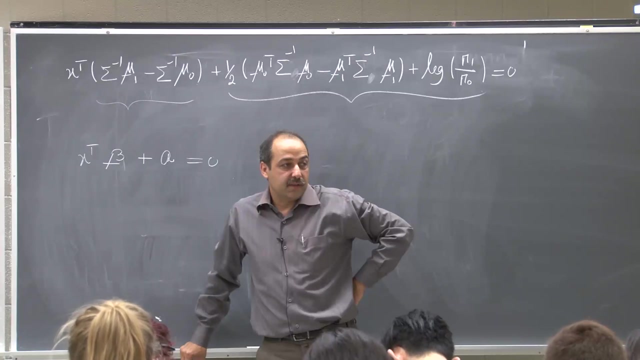 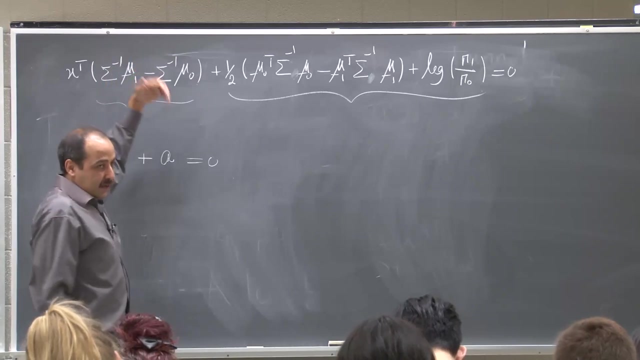 it's another vector. so it's as if you know, I have X, transpose a vector, beta, plus a constant here equal to zero. so if you want to do LDA- linear discriminant analysis- what you have to do is to simply assume that your two classes are. 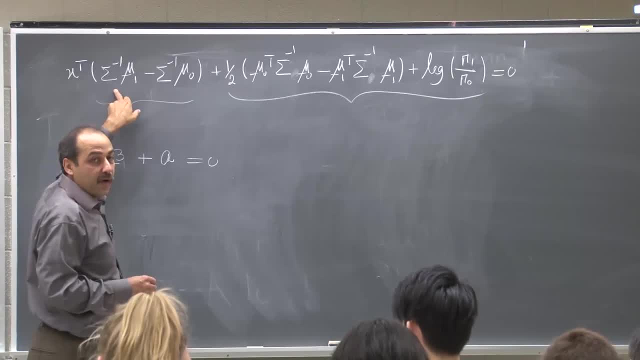 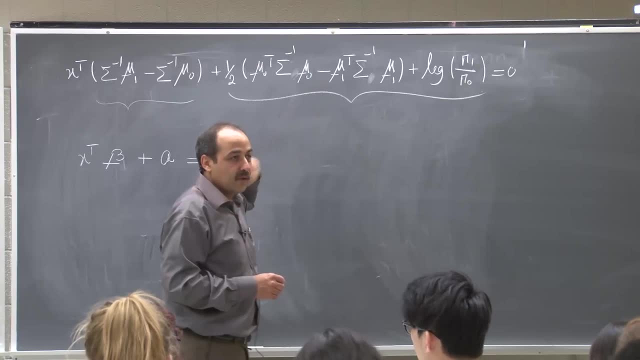 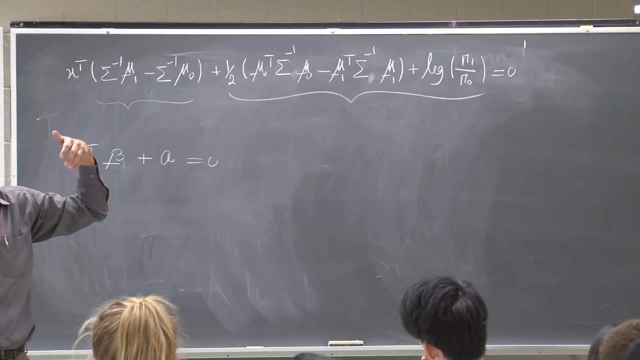 Gaussian estimate the covariance matrix for each class. estimate the mean of each class: mu and mu: zero estimate. the prior prior could be easy to estimate. I will show you the detail in a minute, but it's prior could be easy. just count the number of points in this class. count the number of points on the other class and 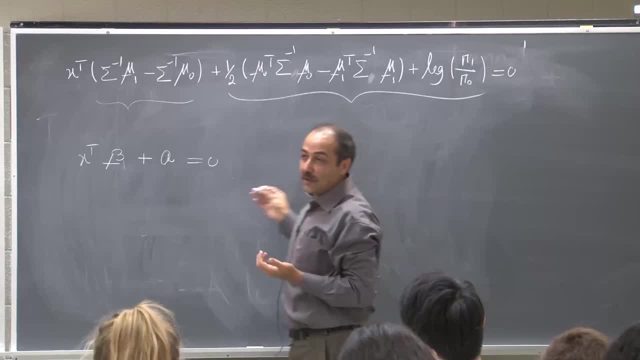 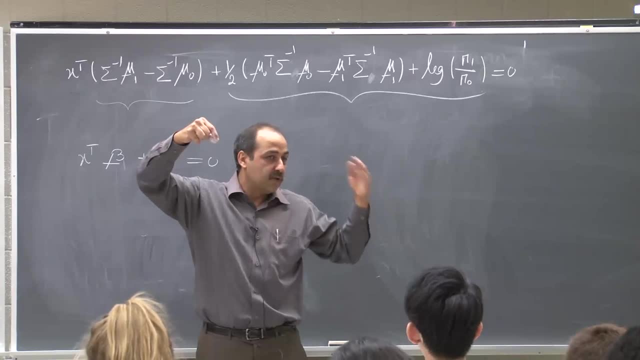 you have all of this parameter, put it in this formula and it gives you, you know, equation for, for a line, a linear equation for a line, a linear equation for a line, a linear equation for a linear equation. so this is your decision boundary. any point on this line has 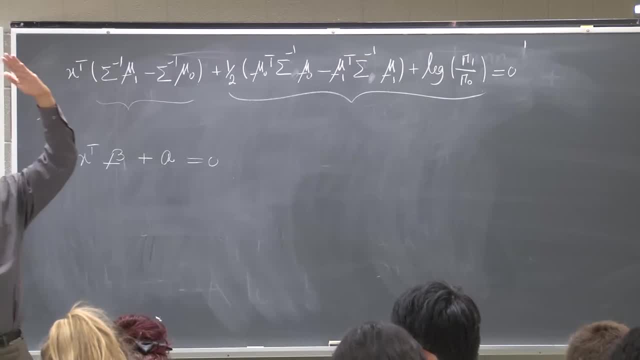 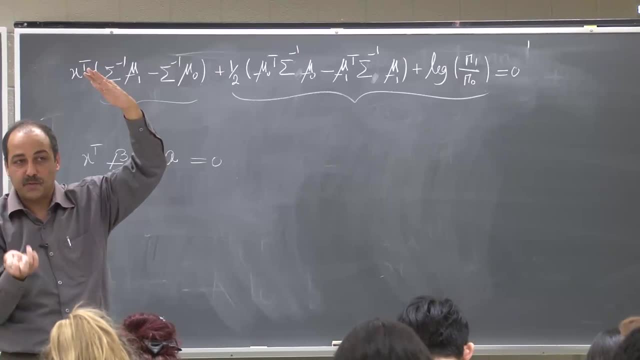 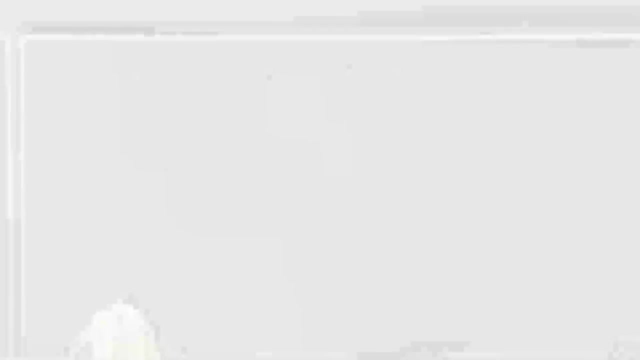 probability of being in class 1 equal to the priority of being in class 0. anything on one side of this boundary has one of this probability more than the other, so we can make decision based on this line. so in LDA, you know, say, for example, I want to do digit recognition and they have three types. 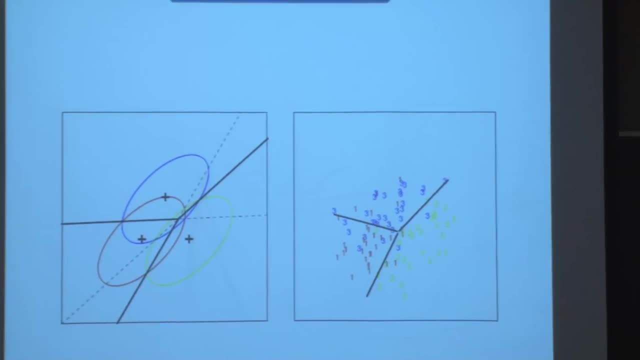 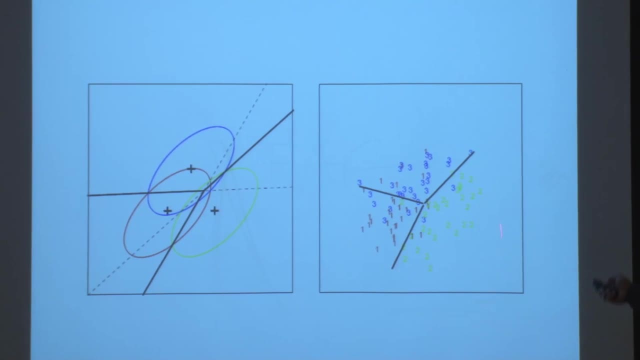 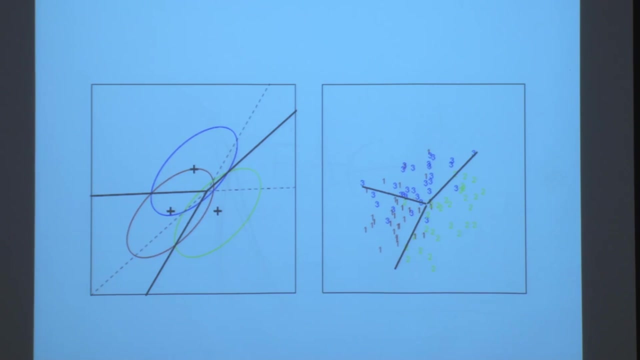 of this. you know, I gave you example for two classes. you can easily extend this to multi-class. so I have digits I. my first assumption is to assume that the distribution of this digits in each class is Gaussian. it's a wrong assumption. nevertheless, I'm going to make this assumption. okay, I'm going to. 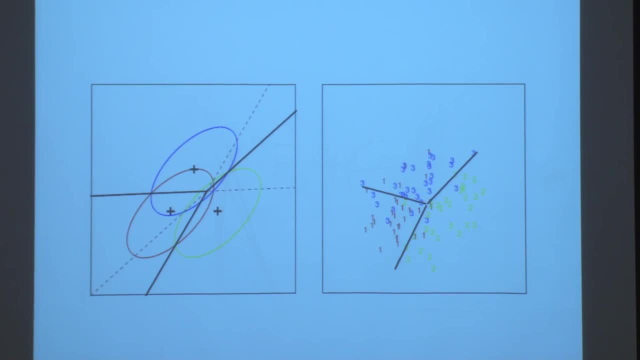 assume that this two have been sampled from. multivariate distribution goes to what? what does it mean? it means you know, I observe this too, but they assume you know that it is multivariate Gaussian, in a sense that if I put it in a matrix, then if I vectorize this based on the resolution of this picture, it's 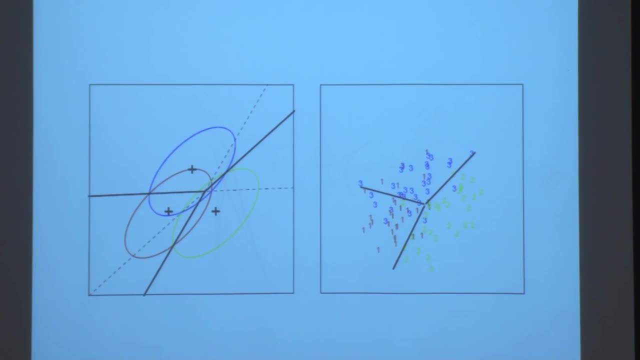 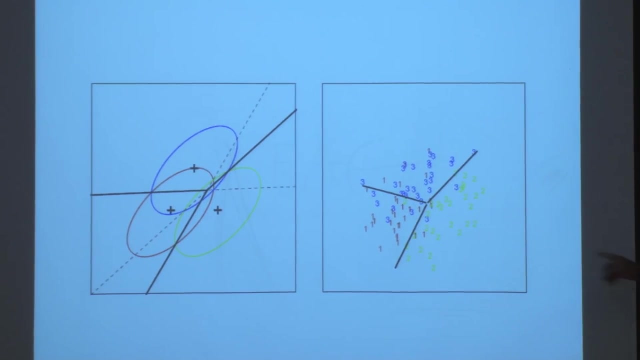 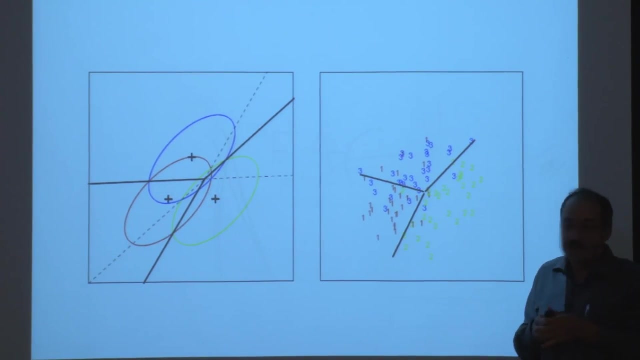 going to be in like something d-dimensional space and they assume the pixels have been drawn from. this multivariate goes okay. so this is Gaussian, this is Gaussian and this is Gaussian. now I can estimate the mean of each of this class. so these are the mean of these three class. I can estimate the covariance matrix of each of these. 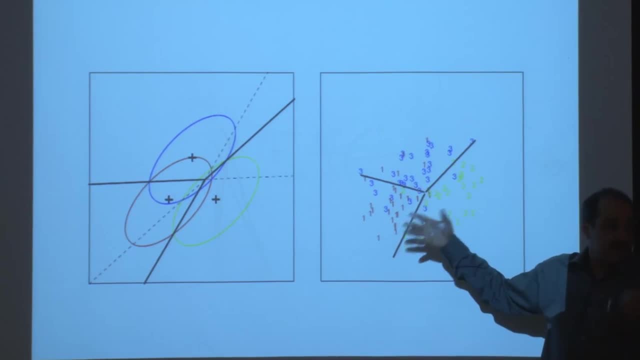 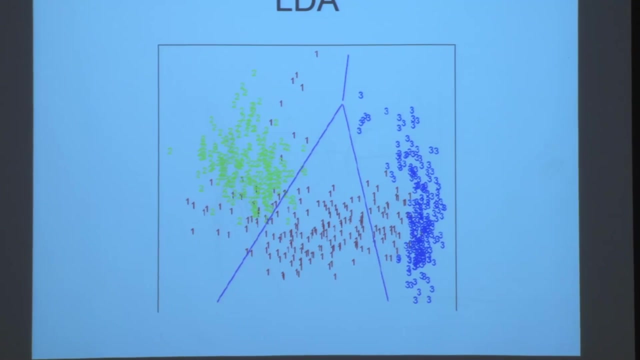 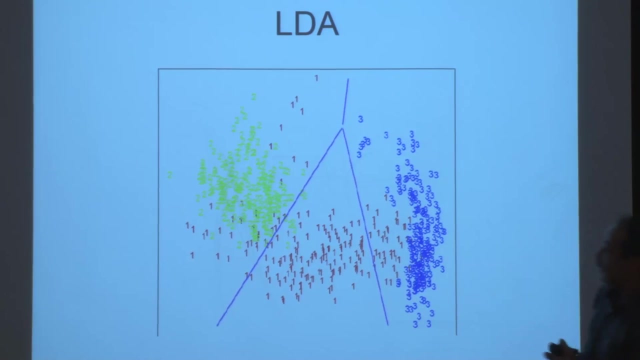 classes, covariance of these three class are not the same. I'm just going to assume that they are okay. I'm going to assume that they are the same, so they have exactly the same shape. if I do so, the decision boundary will be linear. So it gives me a line which makes the distinction between these three. 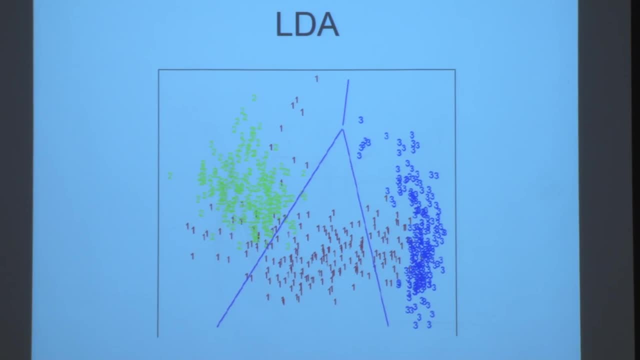 digits, And this is on some real handwritten digits. As you can see, these two wrong assumptions still can give you a decent classifier. This decent classifier, you know, classifies 2 from 1 from 3 in some sense. Any questions? 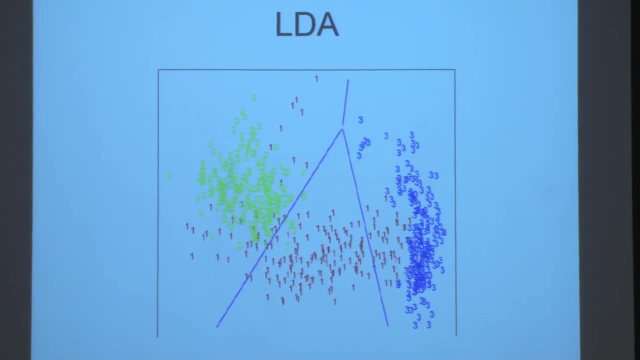 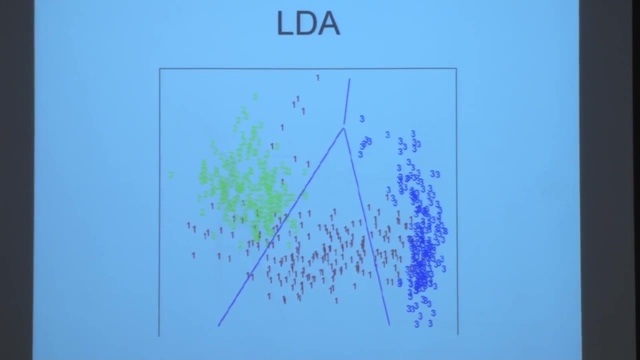 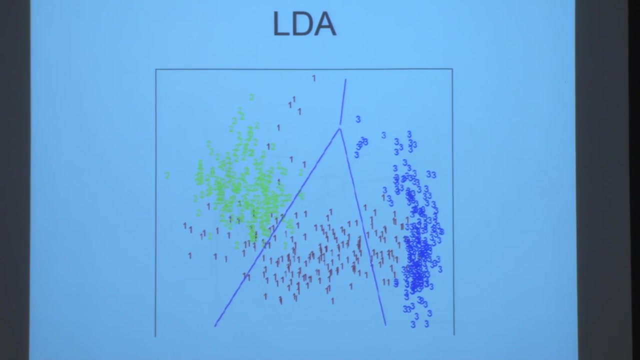 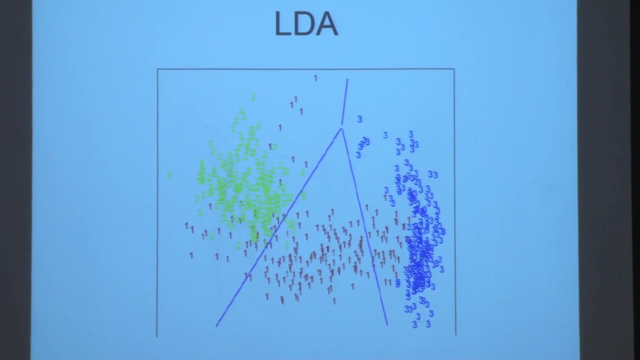 Yes, What is the mean you're estimating? Sorry, The mean of the class you're estimating. What is the mean of what? Well, I go through the detail, but the mean is quite easy, You know. just you take the average In Gaussian. what would be the maximum likelihood estimation of the mean? Just add all of the points, divide by the number of points. That's the mean. That's maximum likelihood estimation for the mean, Right? Yes, 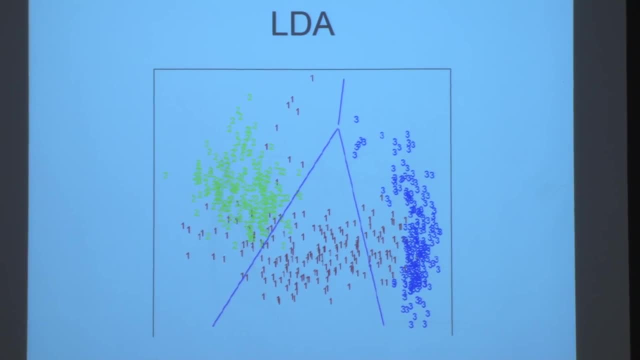 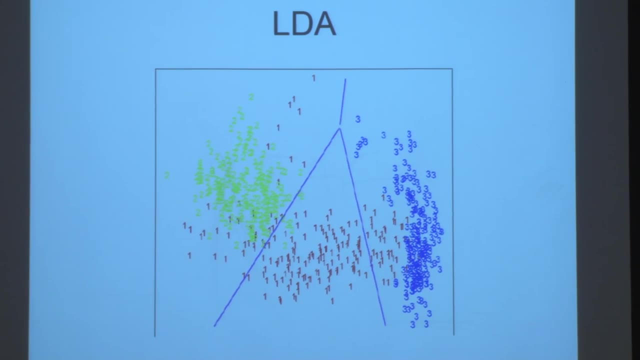 C2.. So you assume that all these two things have all the same covariance equation. Then how is the estimated covariance? You're going to estimate the covariance matrix of each classes. add them up, take the average Again. I'm going to go through details of that in a minute. 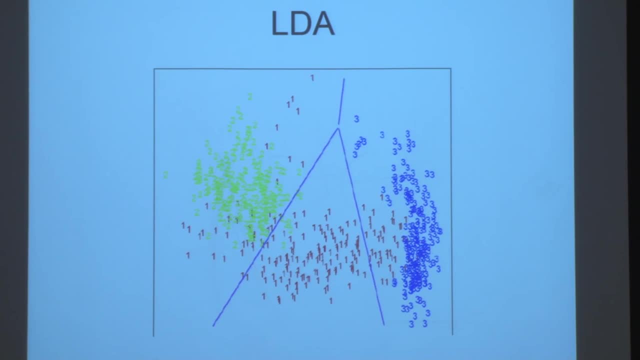 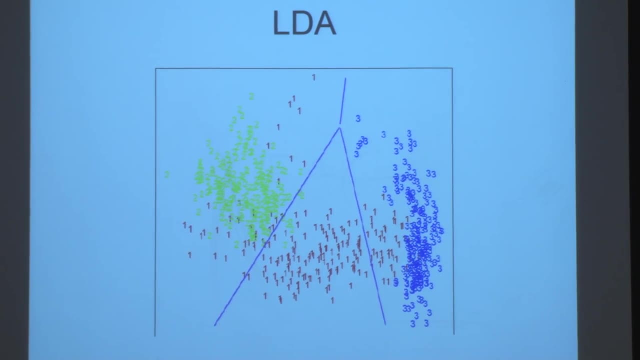 Okay, So since I don't want to again open and close this screen, you know we had two simplification assumption here. one was that the class conditional is Gaussian. the other one was that the covariance of classes are the same. right if I relax the second assumption. second assumption: 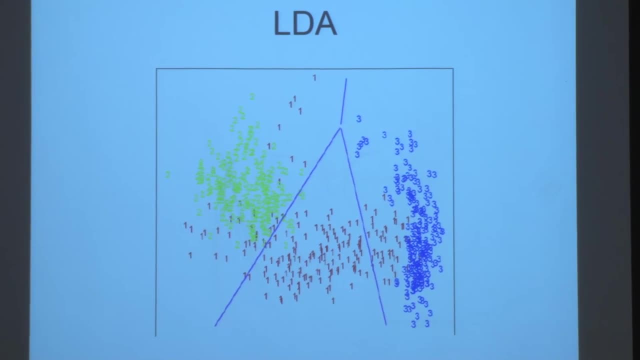 that the class conditional- sorry, the covariance of classes are the same. if I just relax the second assumption, do you know what's going to happen? the shape will change. but how right you know? there, there was a part which is now hidden behind this screen. when we did simplification, there was a. 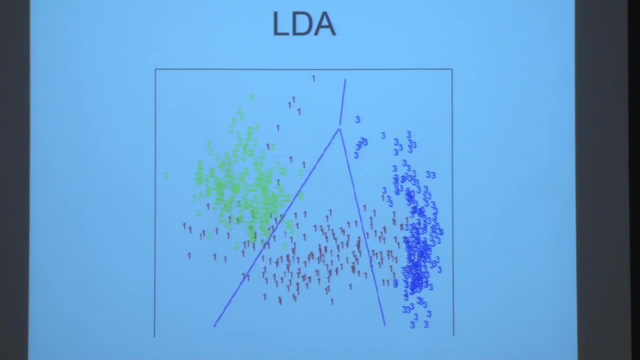 quadruple quadratic form like X. transpose Sigma inverse X, which we cancel out, right? do you remember that from class 1 and class 2 we cancel out this two term? we were able to cancel this term out because we assume that Sigma for both class are the 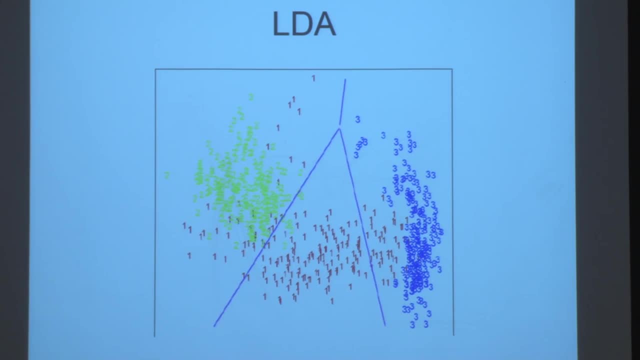 same, because Sigma 0 is the same as Sigma 1. if I relax this assumption, then these two term are not the same. I cannot cancel them out. then I have another term here, which is quadratic. so if I relax the second assumption, then my decision boundary is not linear anymore, it's quadratic, and this is called quadratic. 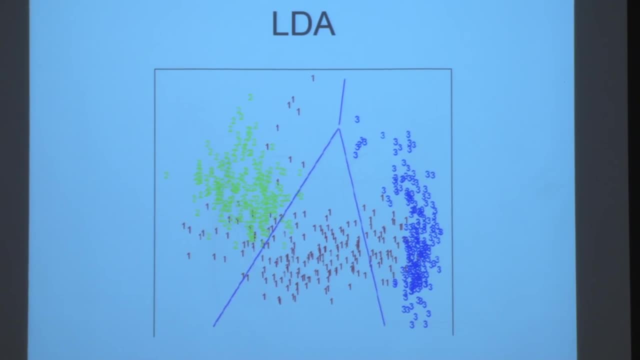 discriminant analysis. so linear discriminant analysis is based on the assumption that class conditionals are Gaussian and covariance matrices are the same. quadratic discriminant analysis is based on the assumption that class conditional distributions are Gaussian but covariance matrices are not the same. So in this case you're gonna have decision boundaries like this, You know. 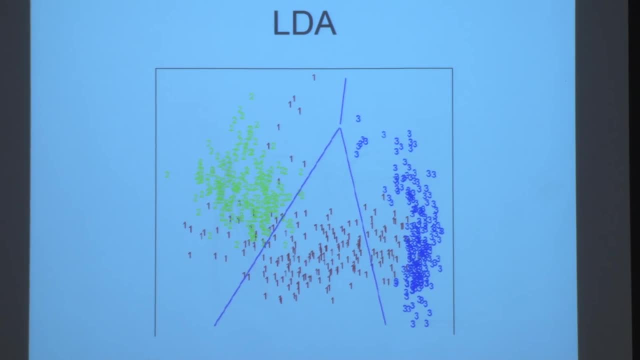 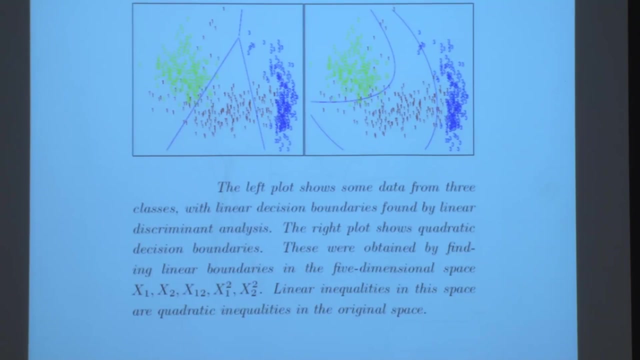 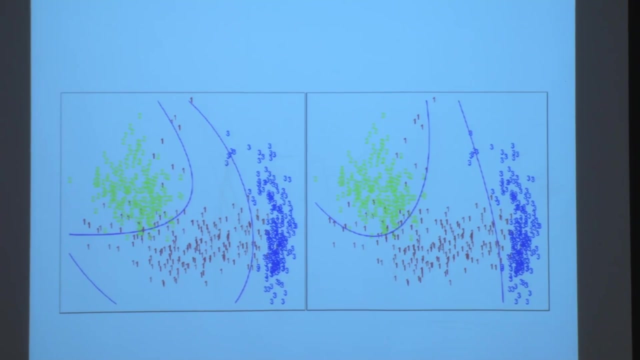 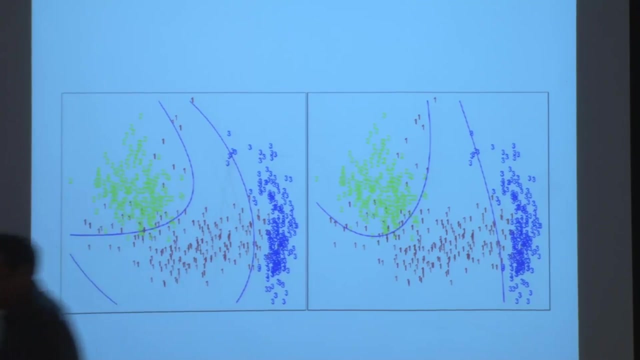 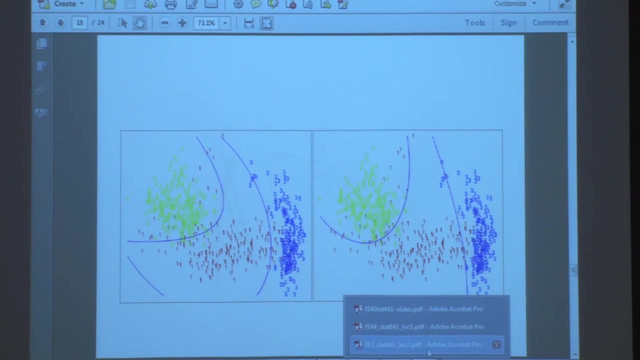 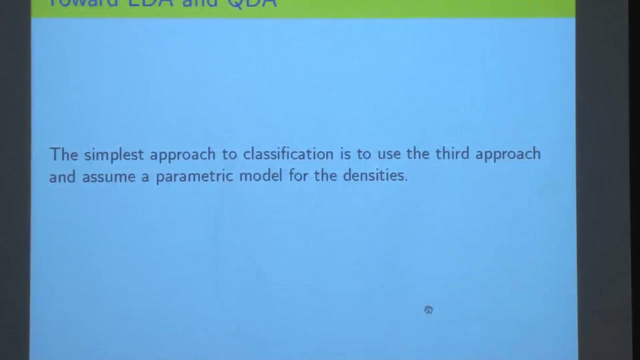 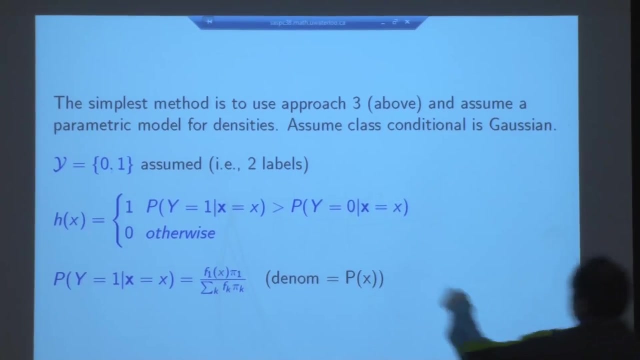 compare these two. This is linear. Relaxing this assumption, it becomes quadratic. Okay, it changed the shape of your decision boundary to quadratic shape. Okay, any question. Drawing and measuring constraints. observing C under individual Dobviol: Okay, we learned how to do LDA on on Blackboard, so I'm going to skip this. 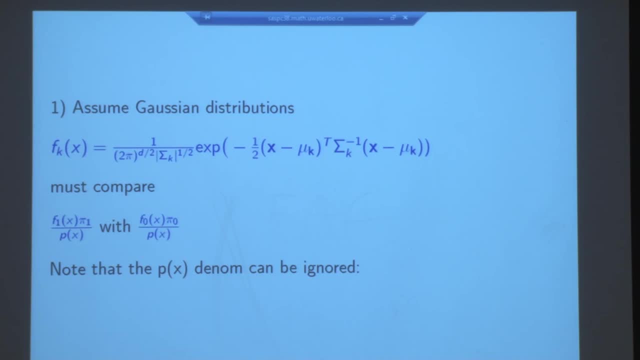 this slide. this is just I we have. we know the details of the. you know this Assumption and how to make simplification come up to this linear and okay Here I'm gonna stop my lecture at this point because I'm just saying it might be faster. I'm going to let you learn afication, afication. 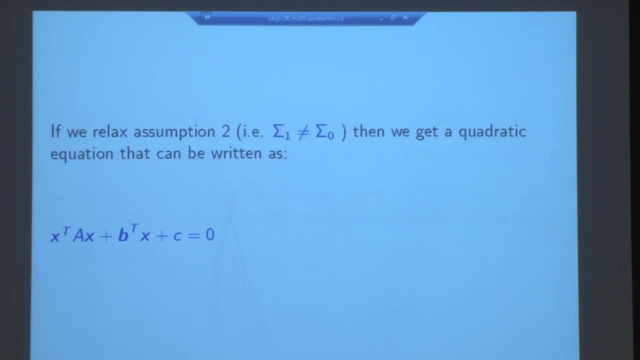 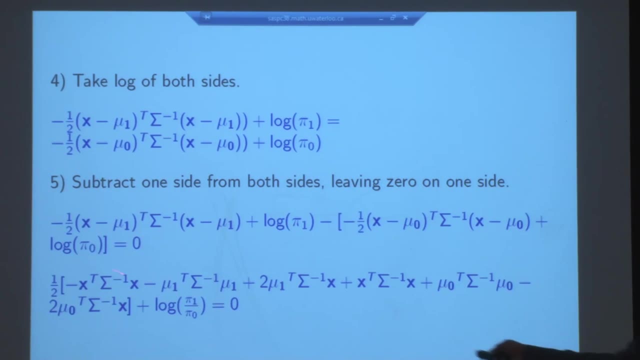 This is the formula, It's just another example in Linear and ط linear And okay, I came up with this. It suits me. Okay, I came up with this product easily. Here you know, we had this term: X, transpose sigma, inverse X. 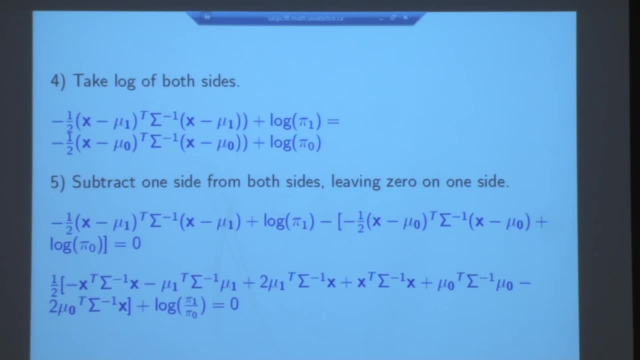 and we had X transpose sigma inverse X and we canceled them out. That's why we got the linear decision boundary. We canceled them out, as I said, because we assumed that these two sigma are the same from both class. If I relax this assumption, they won't cancel each other. 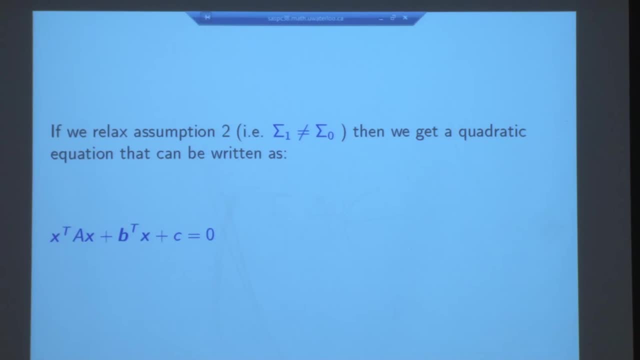 So my decision boundary will not be linear anymore, it's quadratic. So I'm going to have a term like this, and you already have seen, you know the shape. Okay, with the assumption that sigma one is not the same as sigma zero. 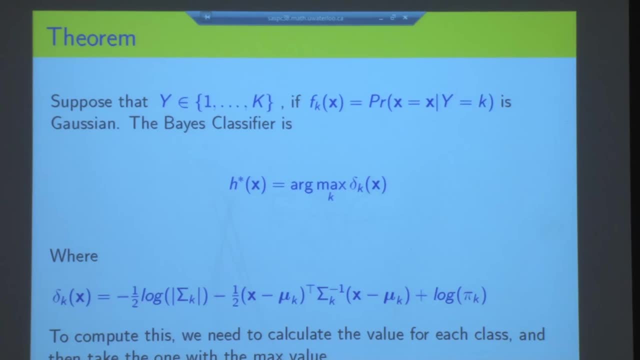 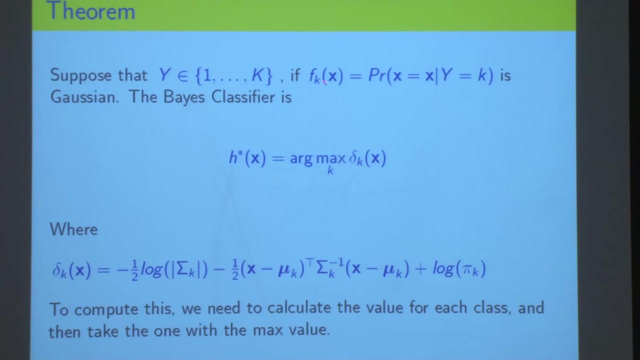 So now, in general form, that's actually what we can do. Suppose that you have K classes and suppose that you know this class class conditional is Gaussian, then your base classifier, which is arg max of this quantity, 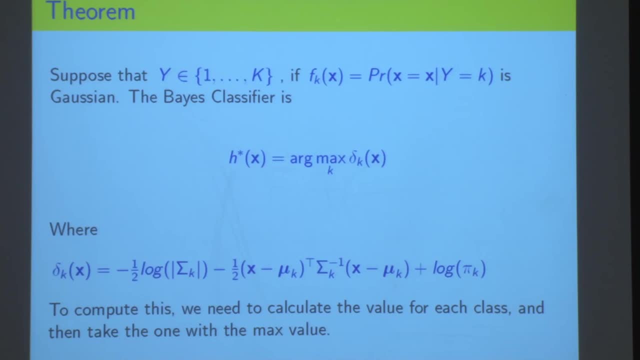 when this quantity is this. you know, basically you can do quadratic discriminant analysis for K classes just by computing this quantity for each of these K classes as compared, And I think you can easily see where this, for me, is Okay. 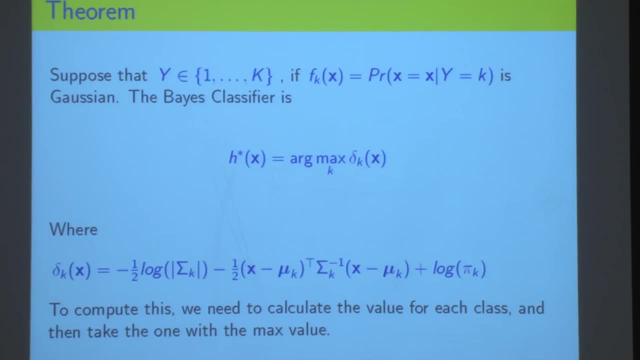 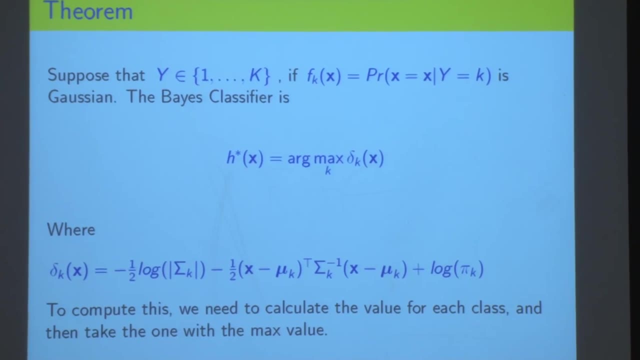 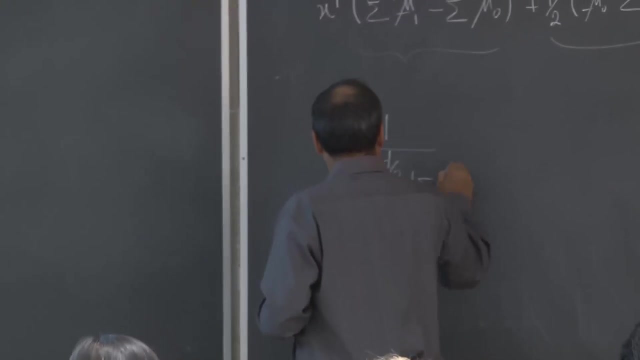 So how does this kind of formula comes from? You know, if you have this, if you have this multivariate Gaussian, you can put it in, you can put it in the bracket, you can put it in the bracket for each of these K classes. 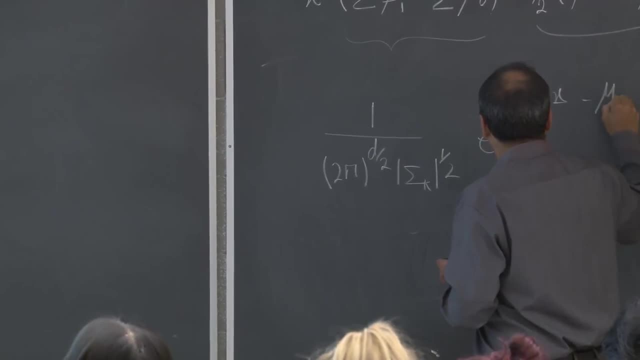 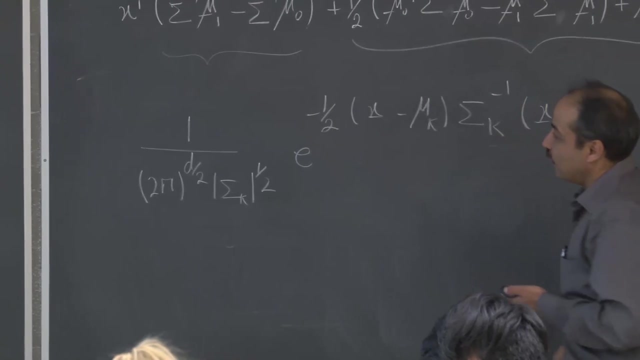 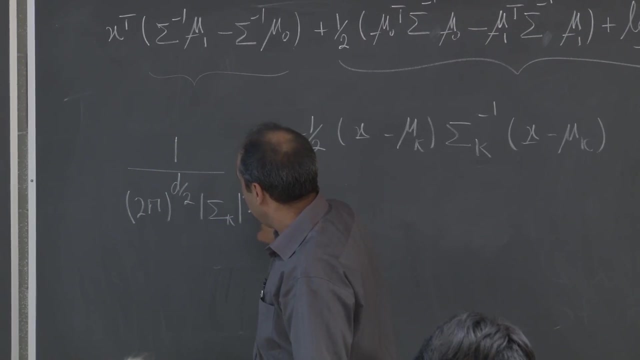 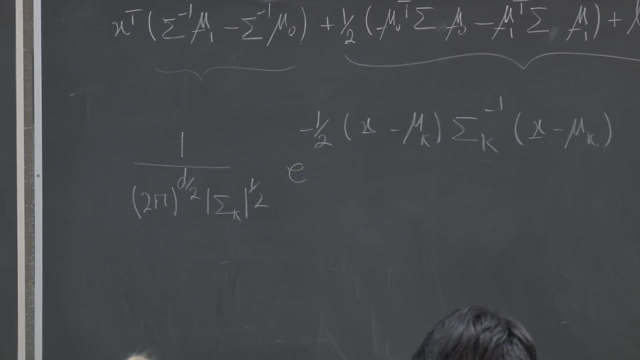 And then you can put a formula by taking this formula and you have the idea of the formula. if you take log from this, you're going to have minus one half log of determinant of Sigma K just here, and then you can get rid of this E you're. 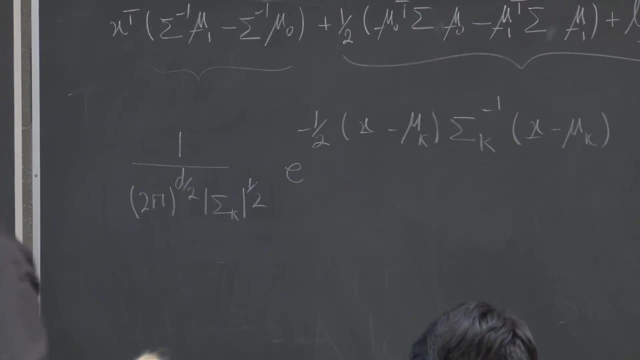 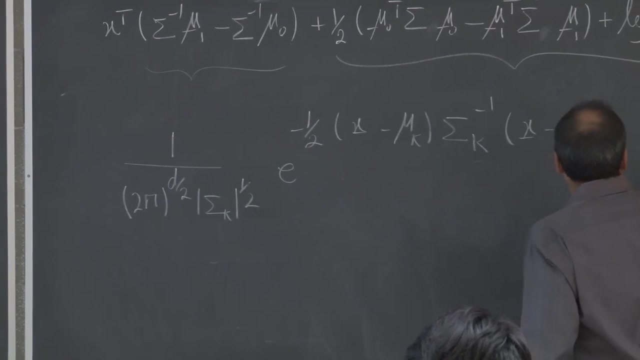 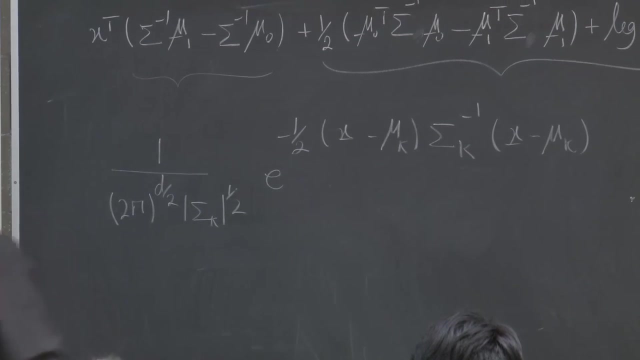 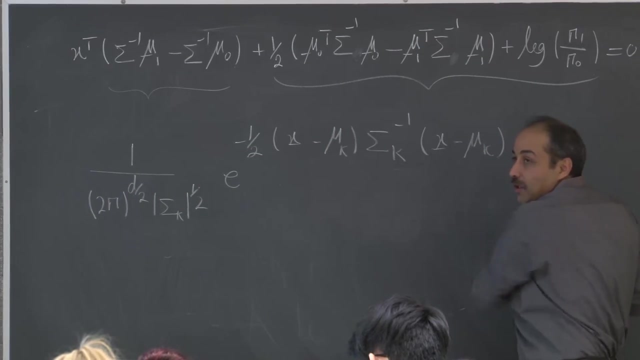 going to have minus one half of this term, which is here, right, and then that was your prior plus log of PI K. so basically, what this quantity is is just the log of class conditional times prior. so you have K classes label belongs to the class conditional times prior. so you have K classes label belongs to. 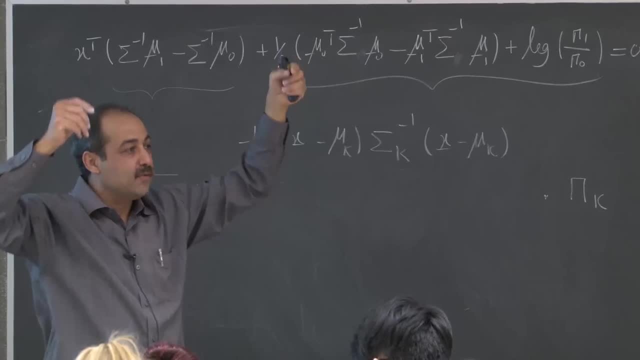 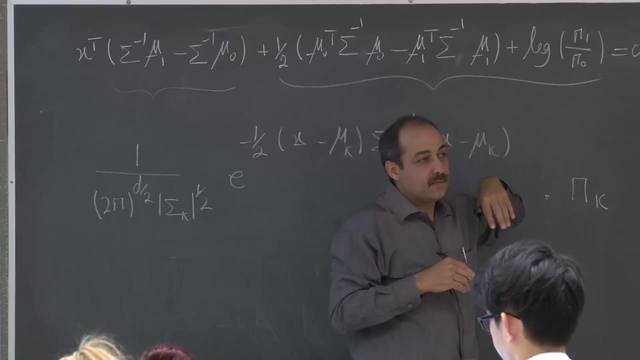 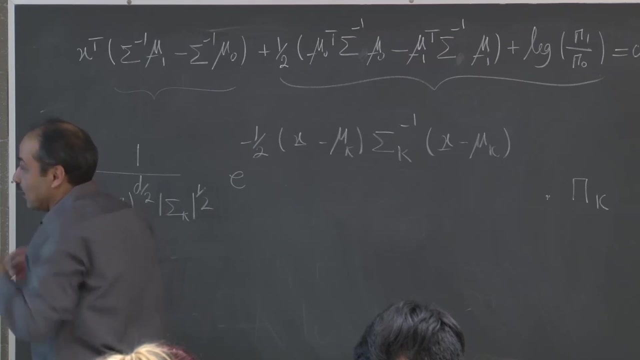 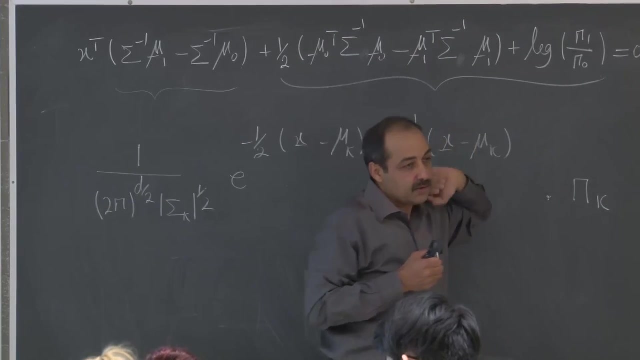 the class which has the maximum posterior or maximum class conditional times prior. log is, you know, in a stuff. just maximizing this, you can maximize the log of this function, right? so what would the? for this formula is basically the log of class conditional times prior. so compute this quantity for each. 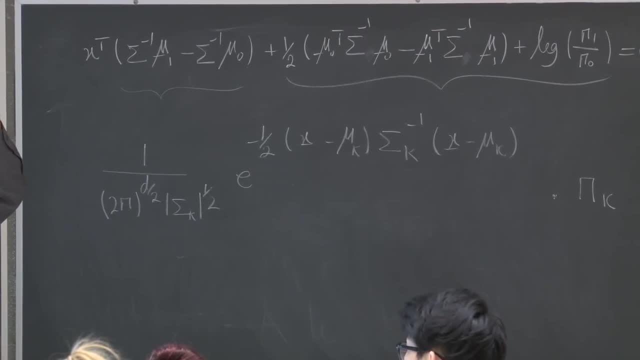 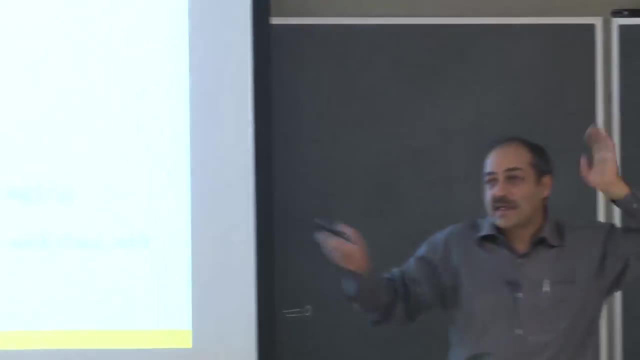 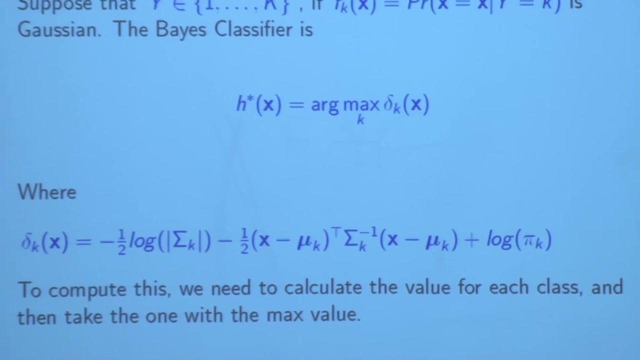 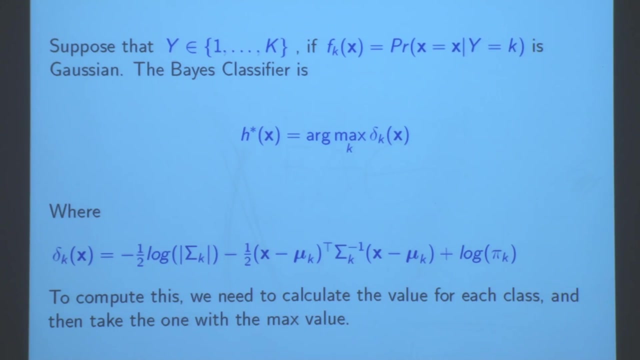 classes. when you have K classes, compute this quantity for each classes. when you compare them, assign the label to the one which is the maximum value. so that would be your base classifier in multi class scenario. when you have, you know, K classes and you don't, you didn't assume that Sigma's are the same. okay, and you. 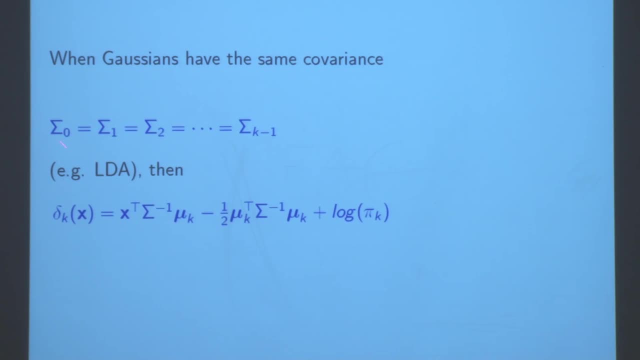 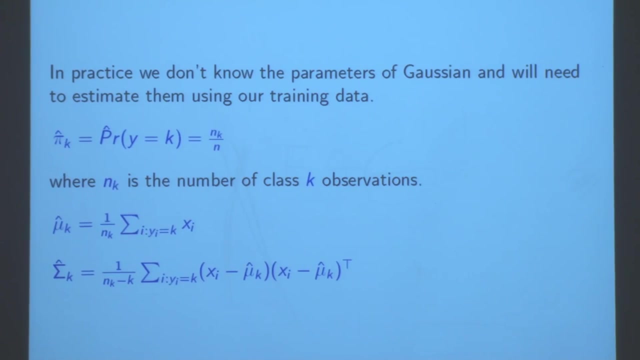 know, if you assume that all of these classes are the same, then it's LDA, otherwise it's QDA. You know, in LDA, your Sigma will be simplified in this form: Okay, how do we, how can we in practice, how can we estimate these parameters? So you know, we made an assumption about the 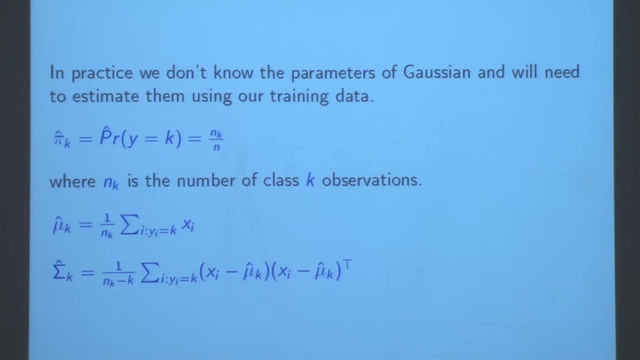 form of the distribution. we assume that it's Gaussian, but still we need to estimate the parameters of this Gaussian: the mean, the, the covariance and so on. we need to estimate the prior as well. So estimating the prior is very easy. Okay, I have 100 points. 10 of them is in class 1, 90 of them is in class 2. so NK divided. 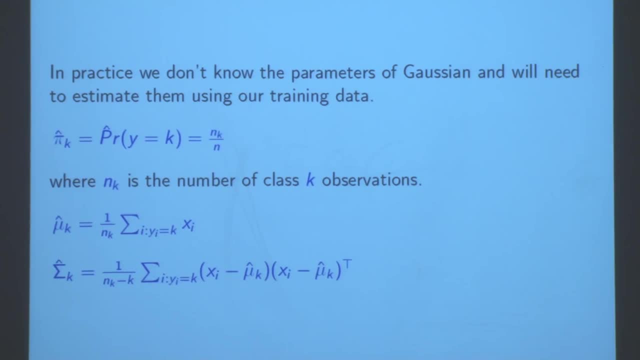 by N. N is 100 and K is the number of point in class K. 10 over 100, 1 over 10 is my prior about class 1.. 9 over 10 is my prior about class 2.. Okay, so easy. so, based on the assumption that 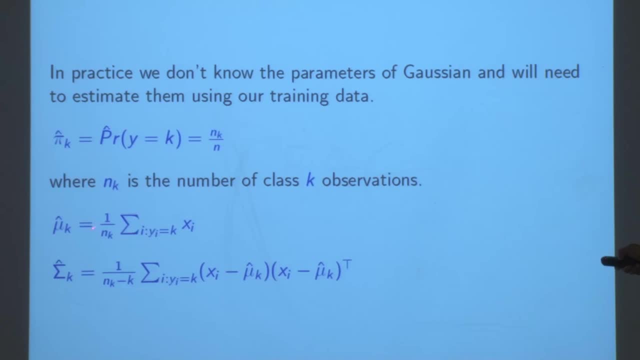 it's very newly distribution. How can I assume mu mean of each class, The, which? the maximum likelihood estimation of the mean of Gaussian is just average, right, So take the average of point in that class. you know, I give you two classes and I assume there are 10 points here, 90 points there. Take this, 10 points add. 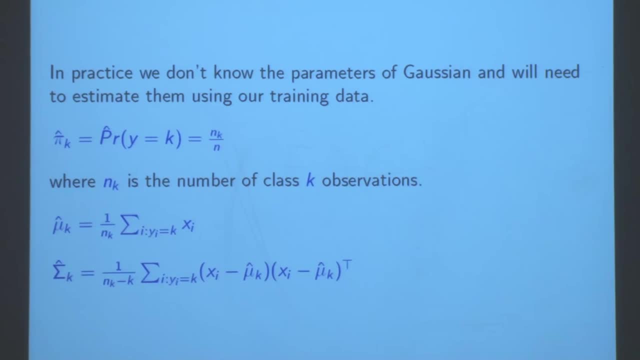 them up, divide by 10, that's your mu. Take this 90 points, add them up, divide by 90, that's your average for the other class. So it gives you the mean of each of this class. Okay, yes, In the terms of text recognition. 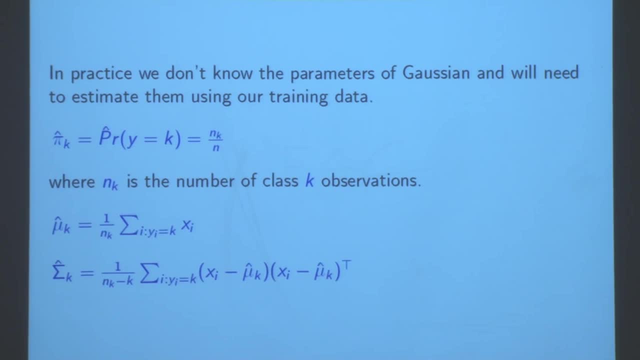 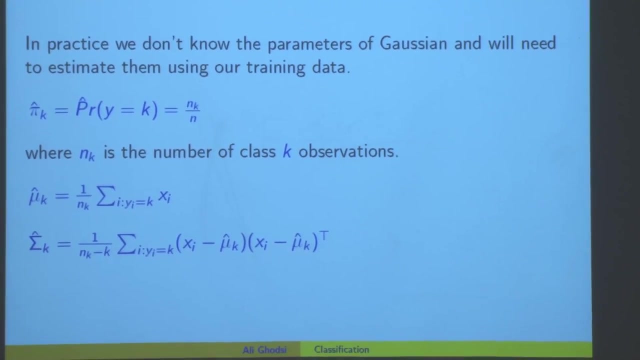 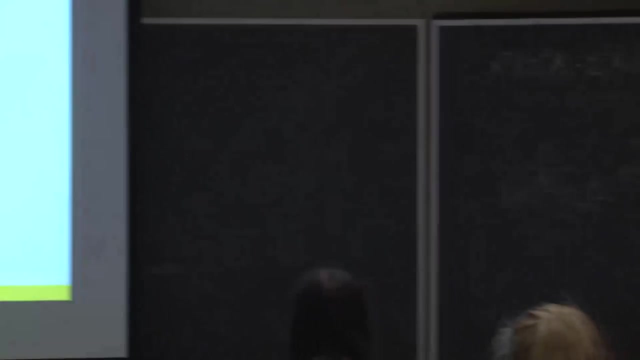 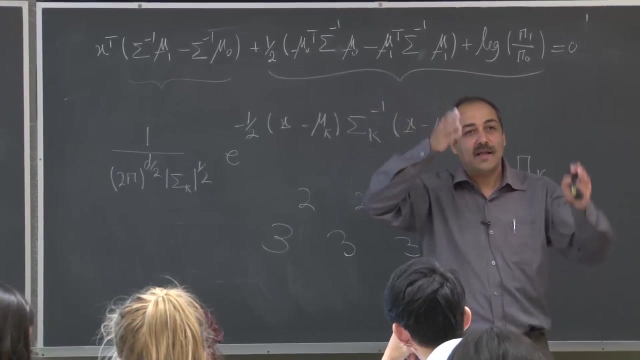 Okay, right, Just images. you know, I give you set of images. these are twos. Okay, I give you in training set. I gives you some trees. These are. each of them can be represented as a vector, right? So each of them is a d-dimensional vector. Add all. 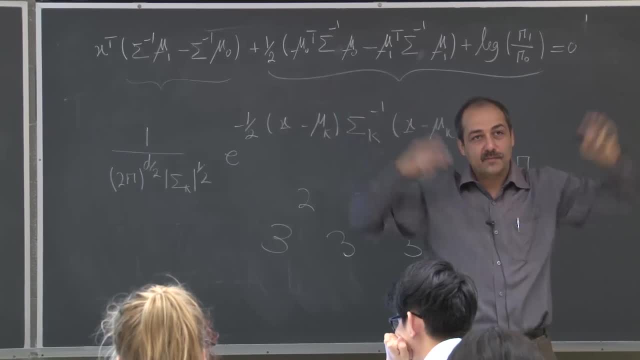 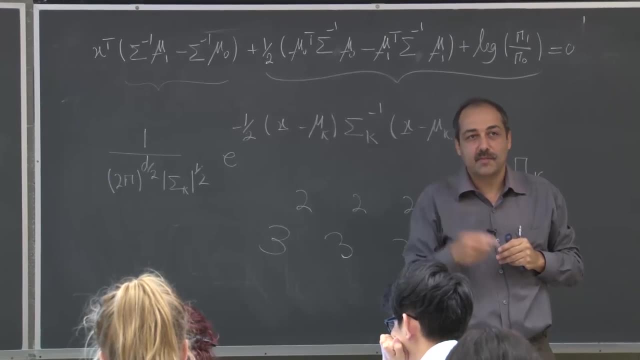 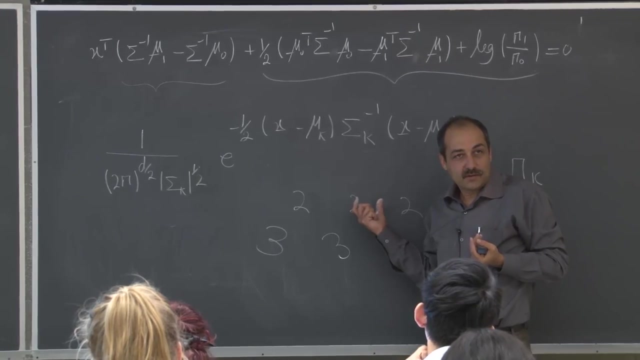 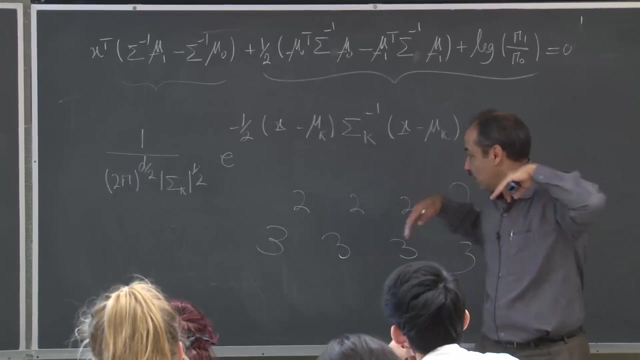 of these d-dimensional vectors. divide by the number of them, Yep, value of the pixels, adding up divide by the numbers. So, and then you can reshape it and look how this image look like. you know It's sort of blurred. 2. You know which is average of all of twos that you have observed, average of all of. 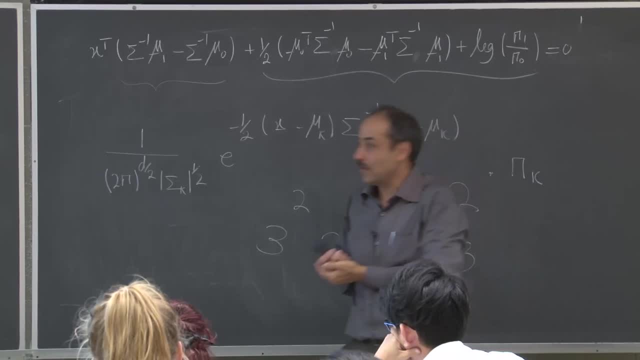 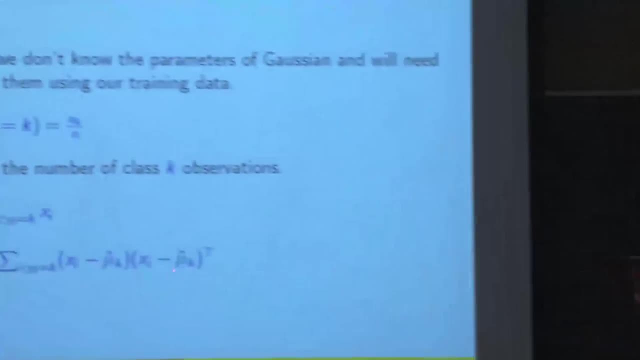 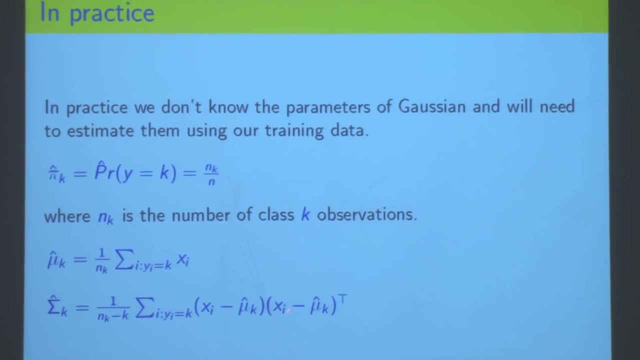 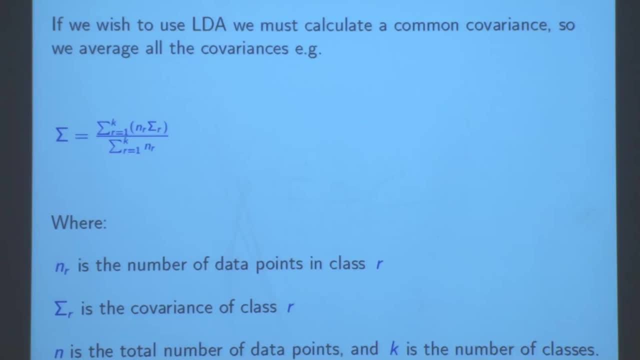 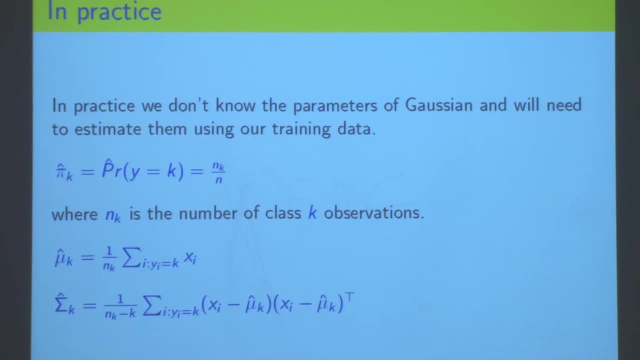 Okay, Okay, so this is sigma k, that's covariance for each class. So, basically, if I have, you know, if I have twos here and and 3 is here and 1 is here, I can estimate this covariance matrix here, here and here. 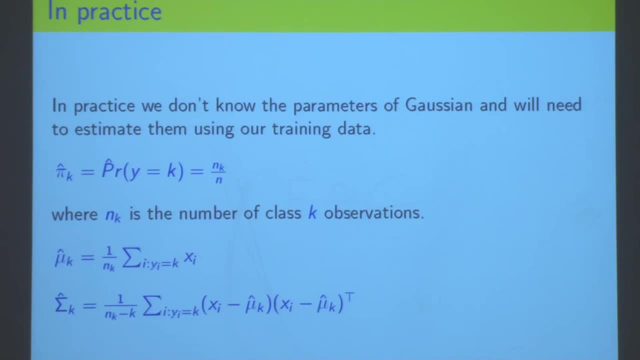 But if I want to do LDA, I mean the assumption is that covariance matrices are the same. I computed three different covariance matrices. I just need to take the average of these two covariance matrices. So my sigma would be just summation of the covariance matrices. 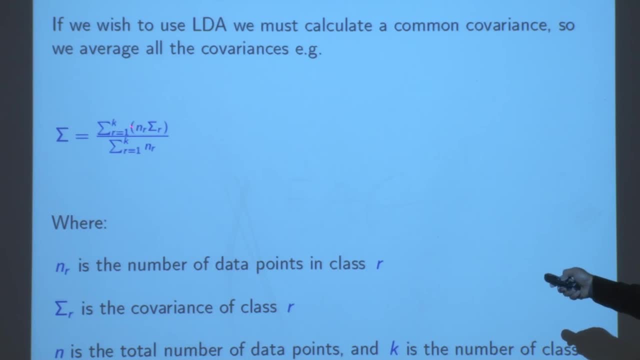 that I had divided by the number of points and this summation could be weighted. You know, if I have 10 points here and I have 90 points there, I give more weights to 90 points. So 90 times this one plus 10 times the other one divided by 100.. Is that clear? 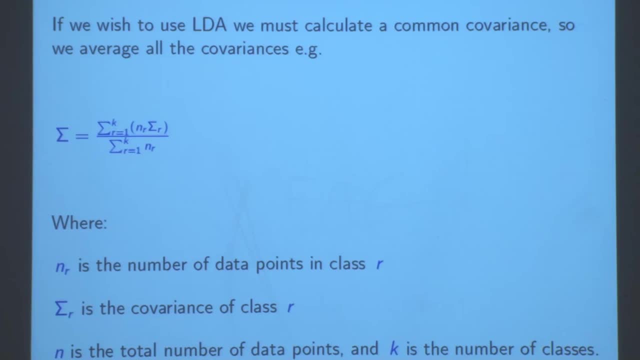 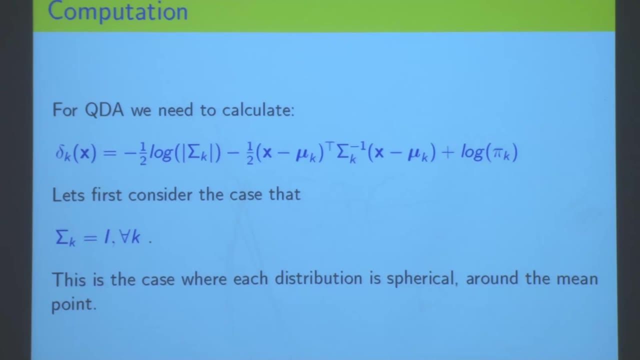 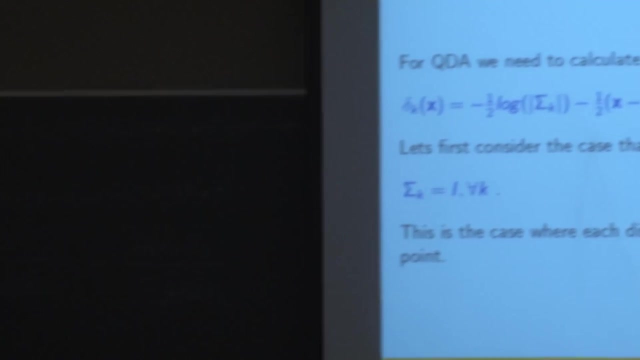 Okay, Okay, Now let me show you something which, in terms of computation, sometimes could be useful and it gives us pretty good insight about the nature of this equation. So let's look at the covariance techniques. nature of LDA and Q. You know, this is the quantity. 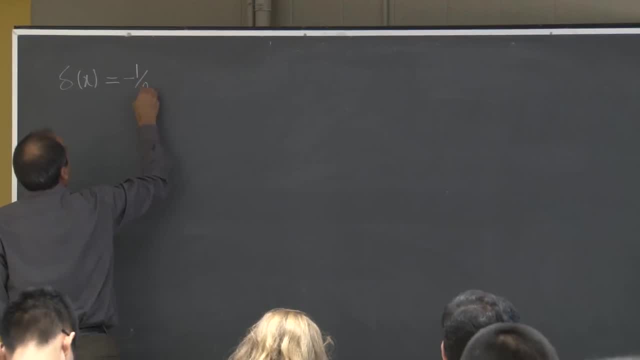 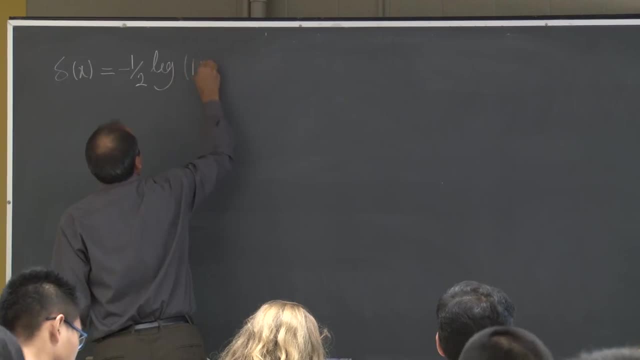 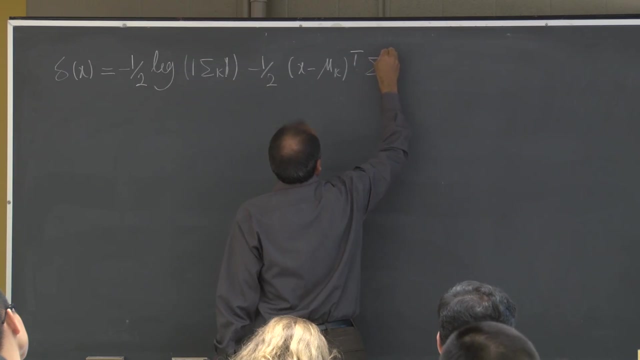 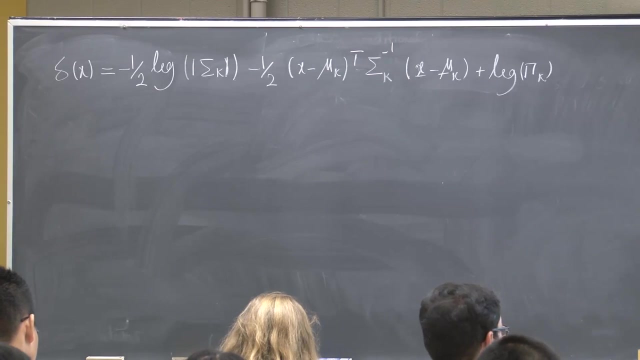 that I'm going to compute. Okay, This is a quantity that I'm going to compute in the case that I want to do multiclass classification. Okay, Okay, Okay, Okay, Okay, Okay, If I assume that this sigma is identity, let's just assume that sigma is positive. 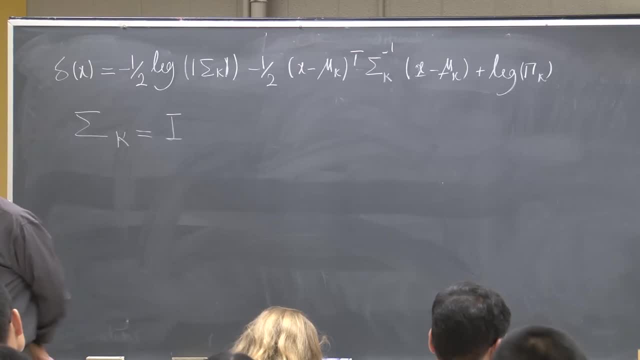 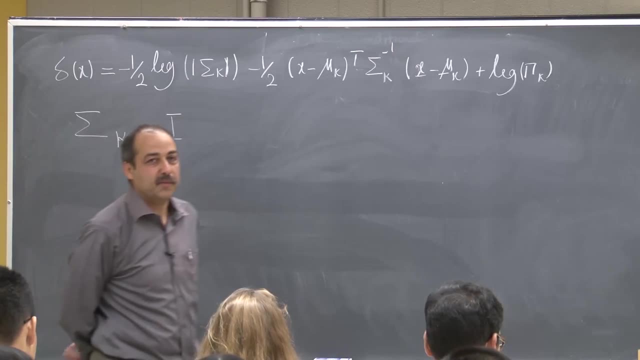 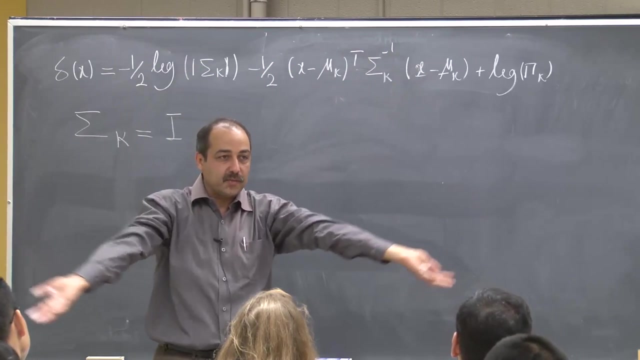 Let's just assume that. let's just assume that the sigma is positive. that sigma is identity. What does it mean? It means that the Gaussian that I have in each class, or in class K, is like a spherical shape. right, Gaussian is a spherical shape. 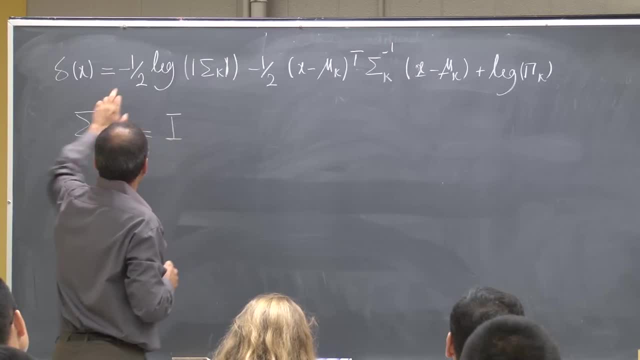 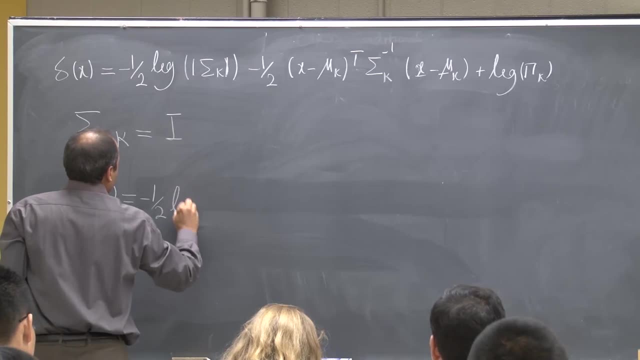 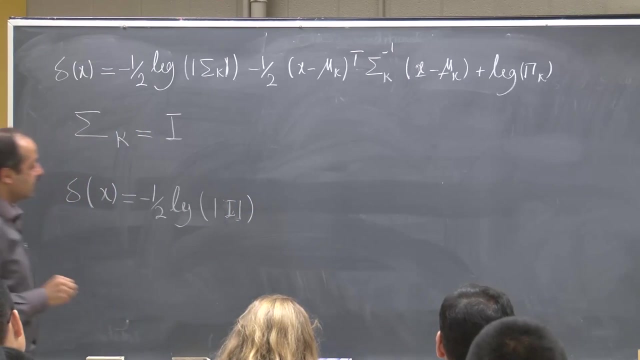 So, if I assume that this is Gaussian, see what's going to happen to my sigma, to my sorry, this delta. It's going to be minus 1 1⁄2 log of determinant of I. and what's the determinant of I? 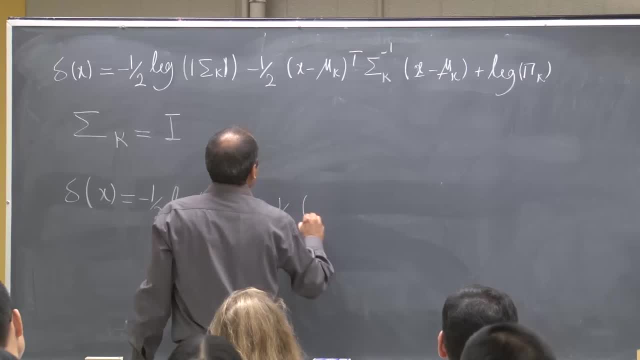 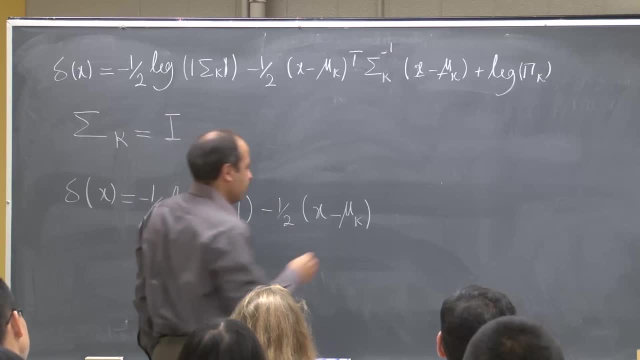 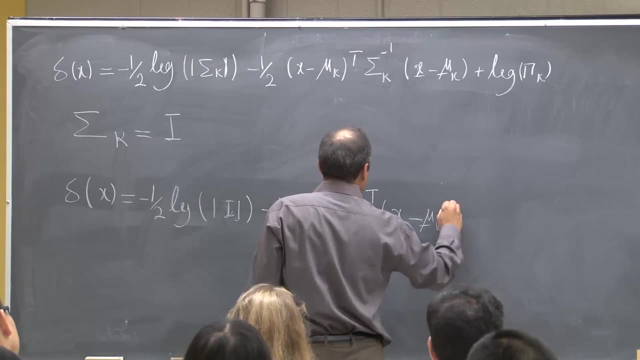 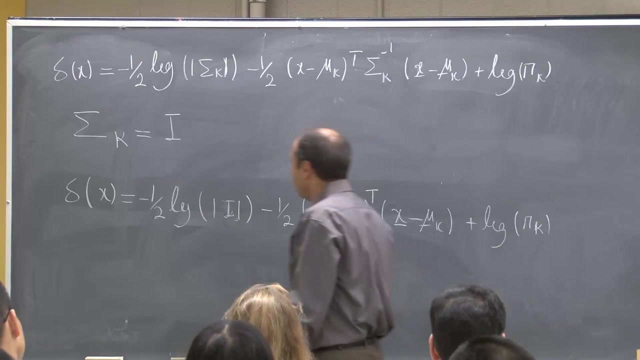 One Minus 1⁄2 X minus mu K, and this is I. the inverse of I is I X minus mu K plus log pi K. okay, So this first term is log of one, which is zero. So this first term is zero. 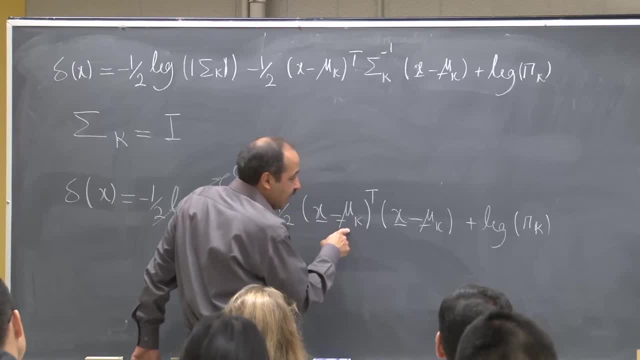 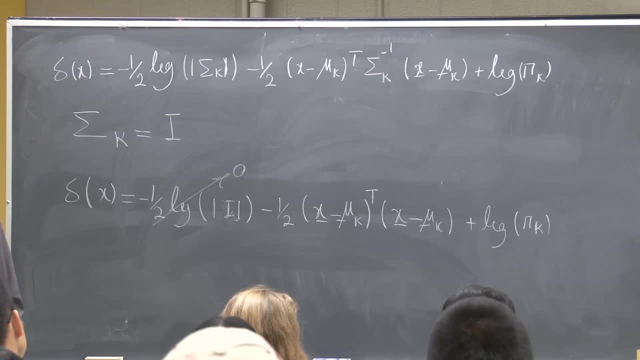 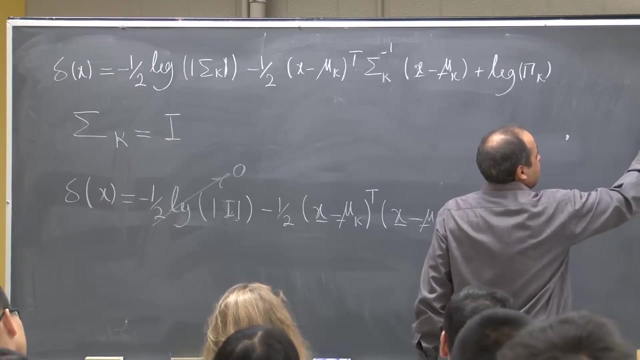 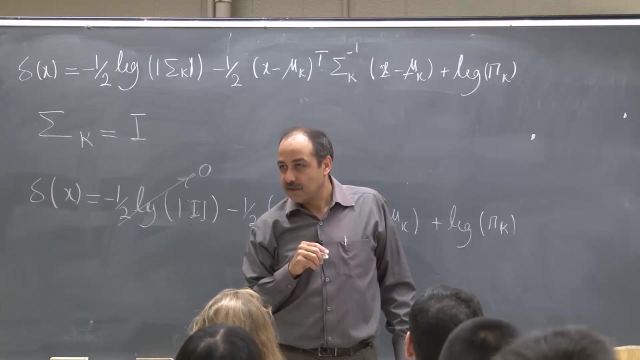 Okay, So X minus mu K times. transpose times: X minus mu K. What is it? Sorry, You know, X is a vector, a point, mu is another point. It's a squared Euclidean distance between these two points, right? 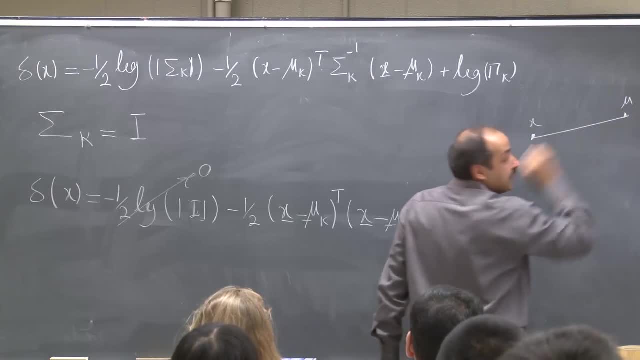 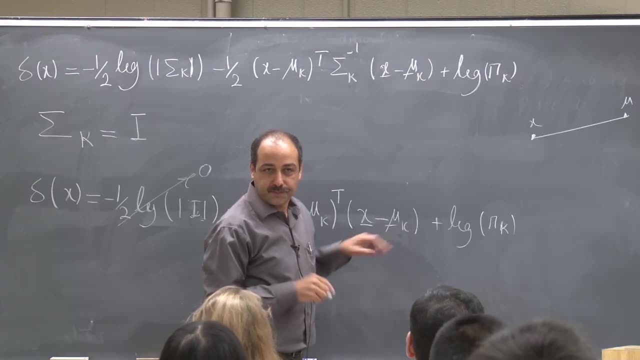 So X mu. so that's Euclidean distance between these two points. So X minus mu K. transpose X minus mu K, that's a squared Euclidean distance And this is a constant log pi K. So for simplicity, at the moment, assume that I'm talking about a case such that. 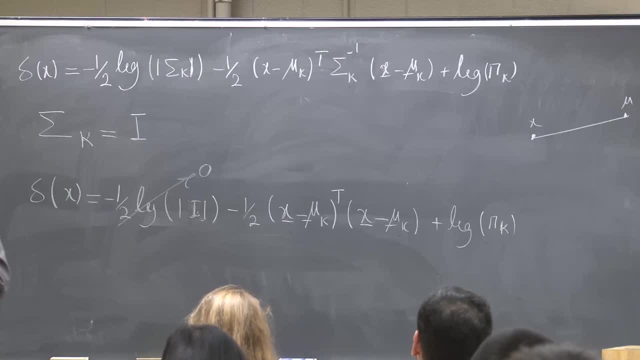 prior of each class is the same as the other one. So points equally has been distributed. So I have two classes, 100.50 here and 50 there. So pi 1 is the same as pi 2.. For the moment, assume that's the case. 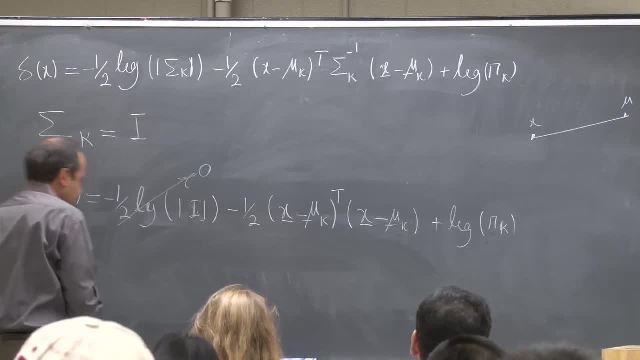 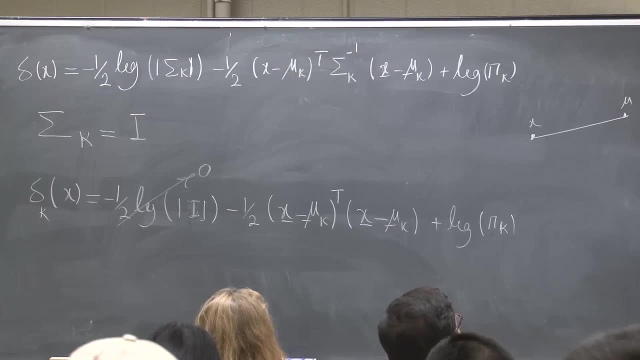 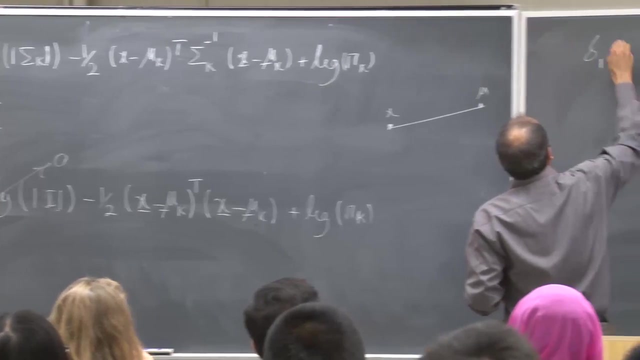 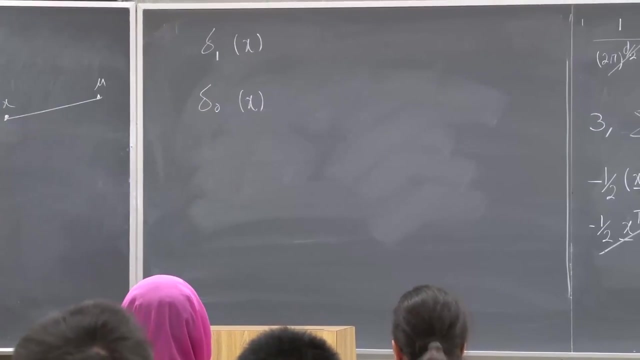 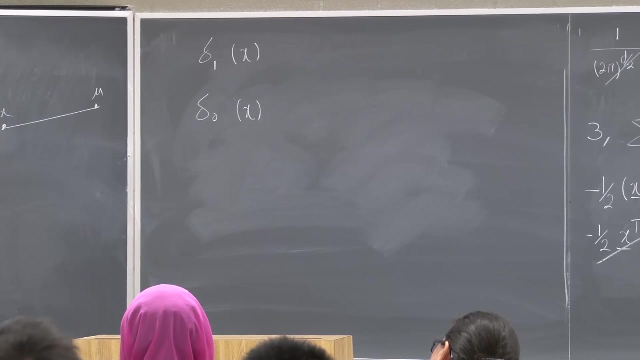 So when I compare- you know, suppose I have two classes- I have to compare delta 1 with delta 0, and delta 1 is Euclidean distance between point X and mean of class 1, and delta 0 is Euclidean distance between X and mean of the class 2. 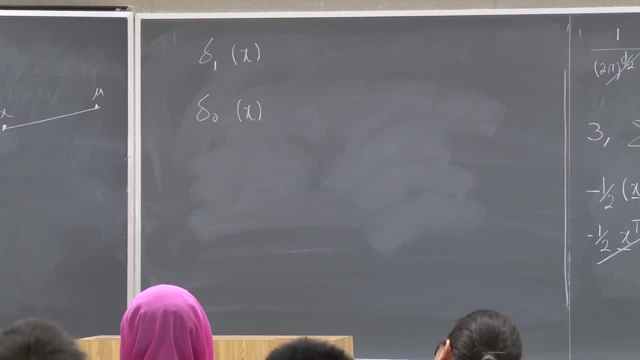 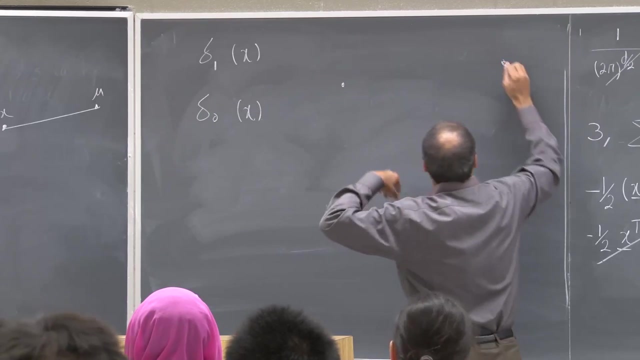 or class 0 plus a constant that, for the moment, I assume is the same for any class. so what does it mean? it means that LDA or QDA classifies points quite easily. you know I have two classes. I assume this is Gaussian. I assume this is Gaussian. 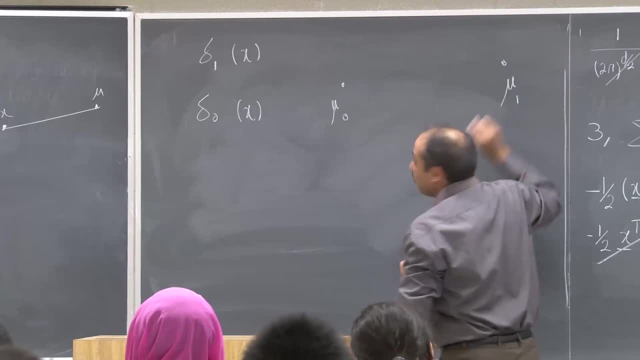 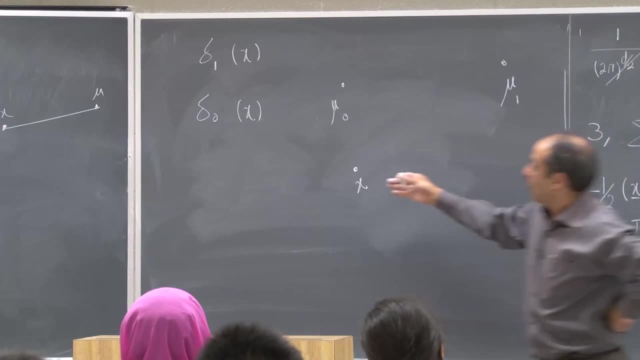 this is the mean of class 1 class, this is the mean of the other class and you give me a point to classify. this point belongs to this class or belongs to the other class? so in the very simplified scenario that sigma is identity. what we are doing 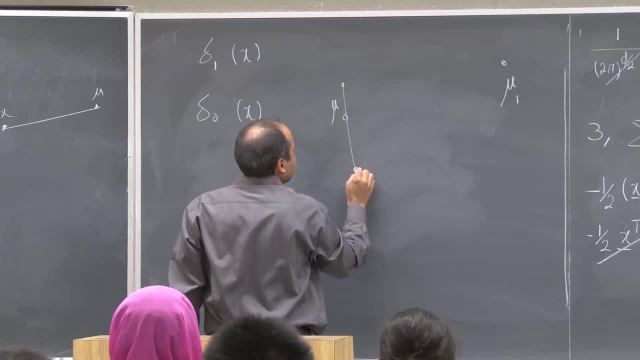 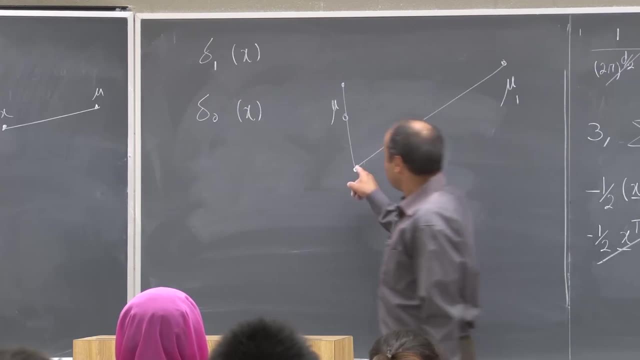 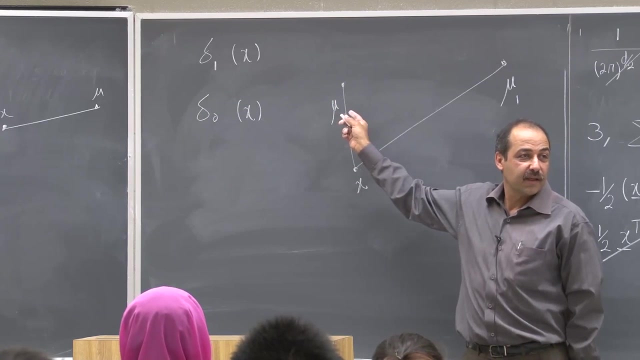 is just to look at the distance between the two classes, between this point and the mean of each of these classes, and decide that this point belongs to the class that has shorter mean, shorter distance. so you are closer to the mean of this class. okay, go here. you're closer to the mean of the other class. 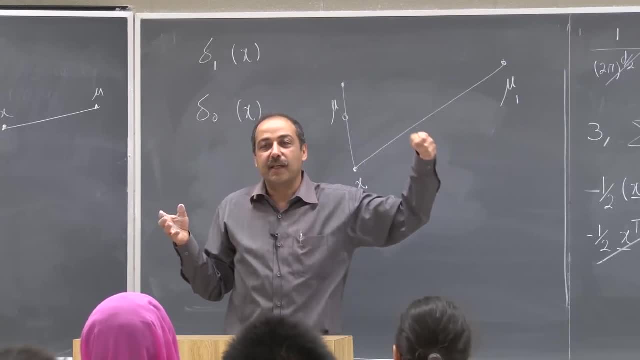 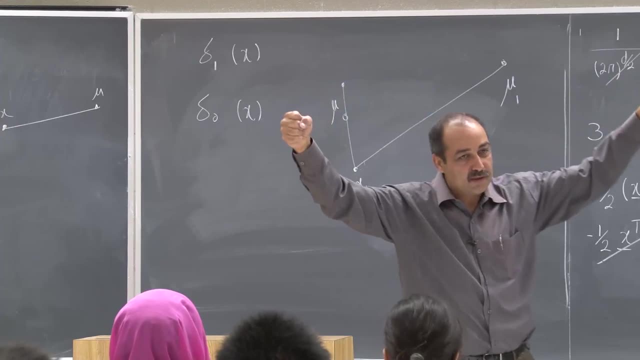 so basically, it's intuitively. you know I have twos and threes. I take the average of twos, I take the average of threes. two is look like this on average trees looks like this. so it give me a new digit: is it two or three? I just compare: is it closer to this mean or it's closer? 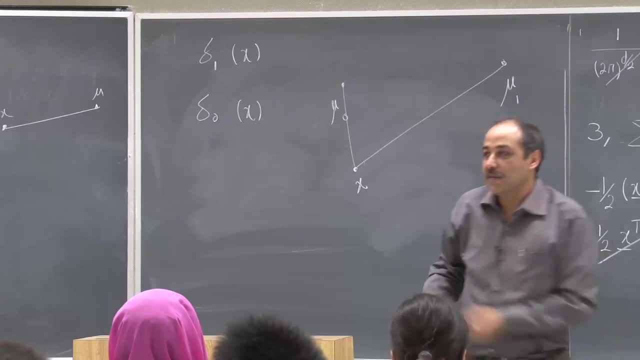 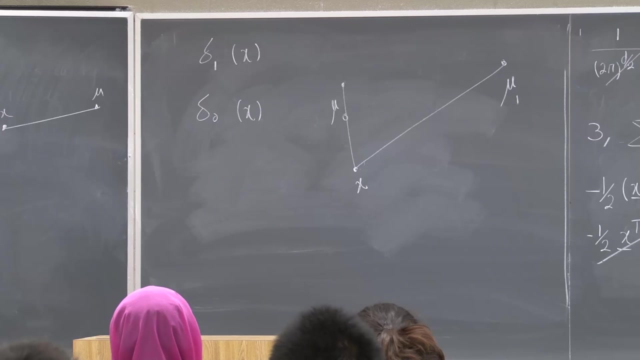 to the other means closer to this one. okay, go for this label, it's two, or the other way around, with this assumption that Sigma is I means Gaussian is spherical. okay, next lecture we're gonna see that, in this more general case, that Sigma is not as recall, and this is not the same, intuitively, what's happening in. QDA and LD.